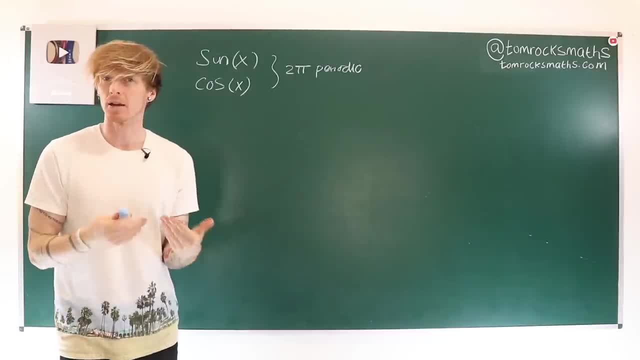 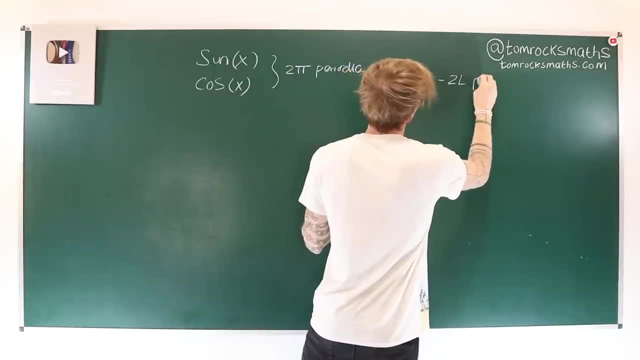 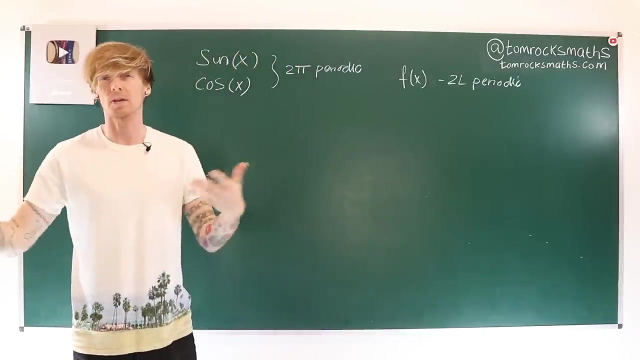 our function f is 2 l periodic. So we have a function f of x which is going to be 2 l periodic. So this means it repeats every 2 l as you move along the x-axis, much like sine and cos repeat every 2 pi. 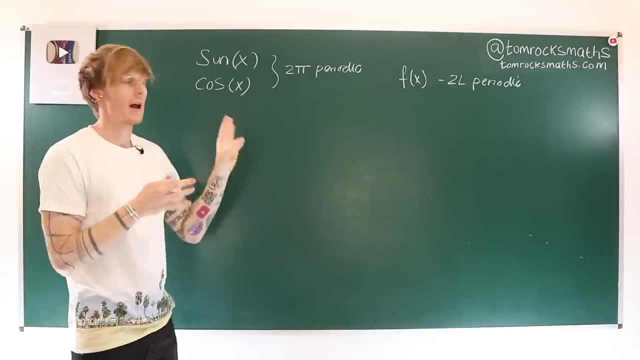 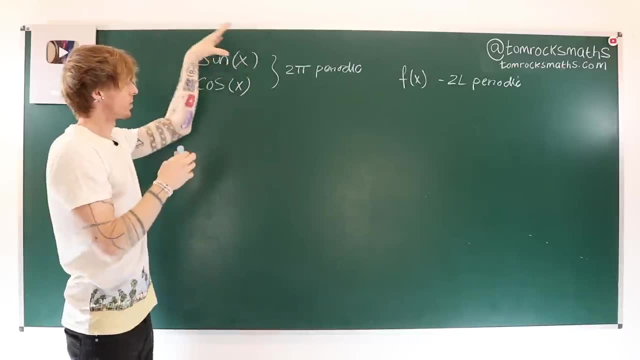 Now, because we want to construct our function f using an infinite series of sine and cos, we actually want to consider a certain form of sine and cos which are going to be theï, which are going to be the proper bakery model function. So what we 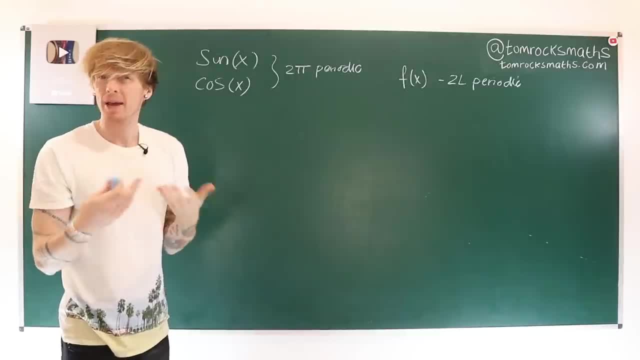 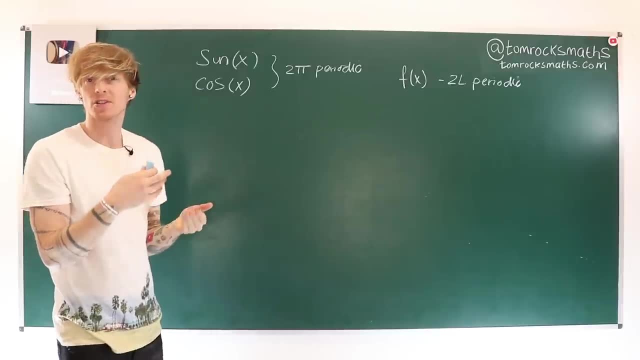 moonsatherine. we want to just twice over. disconnectedierno are going to be 2L periodic also. So in fact, what we're going to look at here is rather than just sine of nx or cos of nx for some integer, and then we sum them. 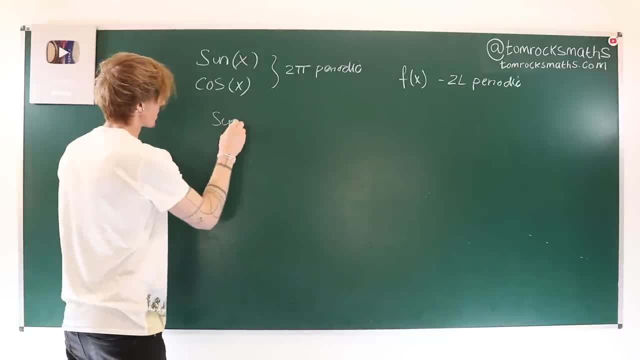 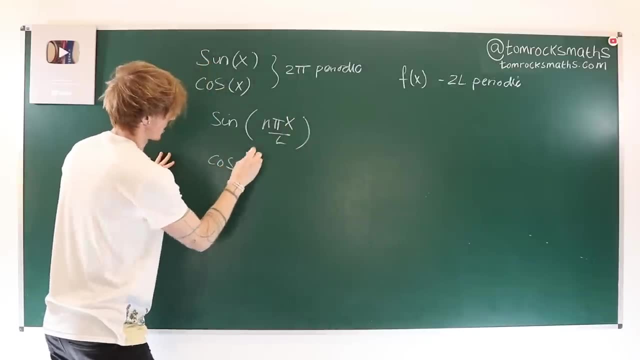 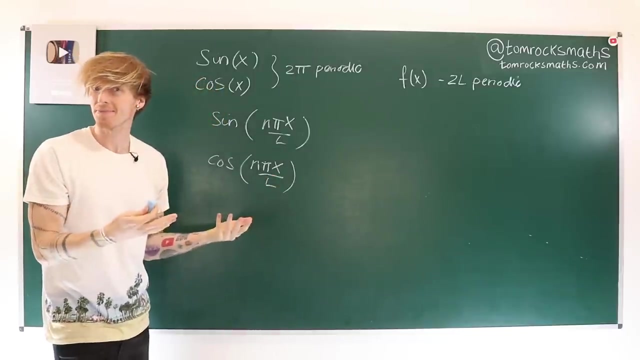 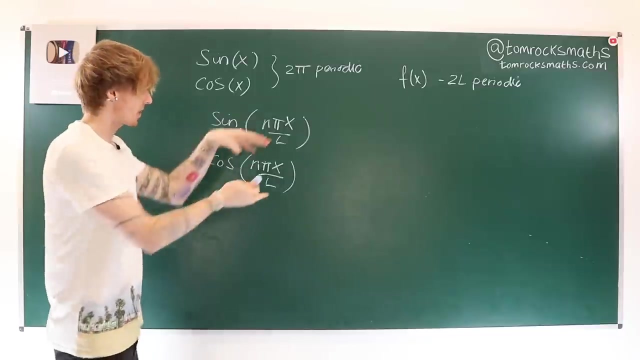 What we're going to do instead is to consider sine of n- pi x divided by L and cosine of n- pi x divided by L, Because for each value of n and again, we're going to add together all of these as n increases from 0 to infinity for each. 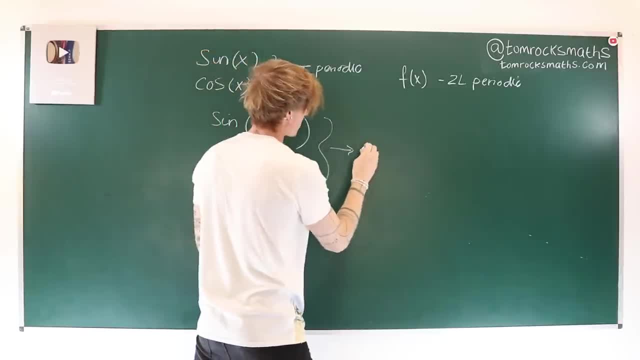 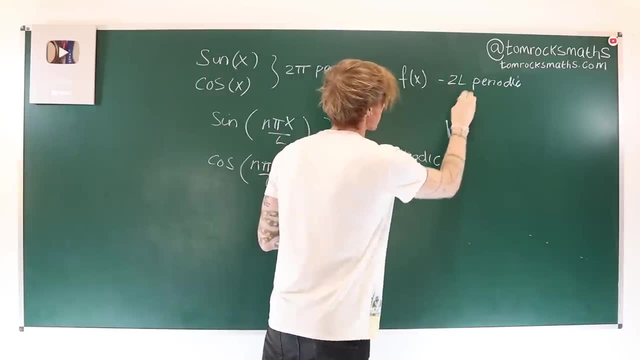 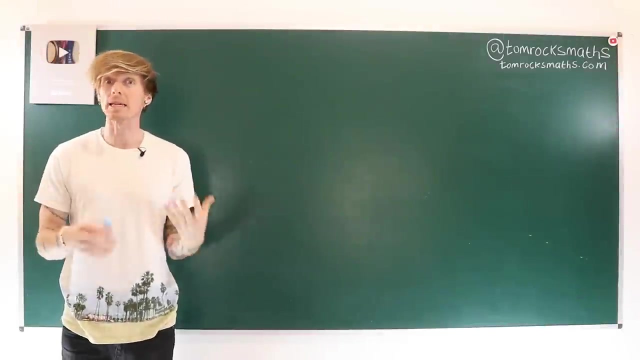 value of n. these functions are now 2L periodic, and so they match with our function f, which is a general periodic function. the second property that we need to construct our Fourier series is going to be the orthogonality of both cos and sine. I'm going to show you an 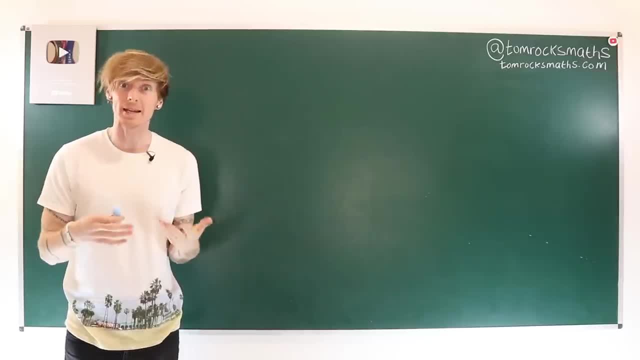 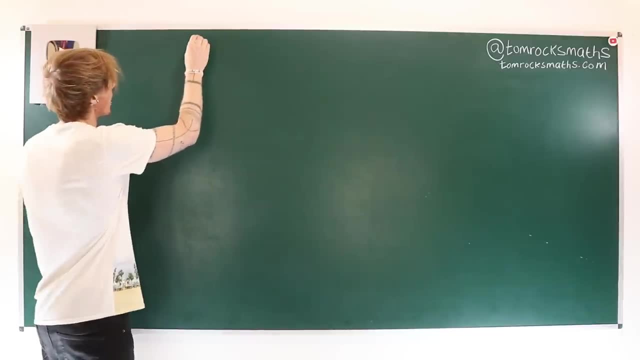 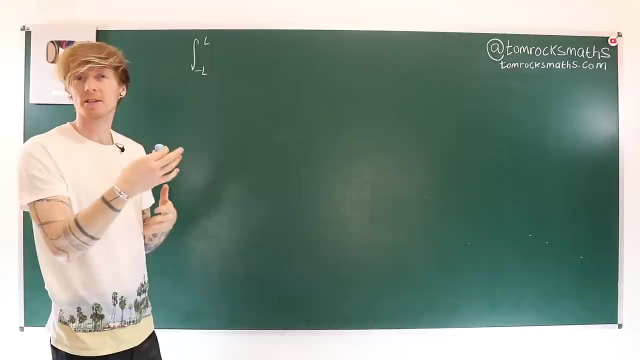 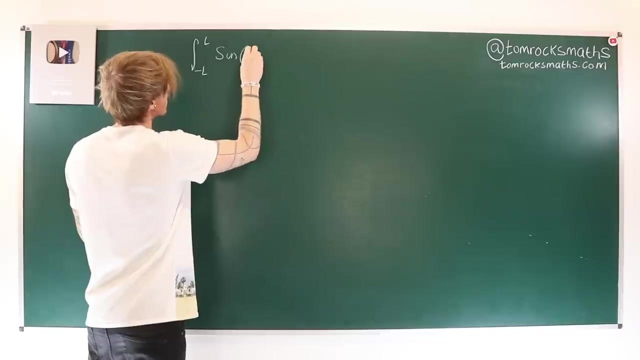 example, to demonstrate exactly what we mean by the word orthogonality. So suppose I want to do the following integral To integrate from minus L to L. you'll notice this has length two-eighths l, which is going to be the period of our function, and I want to integrate sine of. let's suppose we 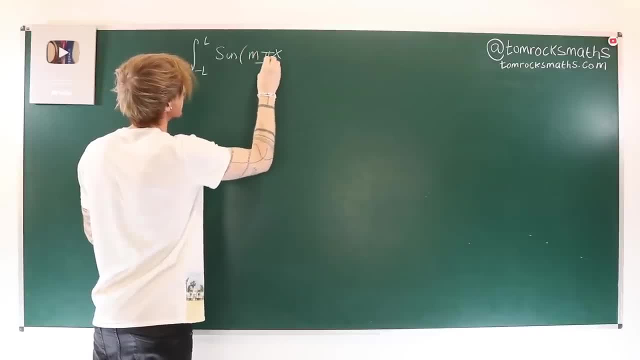 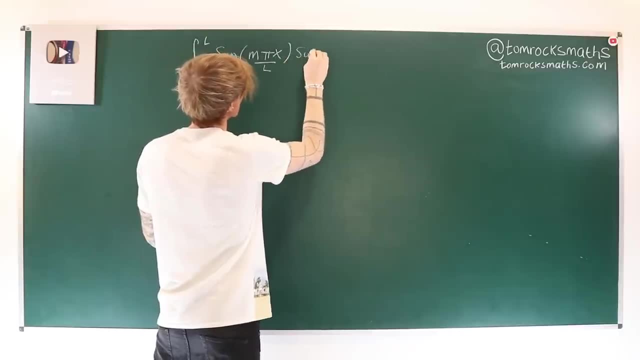 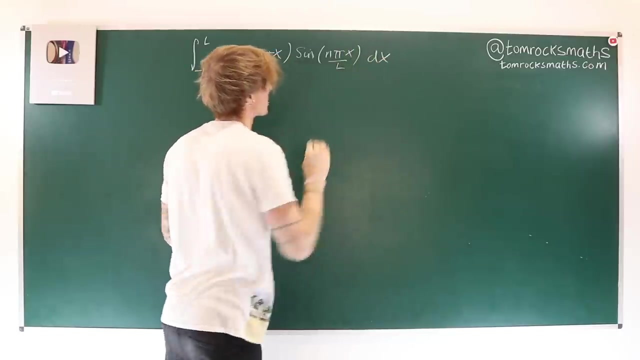 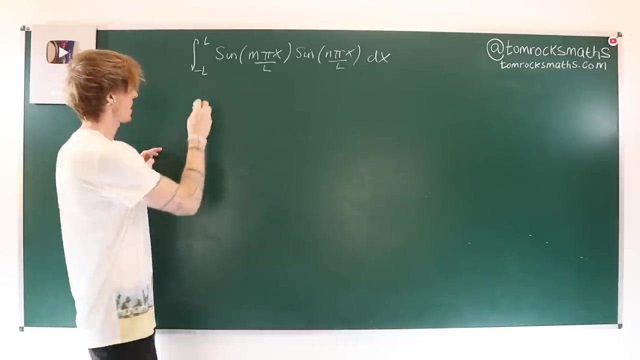 have m pi x divided by l, so that function again is 2l periodic multiplied by sine of n pi x divided by l. and we're integrating with respect to x Using the appropriate product to sum formula. this tells us that the integral becomes minus l to l, there's going to be a factor of a half. 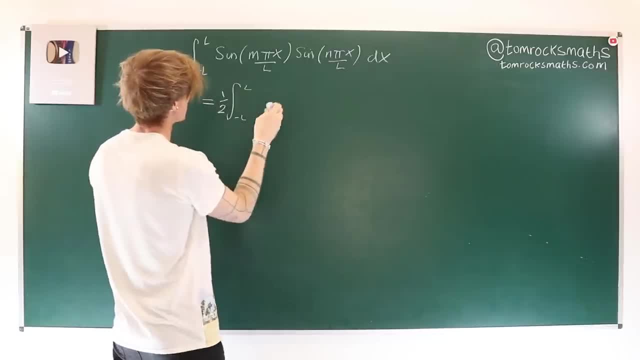 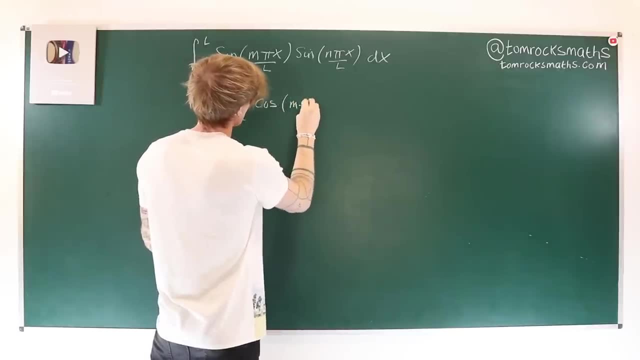 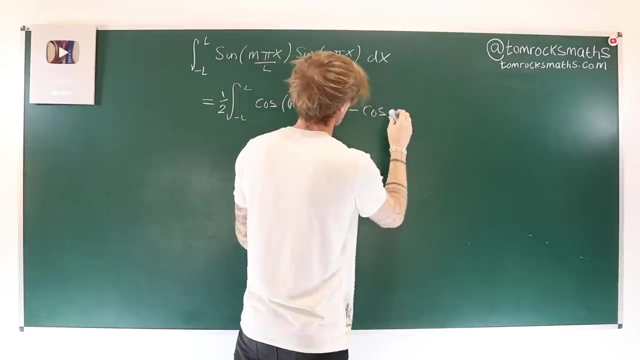 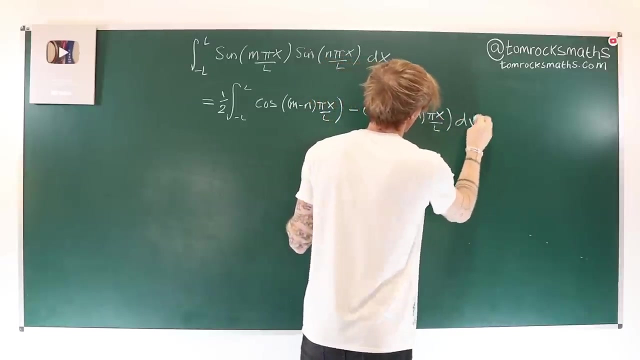 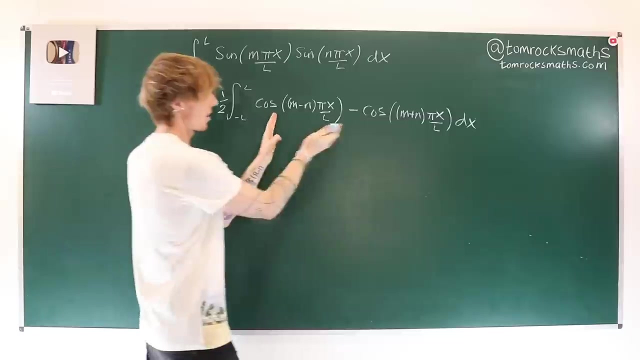 which I'm going to put outside of the integral, and then inside we have, I believe, a cos of m minus n pi x over l, and then we subtract cos of the sum m plus n pi x over l. If you're unfamiliar with the product to sum formula, if you start from the second line here, 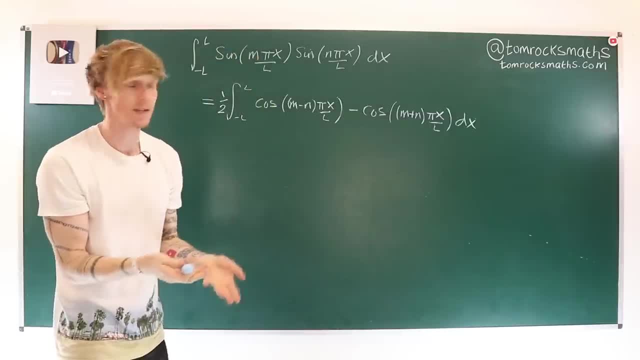 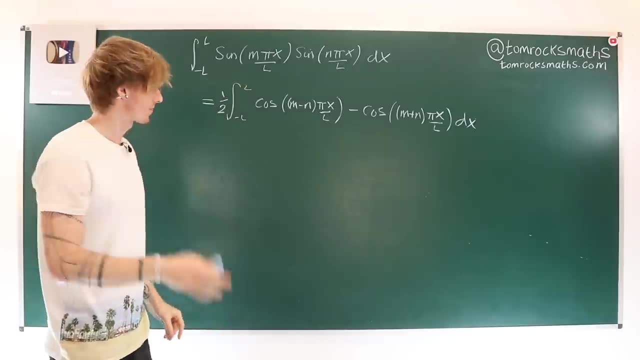 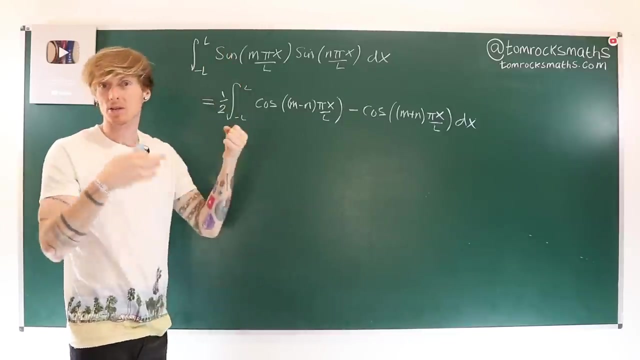 and use these standard trigonometric addition formulas, you will see that the various terms you get cancel out and you're left with exactly what we have at the top. So this is now an integral that we can do. This is the advantage of turning the product into a sum. We have two pieces we can integrate. 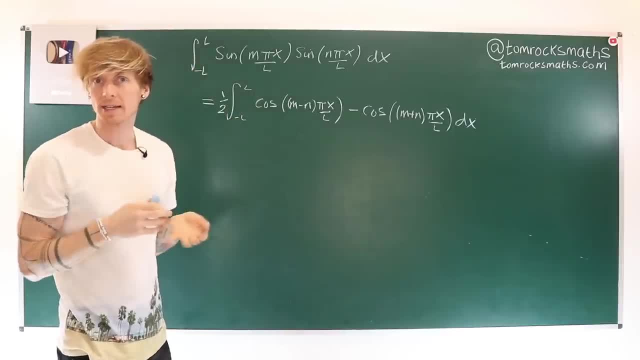 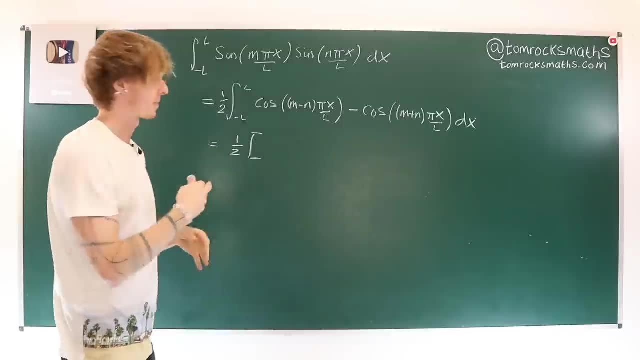 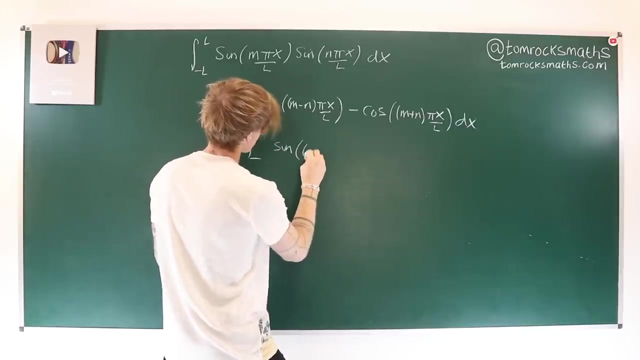 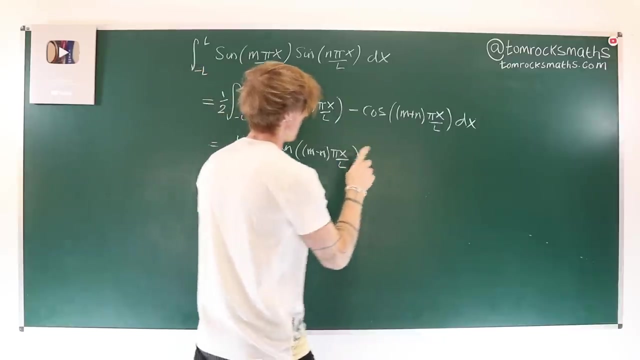 cos of something and use the reverse chain rule to get the answer. So we can do that and say: this is a half times the integrated part. So that's going to be a sine of m minus n, pi, x over L. That's not changed. And then we've also reverse. 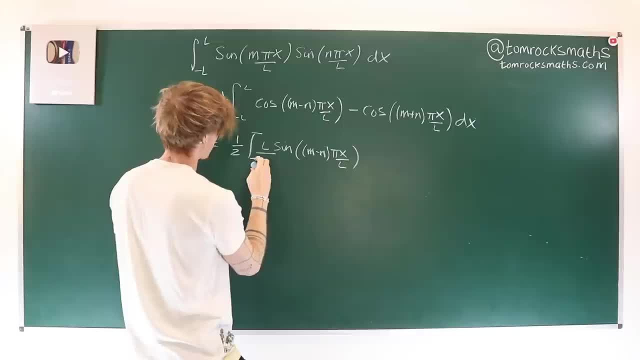 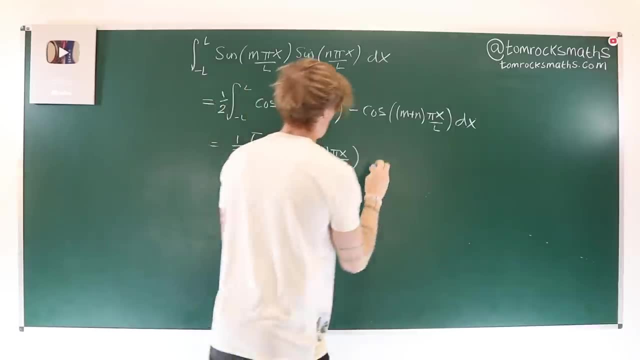 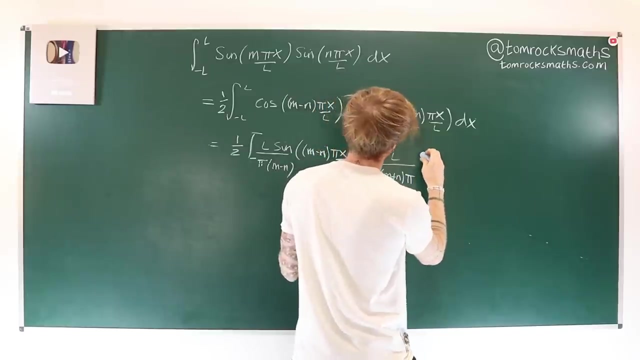 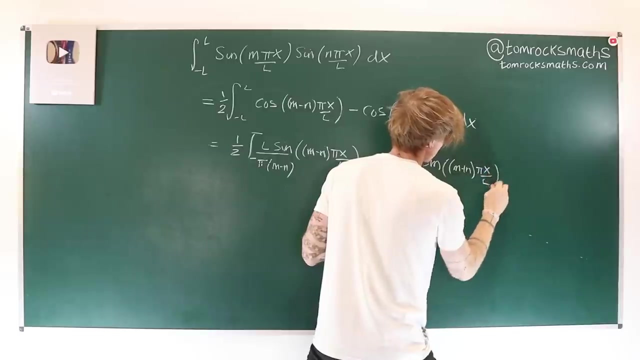 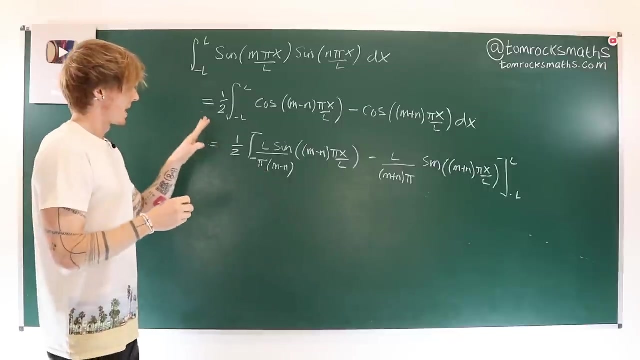 chain rule, given us an L divided by pi times m minus n on the bottom there, And then we subtract off and again we're going to get an L over m plus n times pi, and that's also come from a sine, Okay, so I think that's correct so far. Now there, 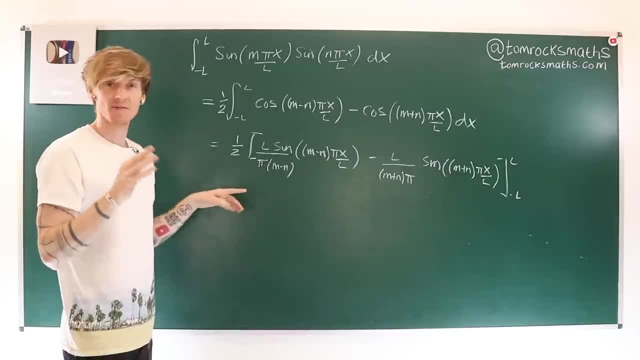 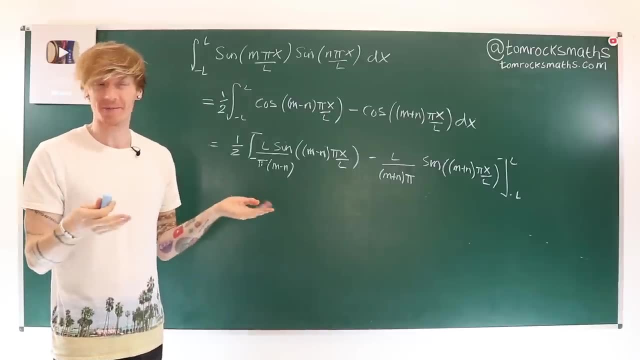 are two things that can happen here, and this is a very important technique or thing to always check whenever you're doing any maths problem, not just this one. This could be a very important thing to always check whenever you're doing any maths problem, not just this one. This could 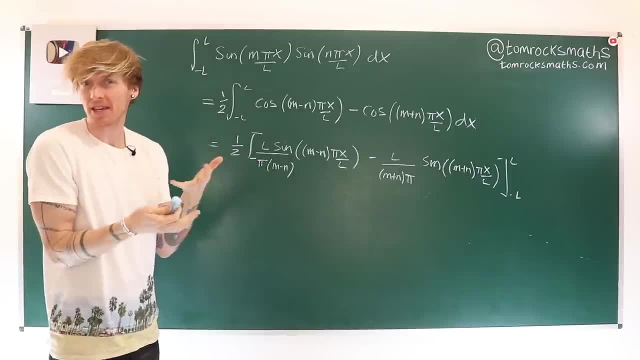 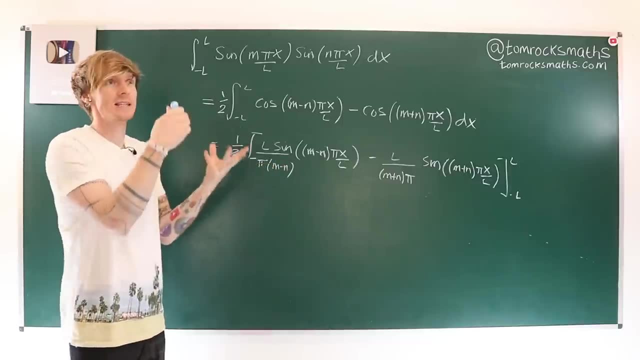 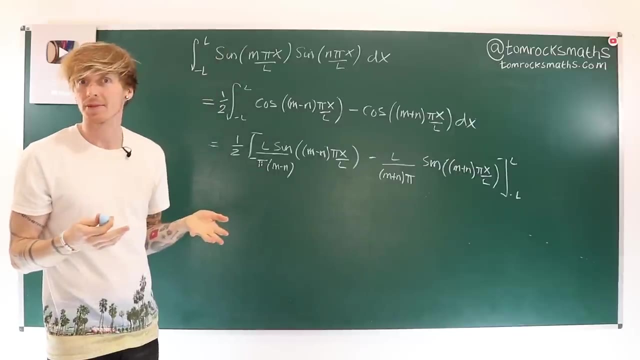 be zero. There's, at this point, there's nothing telling us that m and n are different. We know they're both positive integers because, remember, we're interested in adding together this infinite sum from n equals nought to infinity of all of these different sine and cosine terms. So we can certainly 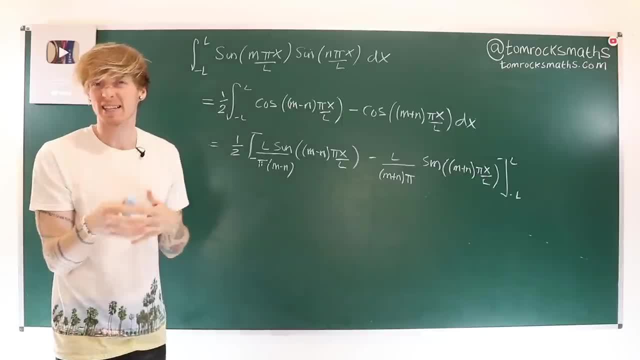 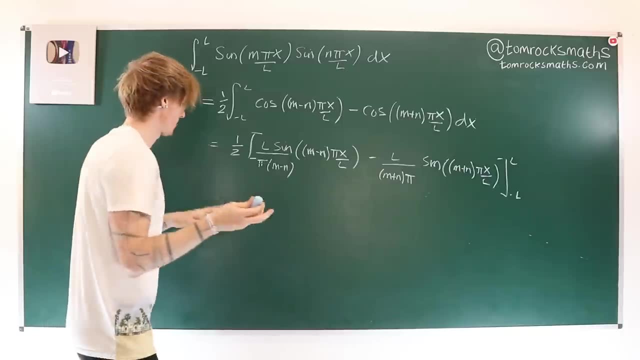 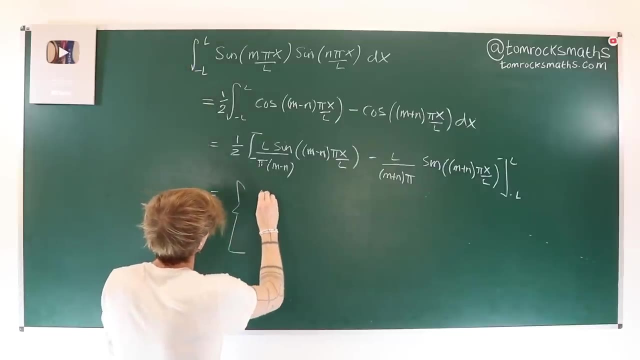 assume they're positive, without loss of generality. let's say, m is bigger than n, But they could be equal. that's the key thing. So we're going to do that. We're going to split this up into two cases. So we've got one case when m is. 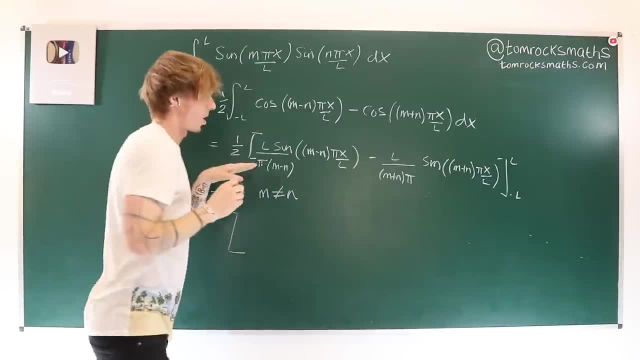 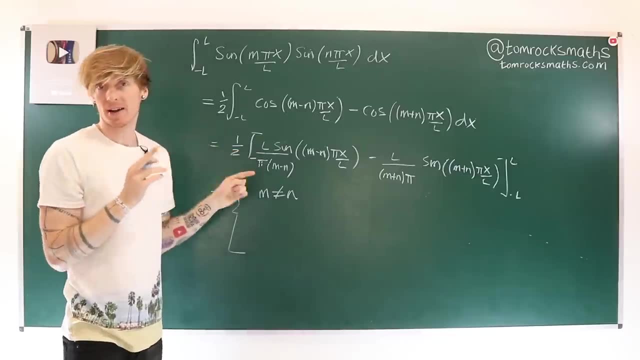 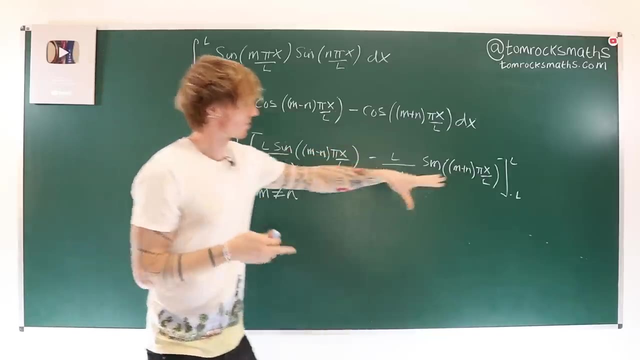 not equal to n, which is the one that I've written out here. So provided m is not equal to n, I am NOT dividing by zero and therefore I can evaluate this expression. So when I do that, I could of course explicitly substitute in the L. 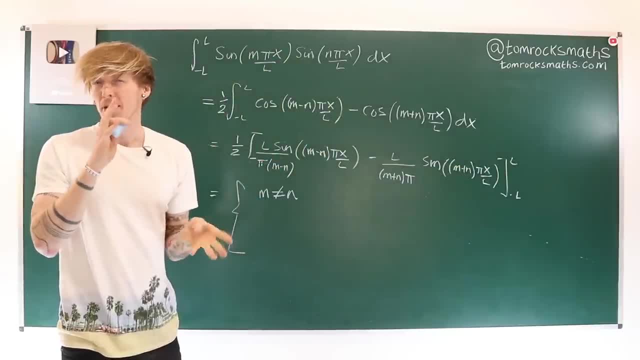 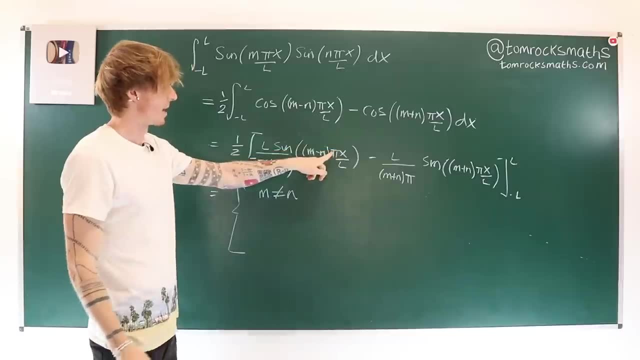 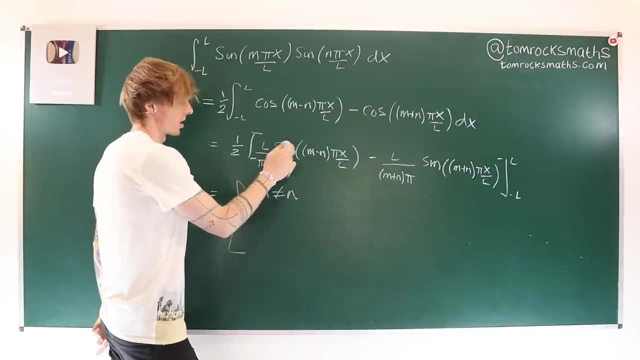 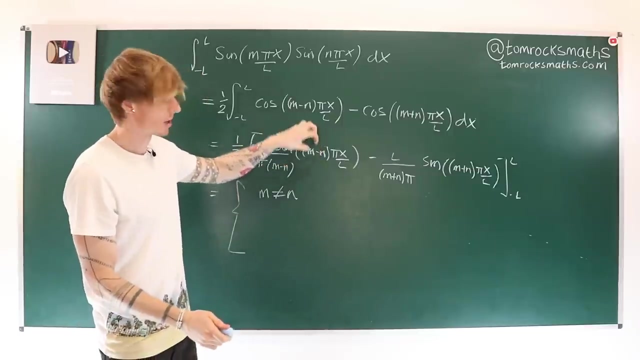 terms and add together those four pieces. But you can spot what's going to happen, because when I substitute in L, this becomes pi, L over L, So the L's cancel and I'm left with a sine function of an integer multiple of pi, It's sine of some integer times pi. If you think about the. 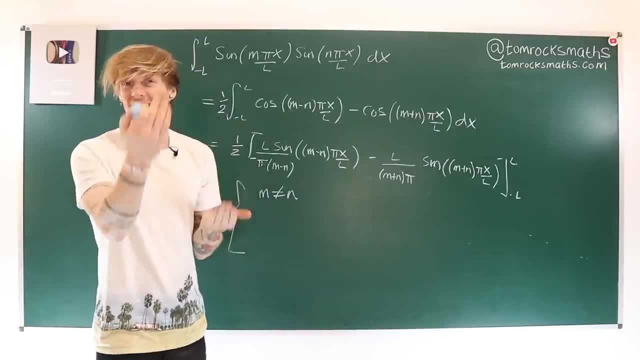 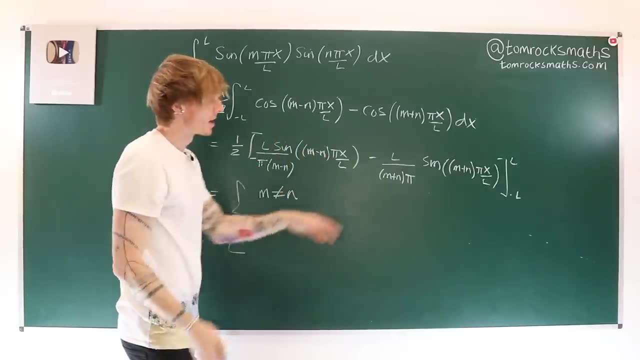 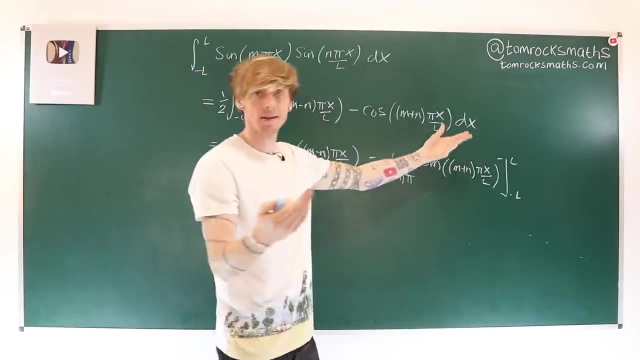 graph of sine. it is zero at every integer multiple. So this will be zero when x is L. Similarly, this is sine of an integer multiple of pi. L over L gives me one again, So this is another sine of an integer multiple of pi. so that's. 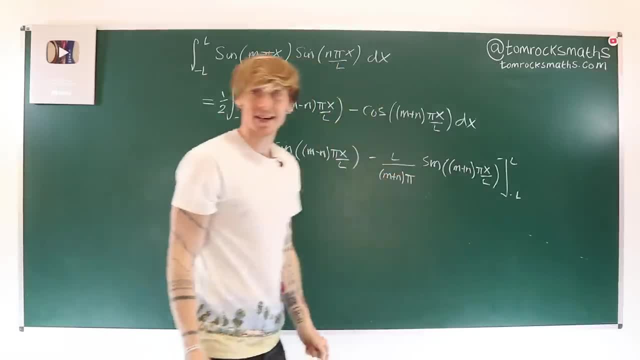 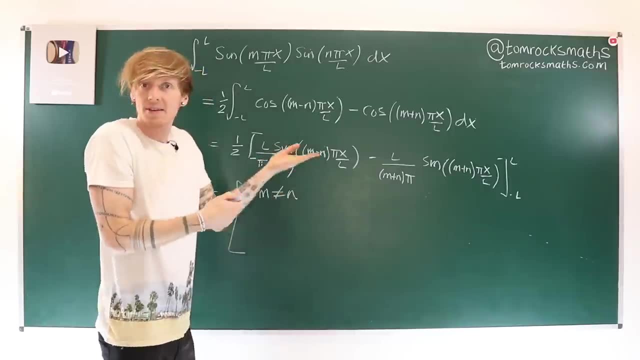 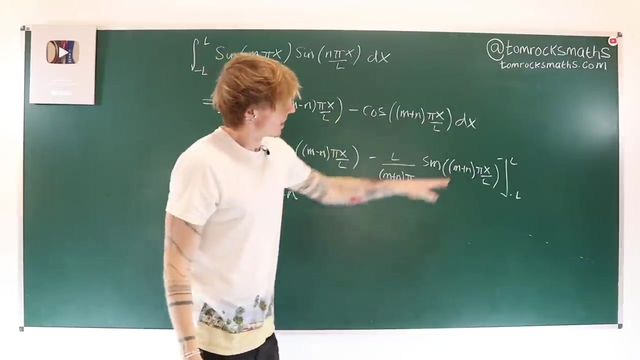 also zero Minus L. the exact same thing is going to happen. We substitute in here we get sine of negative integer times pi- It's still zero, Minus sine of negative integer times pi- It's still zero. So all. 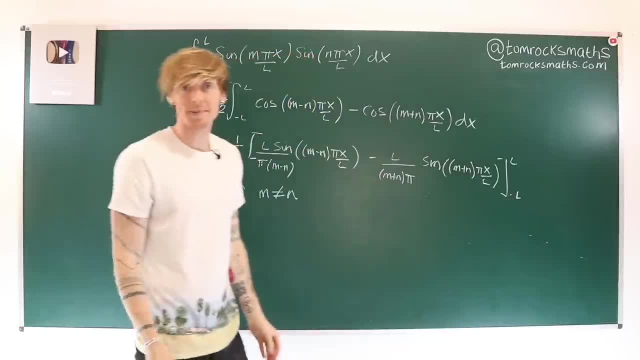 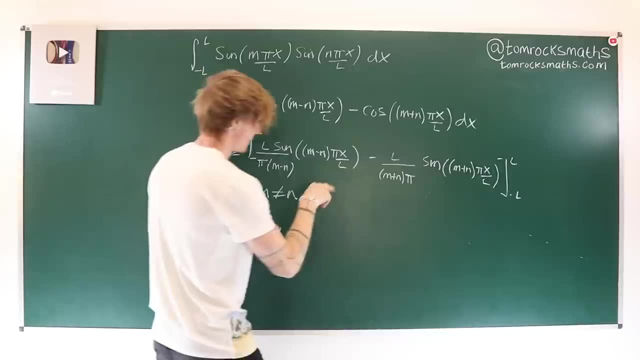 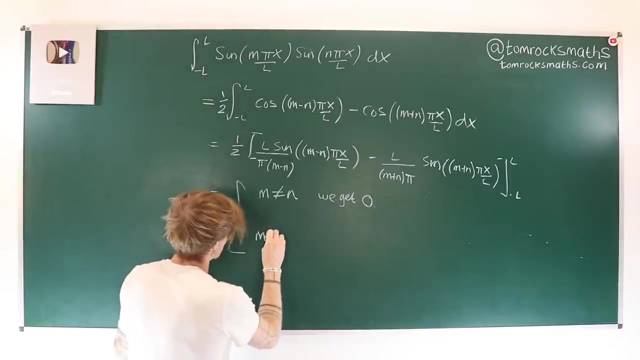 four individual terms, plugging in two from each limit, they're all zero. So, provided this is valid in the first place, provided this is valid, the answer here is just zero. So we get zero. Now the interesting case is exactly when m does equal n. So for this one I'm going to take a different. 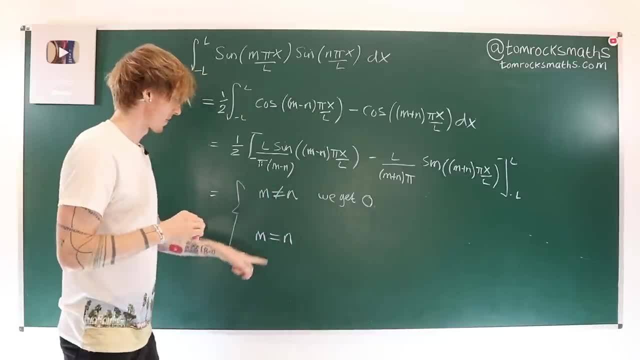 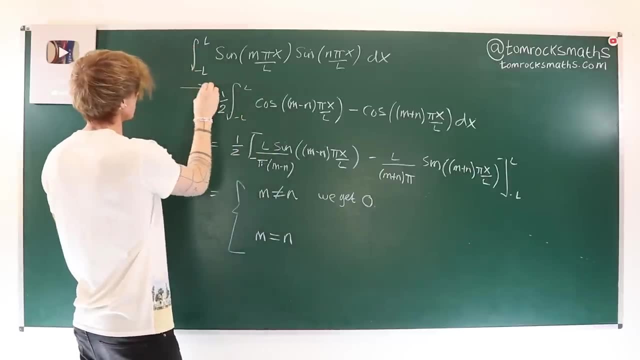 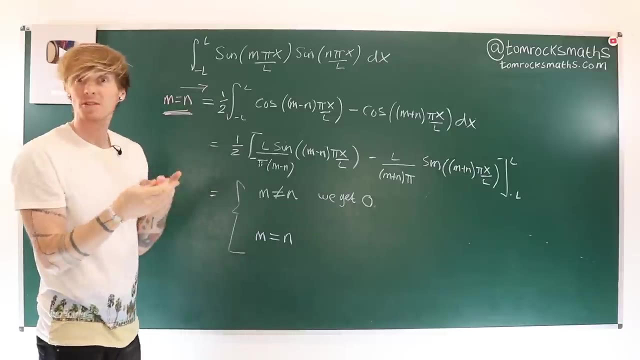 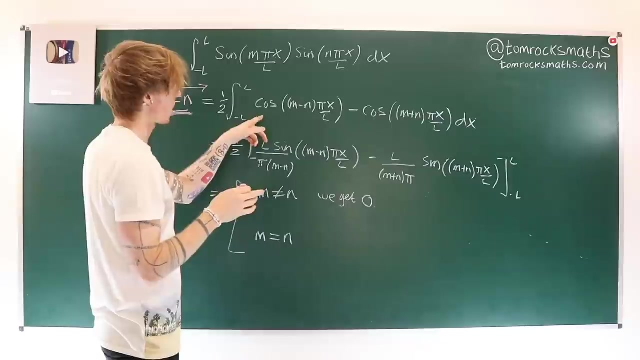 colored chalk so we can see this more clearly. So when m is equal to n, we go back to this stage here and say: m is now equal to n. So what does this mean? Well, this m equal to n, that gives me zero now. So this is cos of zero, doesn't matter, what's. 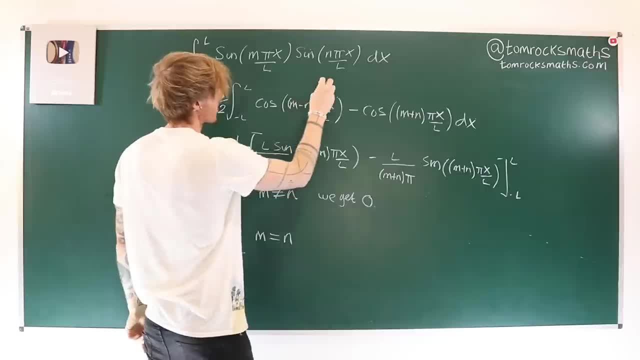 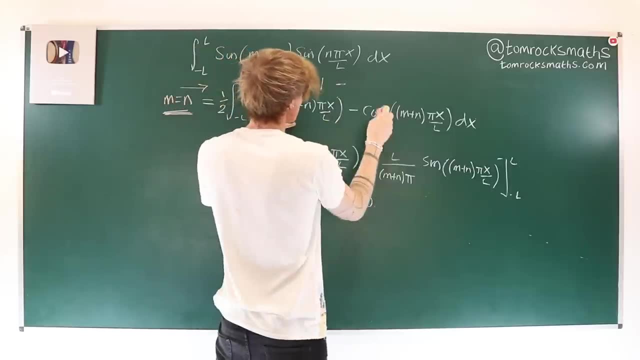 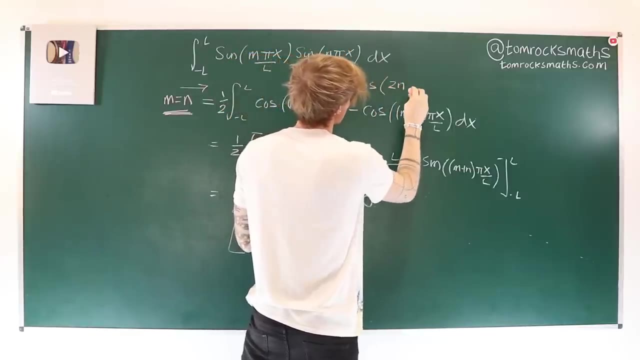 here this is cos of zero, so we know that becomes a one, So this now becomes one. And then here m and n are again. they're the same thing. So we've got a one minus cos, and what we're going to get inside that bracket will be two n pi x over L. 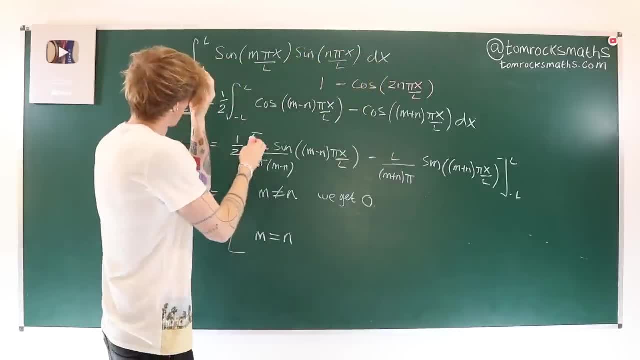 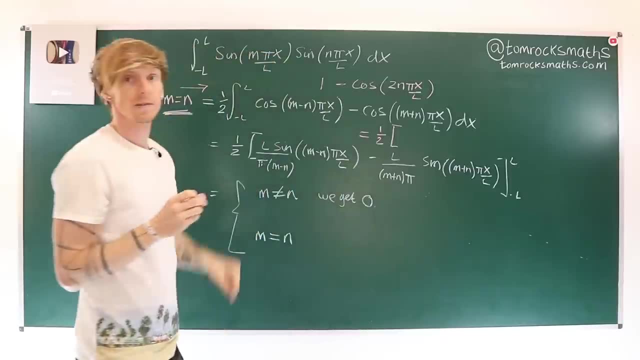 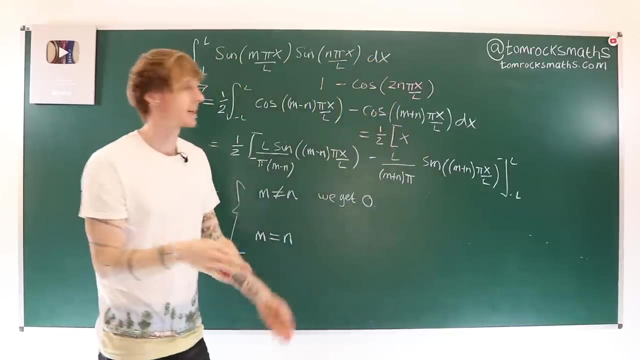 Okay, so proceeding from here and integrating Again, we're going to get the factor of a half outside the term in one that integrates to give me an x. Then the cos term again comes from the sine term. so that's now minus this thing's. 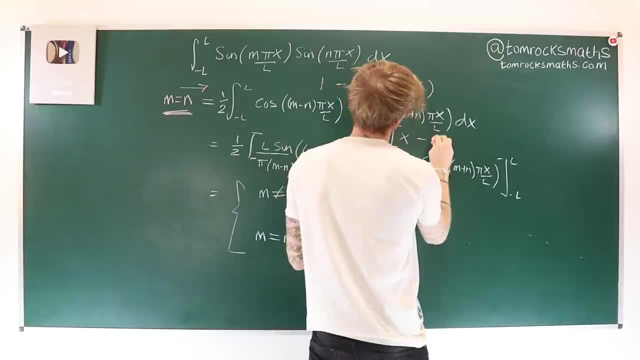 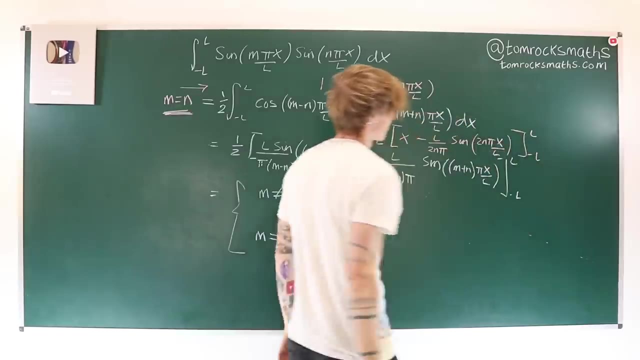 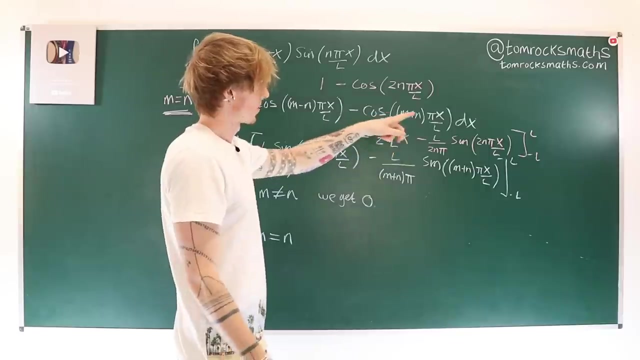 still valid. so I will get L over 2 n pi. And then we're left with sine. so that's sine of 2n pi, x over l, and that's p minus l and l Plugging in the limits, just as before. we're going to get a half of x, which is l, so we get there. 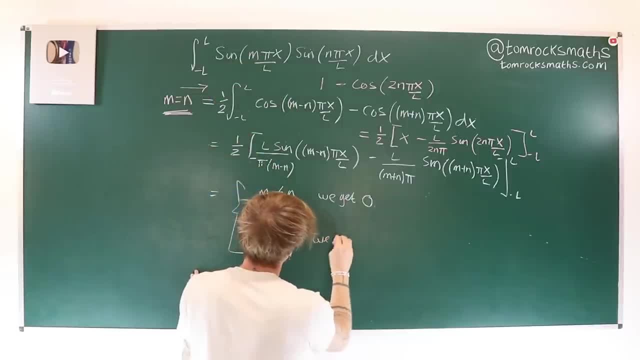 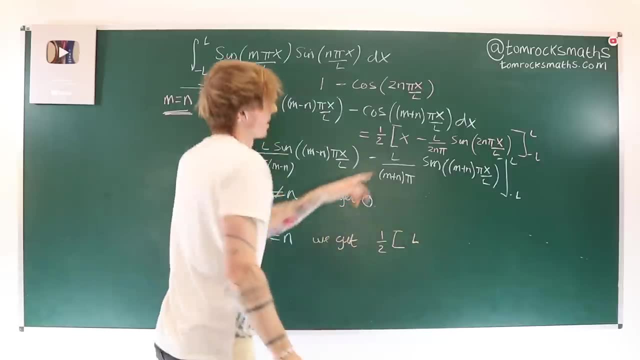 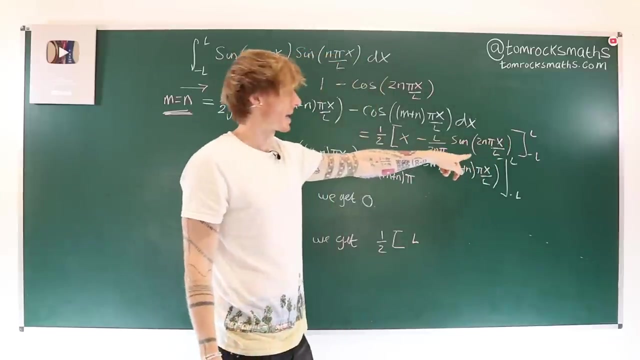 writing it down here, we get a half, and then I'm going to get an l minus l over 2n pi. times sine of 2n pi, l over l is 1, it's an even integer multiple of pi, still zero again. 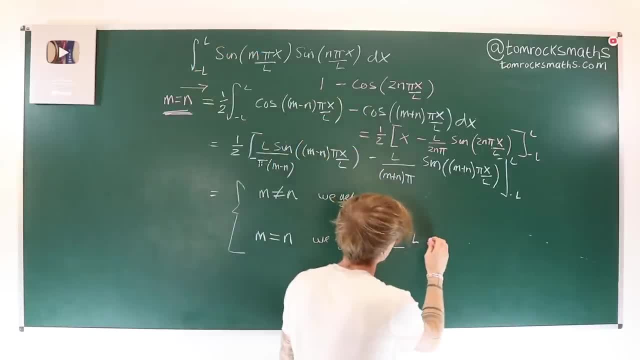 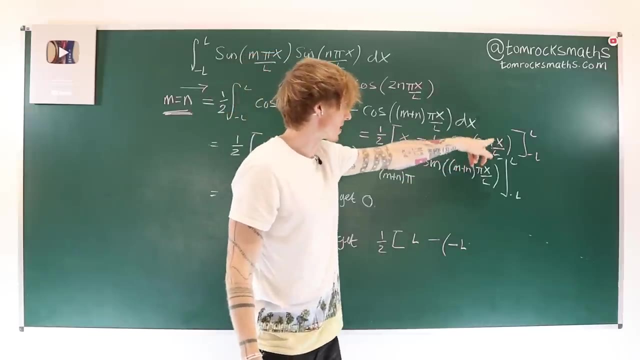 So nothing from that. and then we get minus bracket. it when we plug in x equals minus l, so it's minus minus l. and again, when we plug in minus l it gives us a minus one. in here we get minus an even integer multiple of sine. it's also zero. 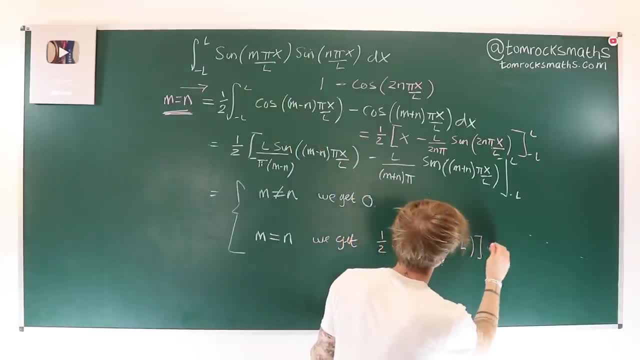 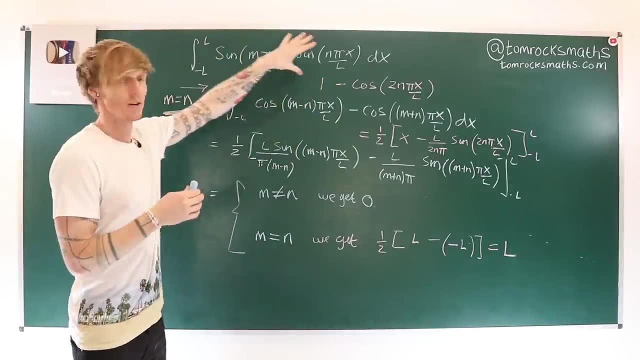 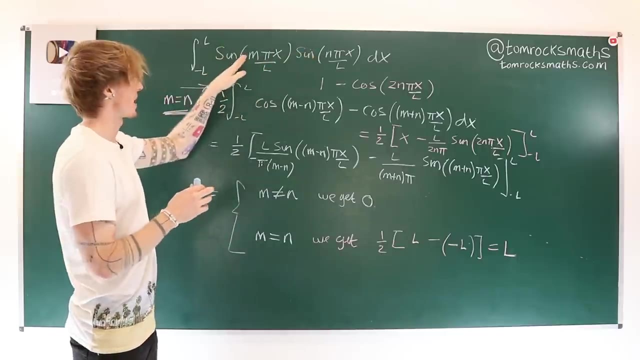 so it's minus minus l brackets. so factoring all of those things out, we get l. So what we've seen is when we have a product of two sine terms- and we will do the same for cos in a moment when we have a product of two signs, with an m and an n. we've seen that. 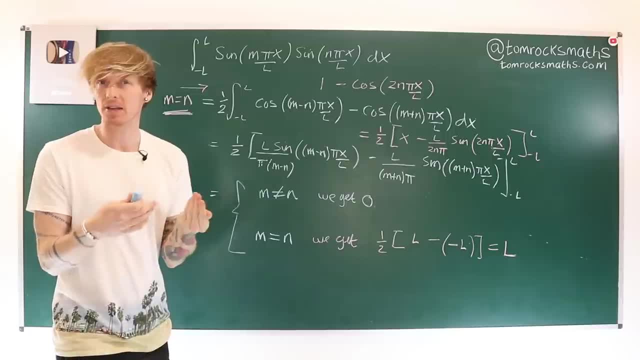 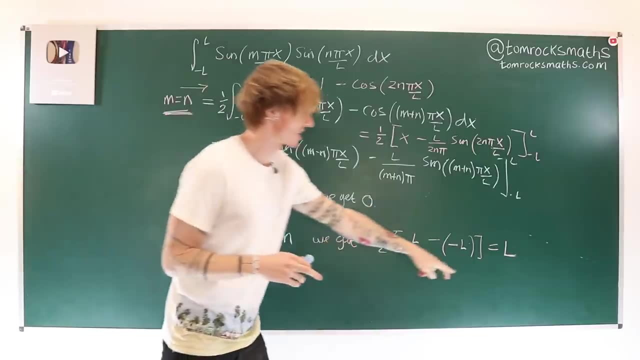 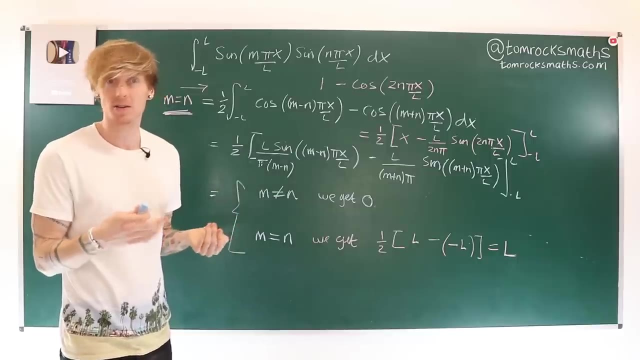 if they are different values, they are integer values, but if they are different, we've seen that the answer is zero, and if they're equal, then we actually get exactly l. So what we can do, or a nice shorthand notation that we can use, is to say that this integral. 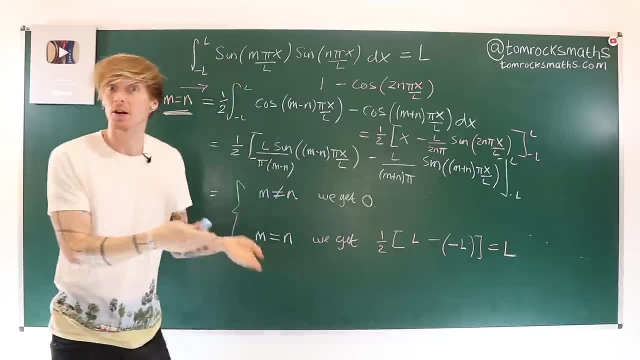 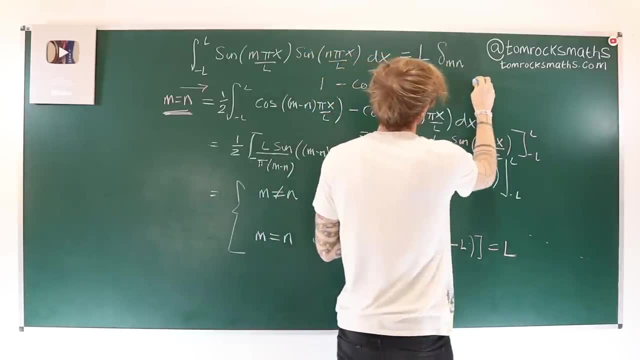 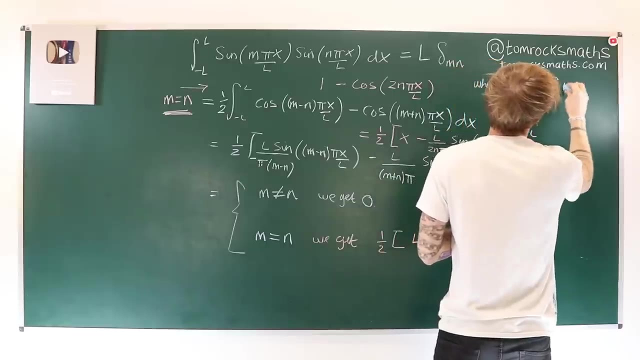 is equal to l, Which is the answer we got when they were equal multiplied by the delta function. So I'm going to write this as delta m n, and this is where delta m n takes the value 1, when m equals n and zero. otherwise, 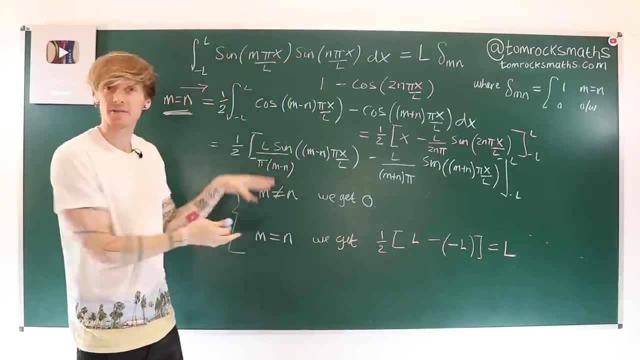 So it's just a shorthand way of expressing exactly what we found here in terms of the integers having to be equal in order to find the integral. So it's a shorthand way of expressing exactly what we found here in terms of the integers having to be equal in order to find the integral. 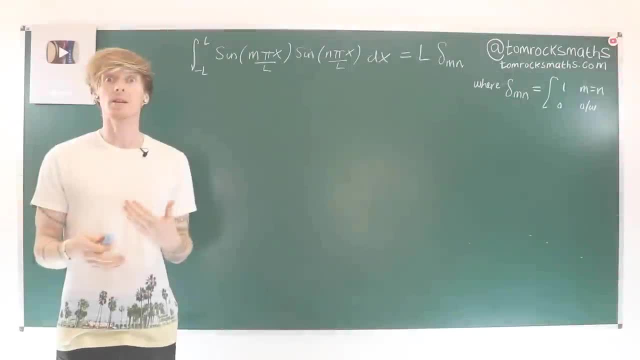 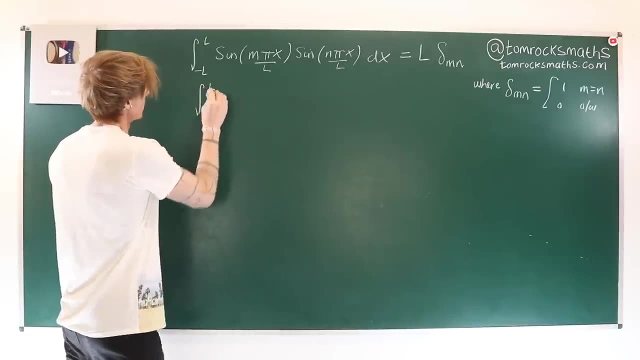 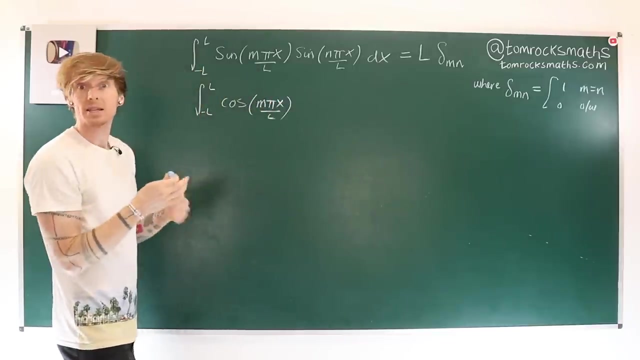 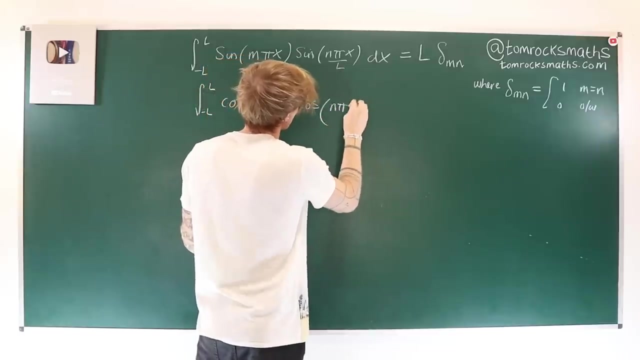 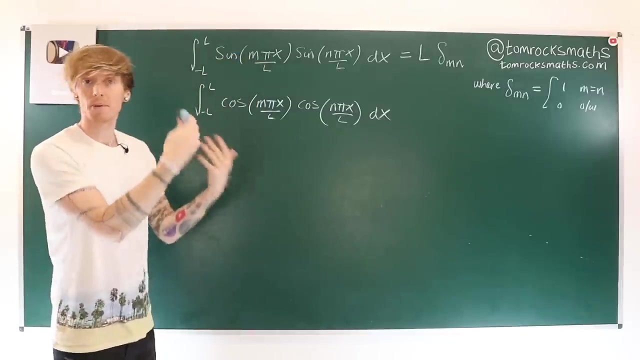 to get a non-zero answer. Now we can do the exact same thing with cosine. so we consider the integral from minus l to l of cos m, pi x over l, which, remember, is a 2l periodic function multiplied by cos of n, pi x over l dx. As before, we want to use the appropriate product to sum. 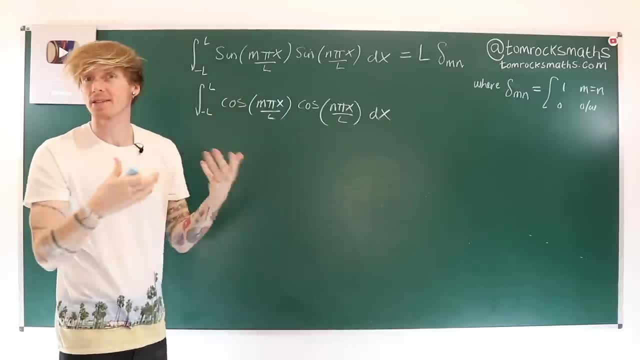 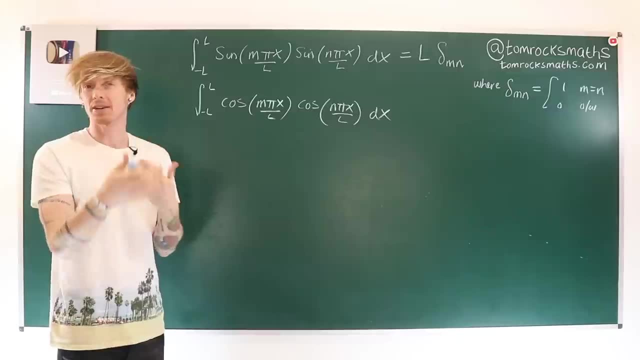 formula to turn our product of causes into a sum. We can then integrate those terms individually and, again as before, we're going to get a different answer depending on whether m is equal to n or not. Following through all of those steps- and I really do recommend trying this one for yourself- 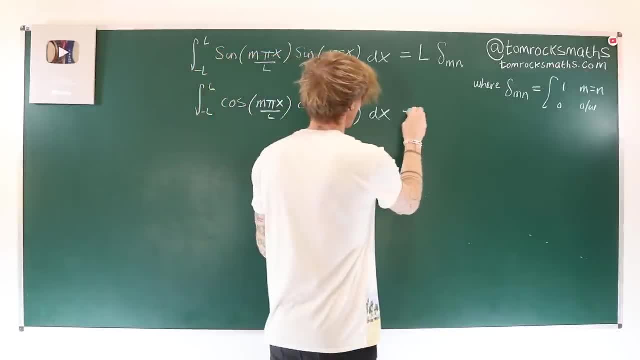 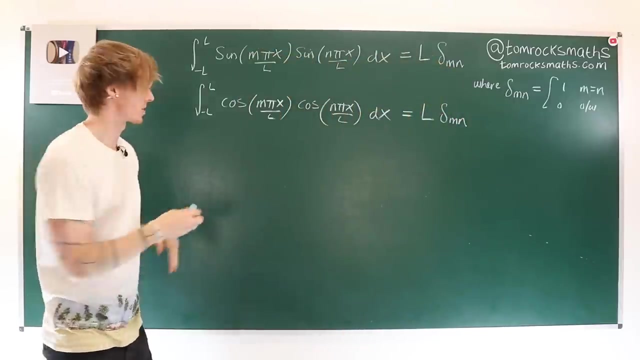 you'll actually get the exact same answer. So this is equal to l, half of the length of the period of our function, multiplied by again, delta mn. Now that just leaves a final combination, which is going to be the integral, from minus l to l, of sine. 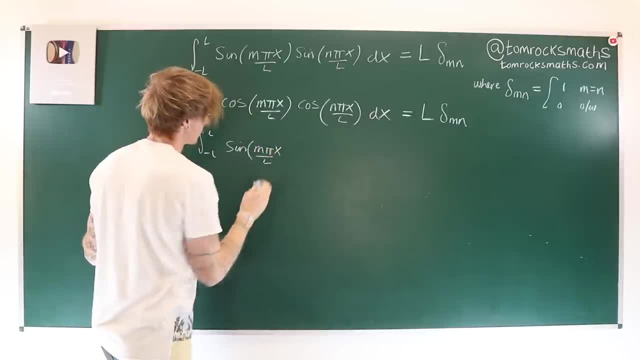 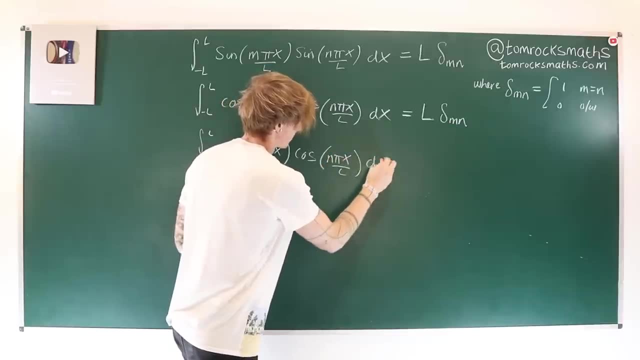 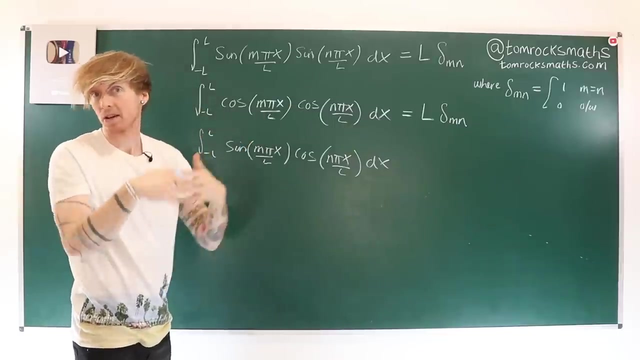 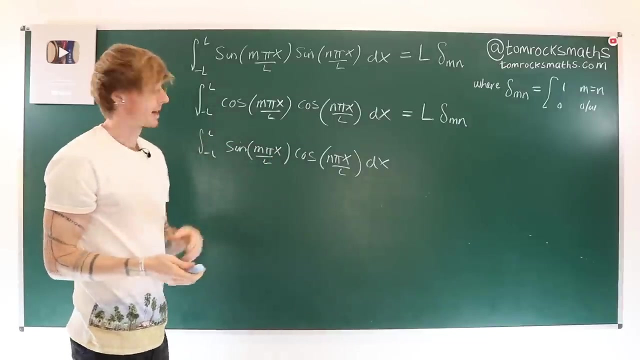 of m pi x over l times cos of n pi x over l. So for the first two we had two sine terms, two cos terms. so the only other possibility that could happen when dealing with cos and sine is we have a sine multiplying a cos. Now for this one we could proceed and use the product. 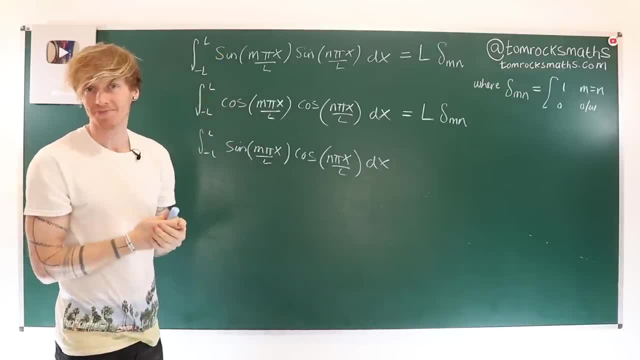 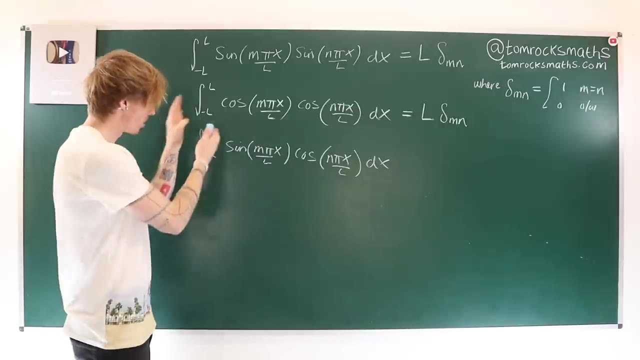 to sum formulae, just like we've done for the first two. However, we can be slightly cleverer and actually spot something about the function that we're integrating. So we know both of these are 2l, periodic and, importantly, we're integrating over a symmetric region. We're 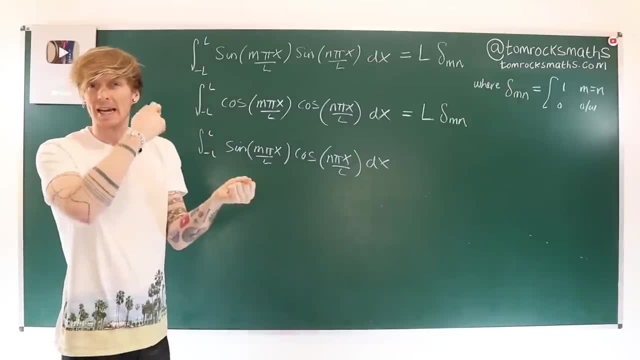 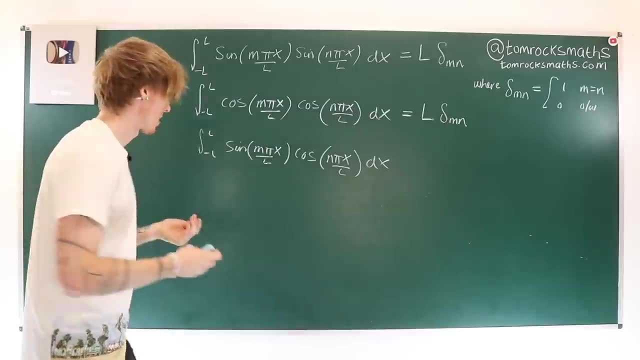 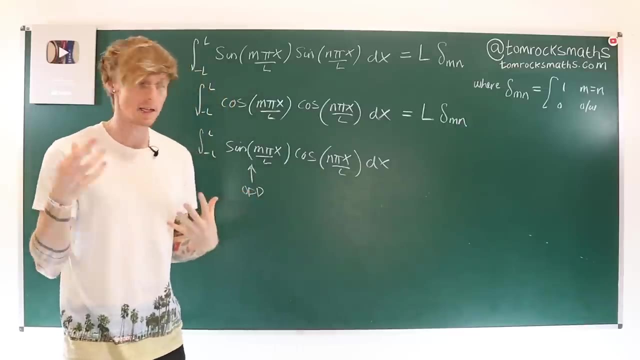 integrating from minus l to l, so we're integrating over a region which is symmetric about zero. Now sine is what we call an odd function. So label that as odd. and to see why, or to see what I mean by this, let's look at its graph. So if I have sine function over here, then I'm going to have 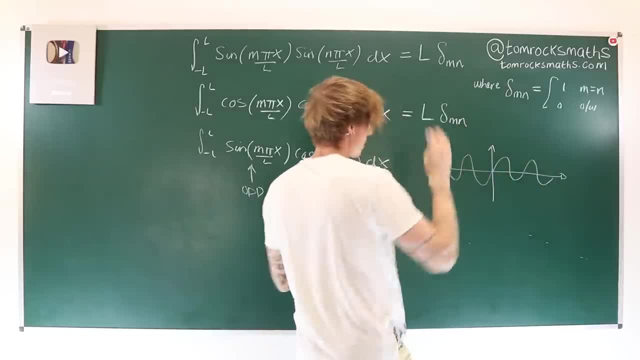 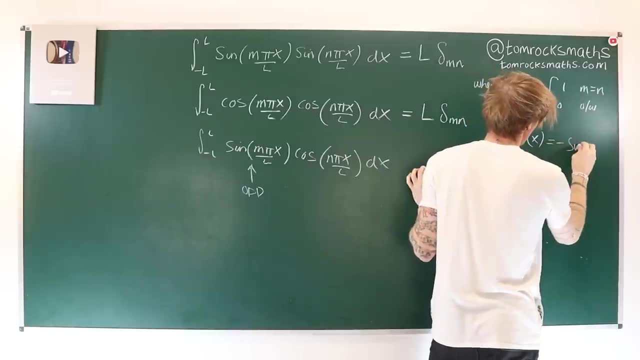 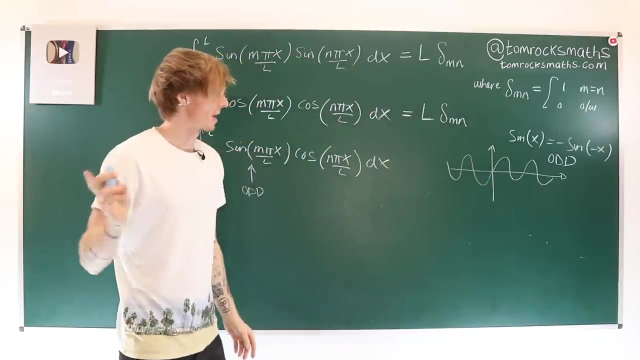 something like this, and then it's kind of reflected over here. So we say that sine, or it's true that sine of x is equal to minus sine of minus x, And that's how we define an odd function. So it's odd. I like to think of it as almost like being flipped in the line y equals x, Now cos. 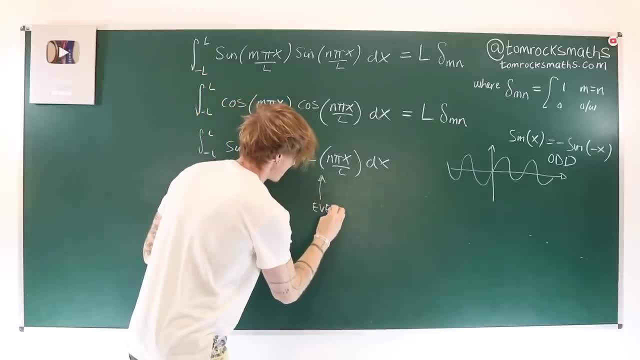 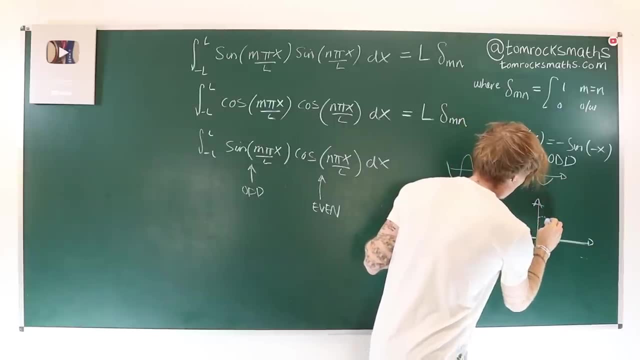 is even. Cos is an even function, And what that means, if I draw the graph of cos, is we start at the top, we go down and then we come back up and then down, and then we go up and then down. I like that. 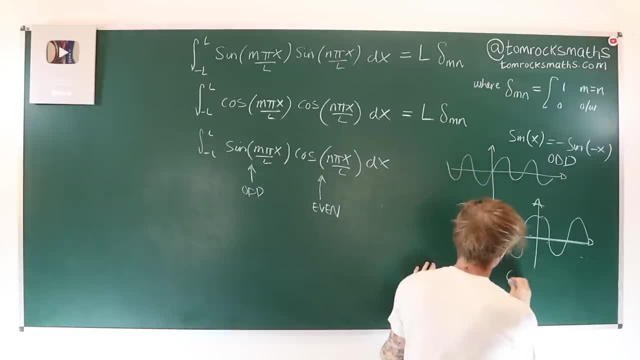 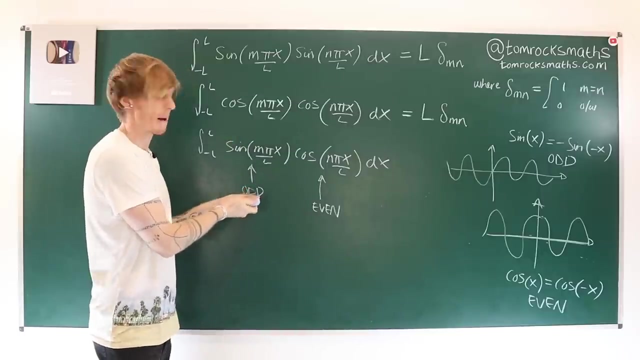 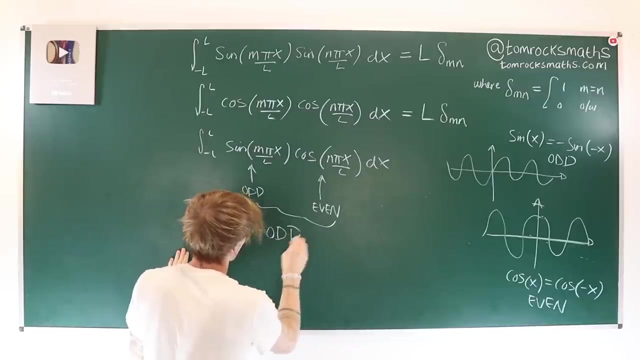 And that is reflected in the y-axis. So we know that cos of x is the same as cos of minus x, And that defines an even function. So because we have an odd function multiplying an even function together, we have, overall, an odd function. And this works in just the same way as it would with odd and even numbers. 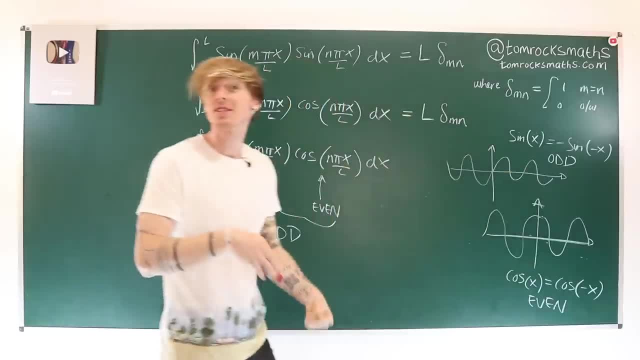 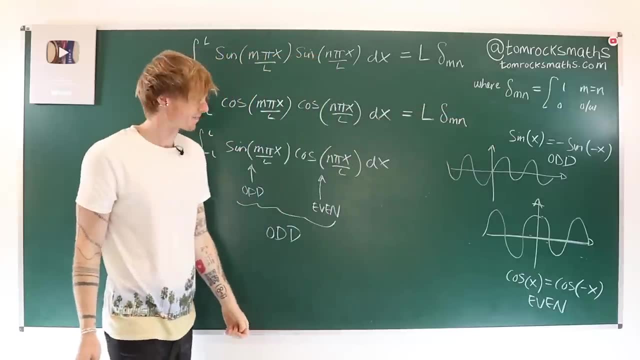 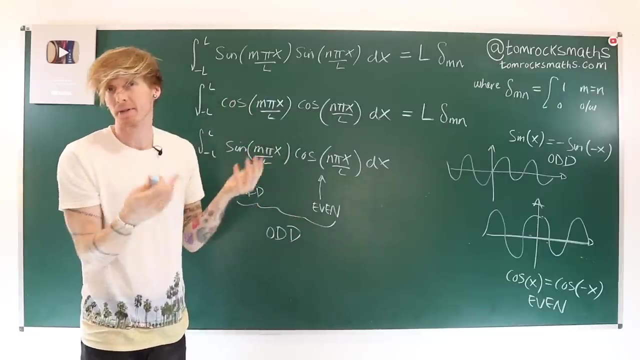 Or, if you want, you can follow through these definitions and convince yourself that when you multiply a cos and a sine, it does satisfy the property of being an odd function. So this whole thing is odd, So whilst we could try and work out its shape, but of course that 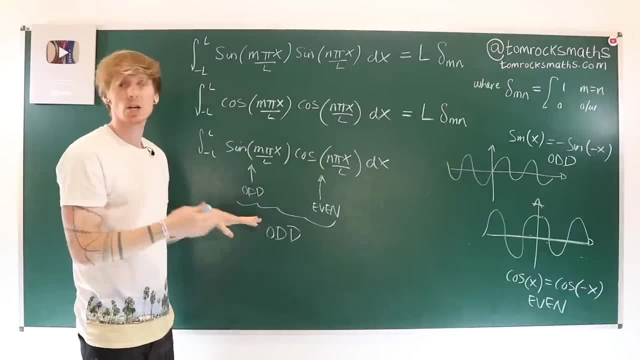 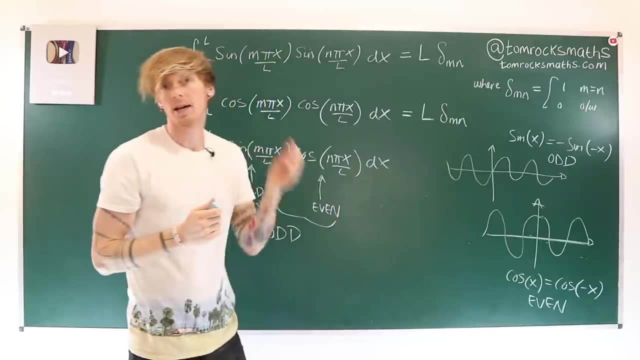 will vary for different m and n. the fact that it's odd tells us that we have this sort of reflective symmetry in the line y equals x. So we can see that this is an odd function. So we can also try and work out its shape. but of course that will vary for different m and n. The fact that it's odd tells us that we have this sort of reflective symmetry in the line y equals x. 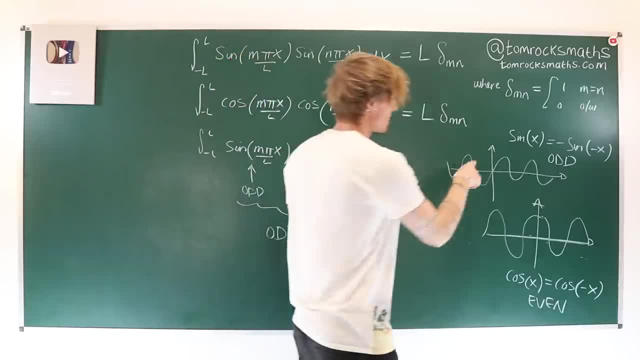 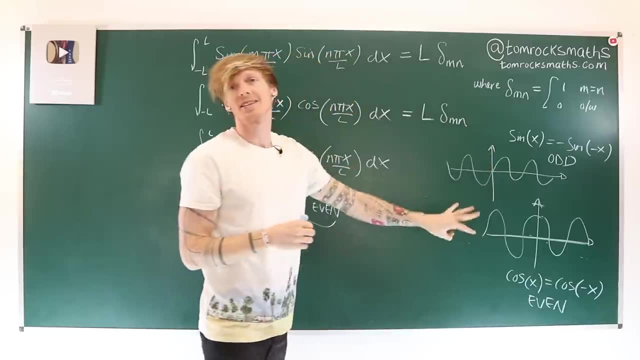 y equals x or y equals minus x. So what that's going to mean here is, whatever we have on one side of zero, we're going to have, like, the exact negative on the other side. So when we do the integral- and this is true, in fact, for any odd function- 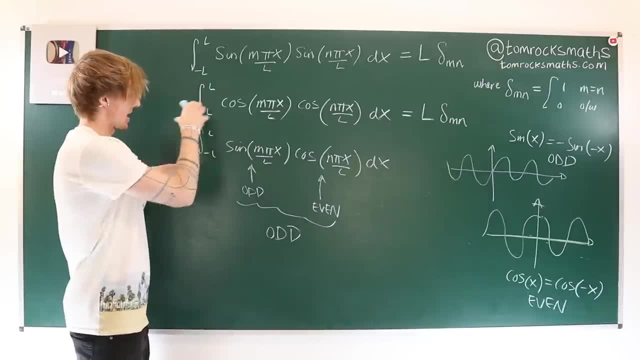 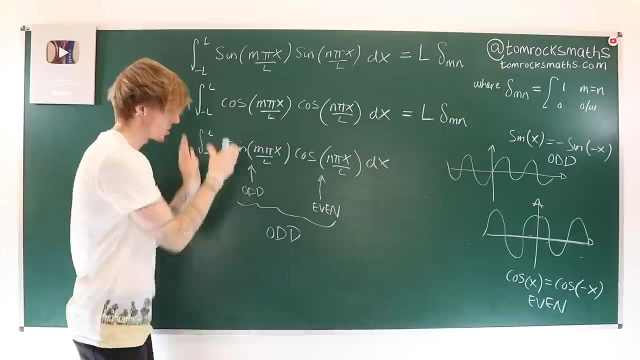 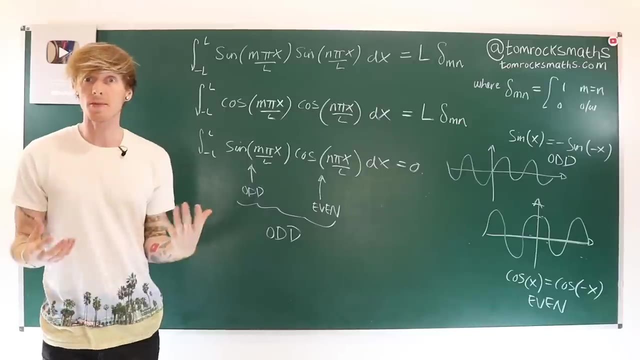 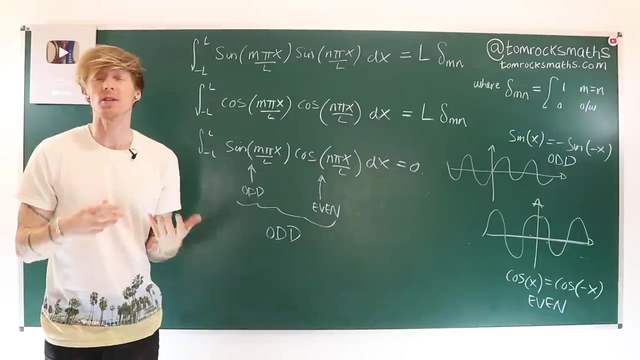 if you integrate any odd function over an interval which is symmetric about zero, you will always get zero, So we can use this property to immediately conclude. this is in fact going to give us zero. So, in summary, we have a total of three orthogonality relations which are going to be incredibly important when deriving our Fourier. 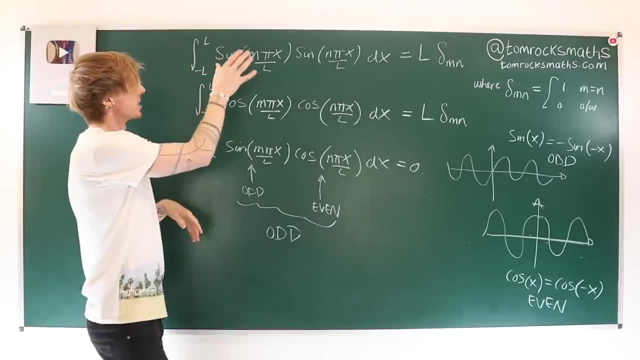 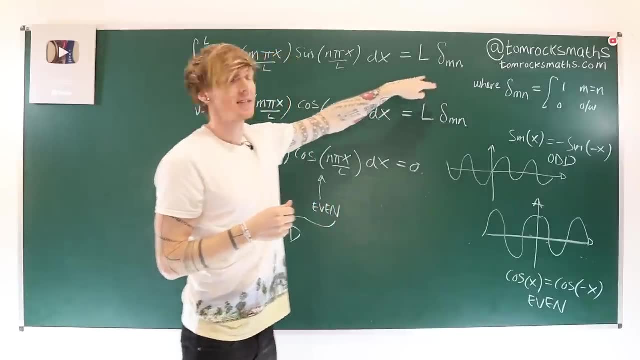 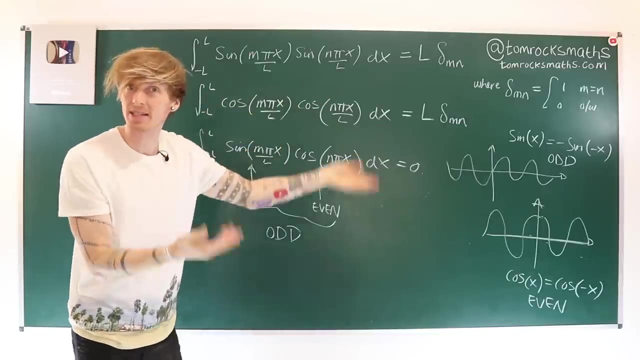 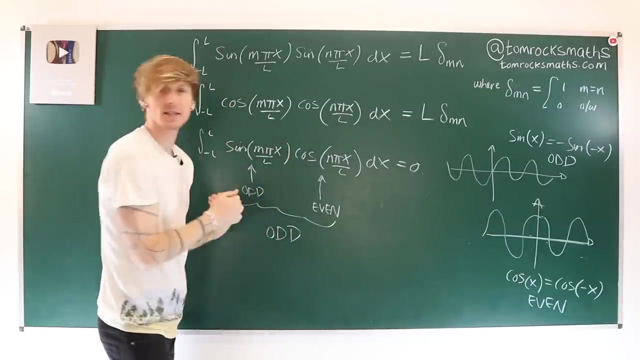 theory. The first one tells us that two sine terms, when multiplied together and integrated, we get zero unless they have the same integer, m and n For cos. we see that again, we get zero unless they are the same cos term. And if we have a sine and a cos, because that's. 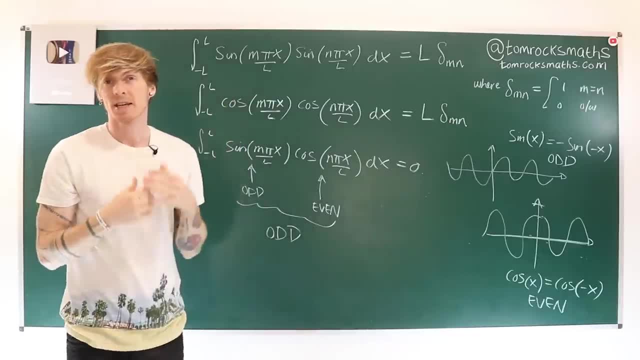 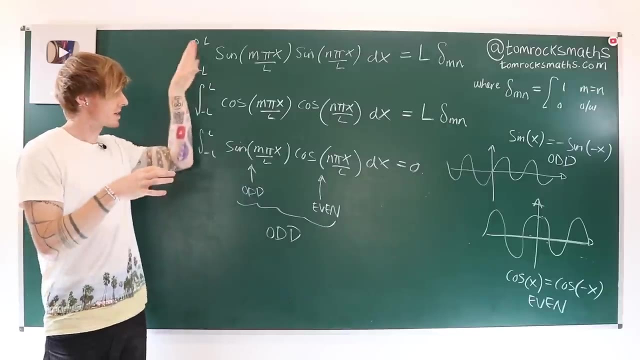 an odd function that will always integrate to give us zero. And these three relations are actually going to be key in deriving the coefficients for our infinite series of cos and sine terms. Now, some of you may have noticed that these orthogonality relations that we've just derived are 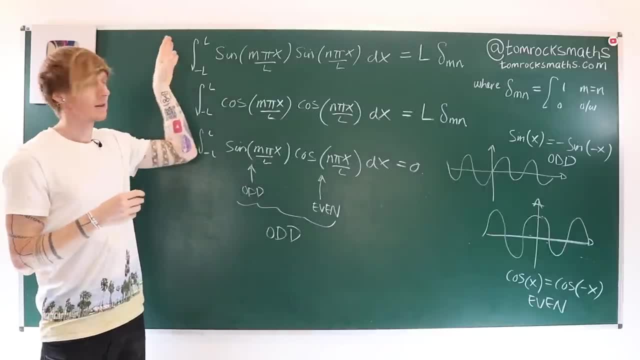 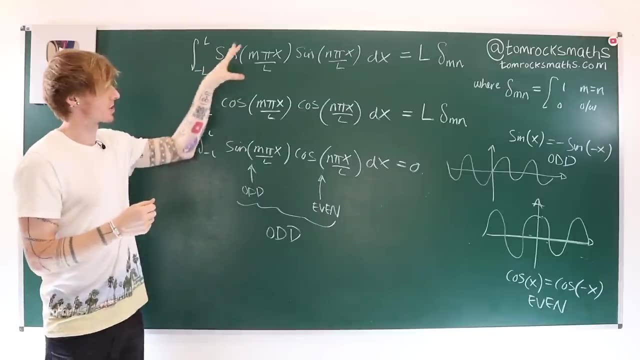 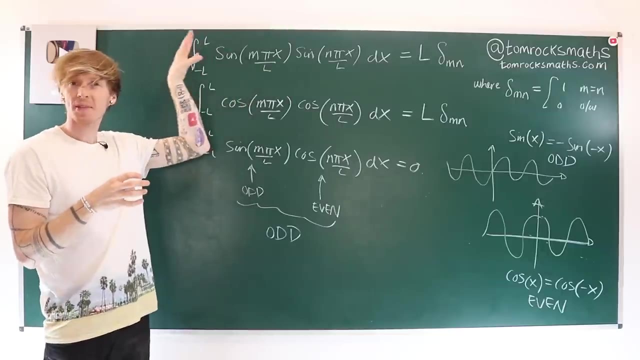 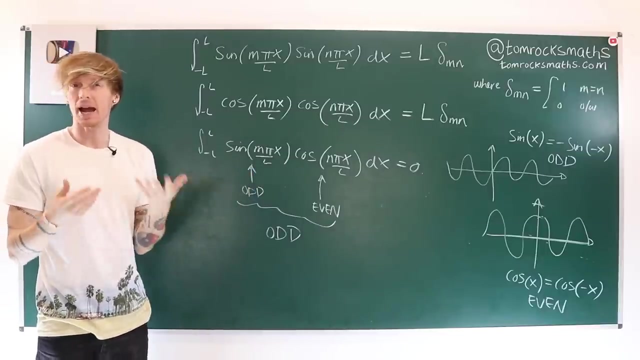 for integrals from minus l to l. Now we definitely need an interval of length, 2l, because our functions are 2l periodic and that's clearly an important relationship between the function and the interval over which we're integrating. But a perfectly valid question might be to ask: 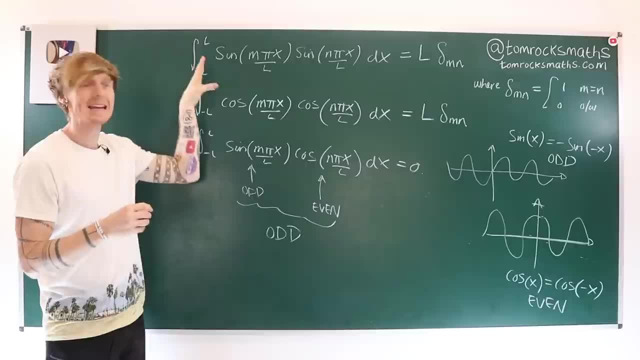 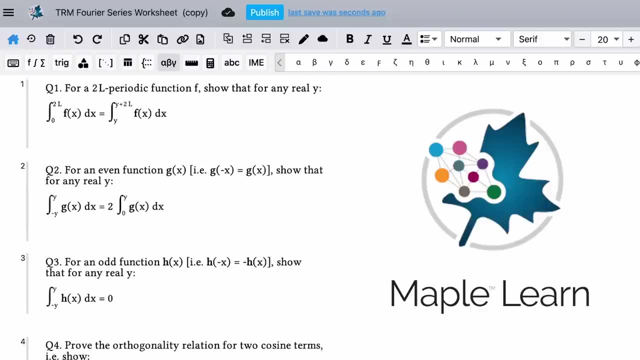 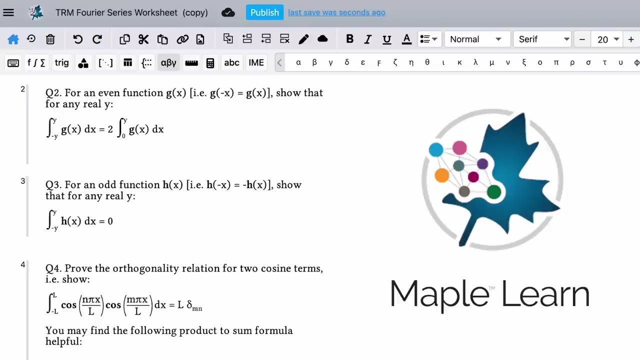 do we always get the same results here over any interval of length: 2l? If you wish to investigate this further, then I recommend checking out the MapleLearn worksheet linked in the video description below this box, which takes you through a step-by-step proof of this property. I've also included some exercises looking at the 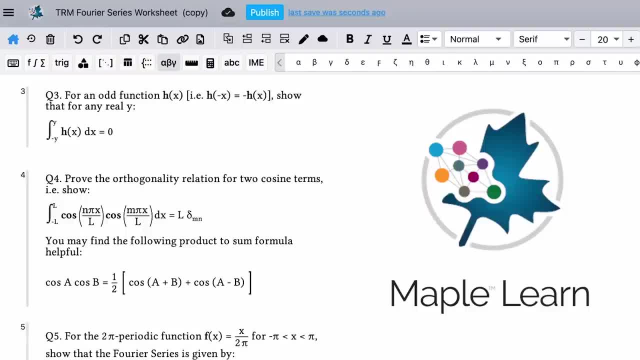 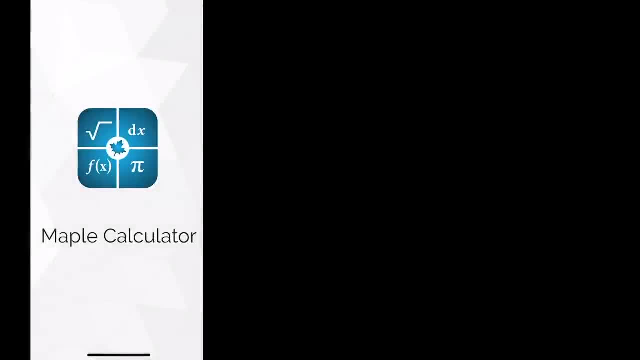 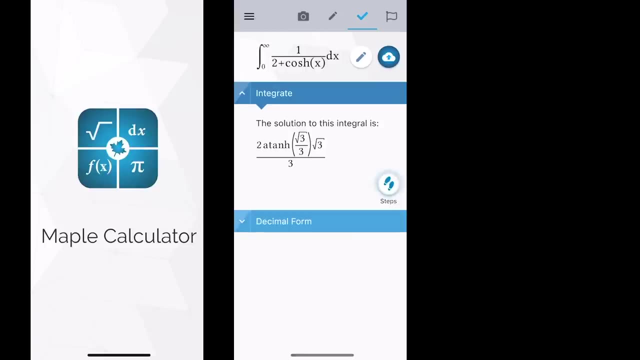 properties of odd and even functions, as well as some further exploration of the orthogonality relations that we've just derived. And if you get stuck with any of the questions, then don't forget, the Maple Calculator app is here to help. Just download the app onto. 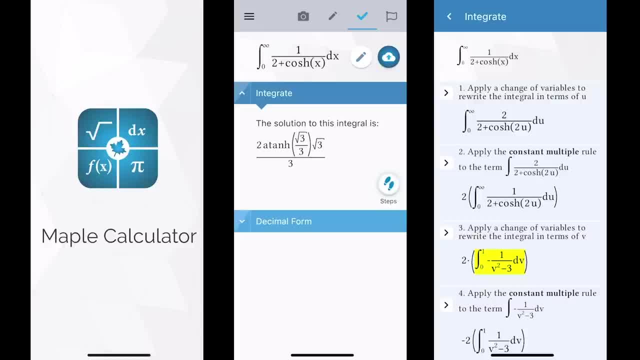 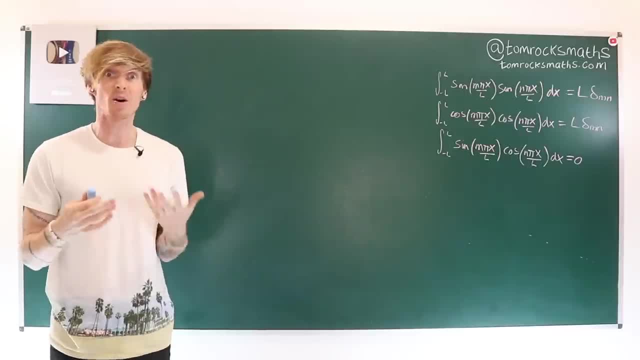 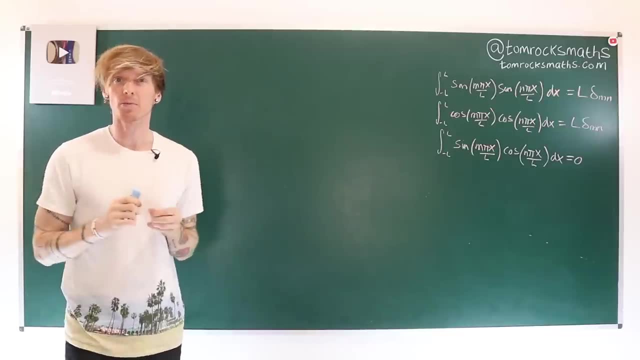 your phone, take a photograph of the equation you want to solve and then click the steps feature to see a breakdown of the solution. Now that we have the orthogonality relations, let's put them to use in deriving our Fourier series. So we begin with a general function f of x, which is 2. 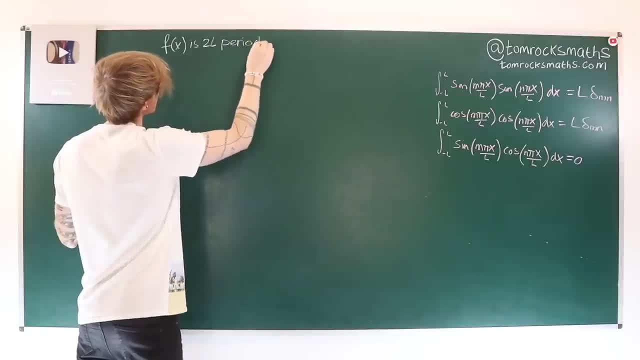 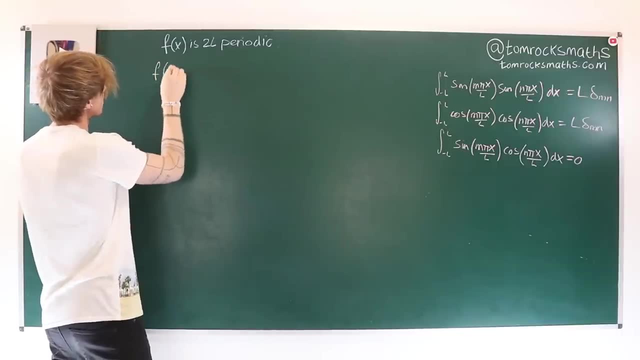 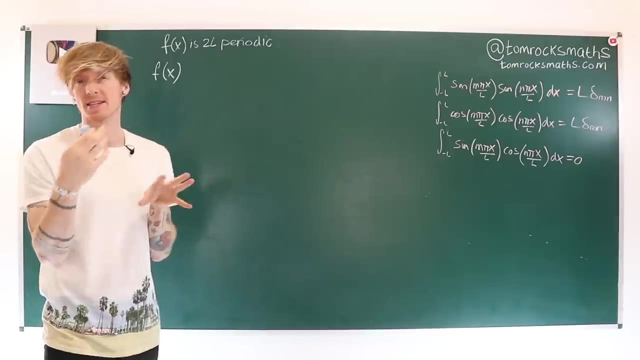 l periodic, where of course l can be any number, And what we want to do is rewrite f of x as an infinite series, an infinite sum of cos and sine terms. So let's suppose that is possible, Let's just go with it and see what happens. So, assuming we can do this, 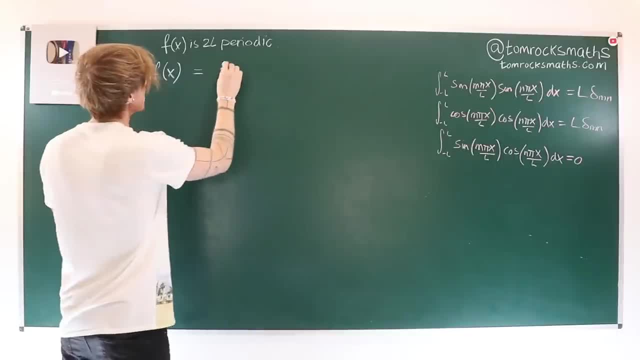 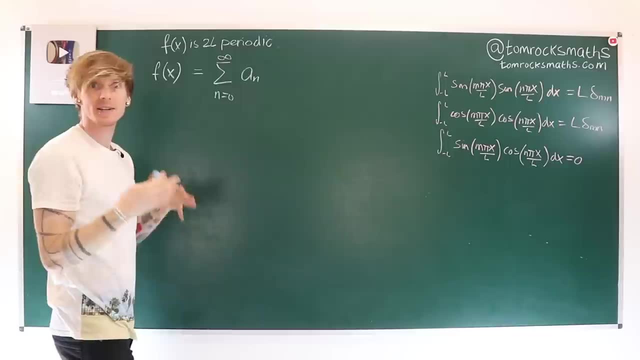 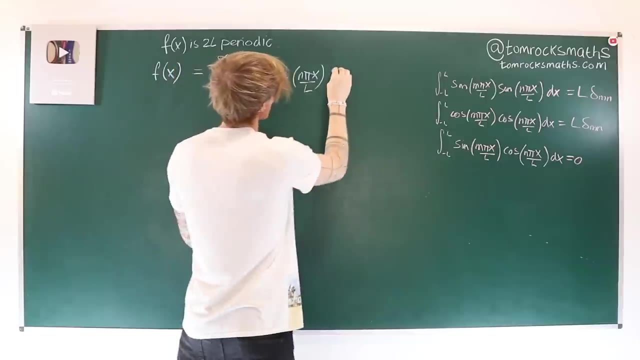 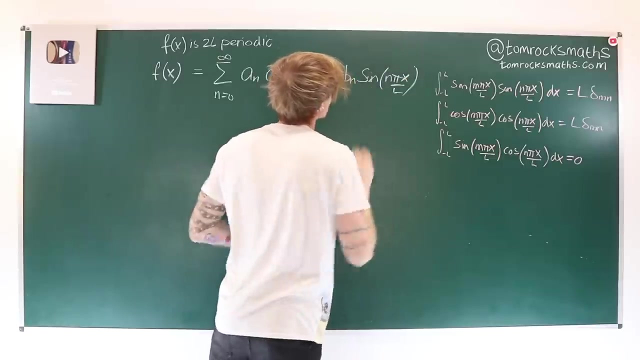 we can rewrite: f of x is equal to the sum from n equals naught to infinity, of the unknown coefficients a? n times cos of n pi x over l, plus the unknown coefficients b? n times sine of n pi x over l, And the idea is that adding together all of these terms is going to give 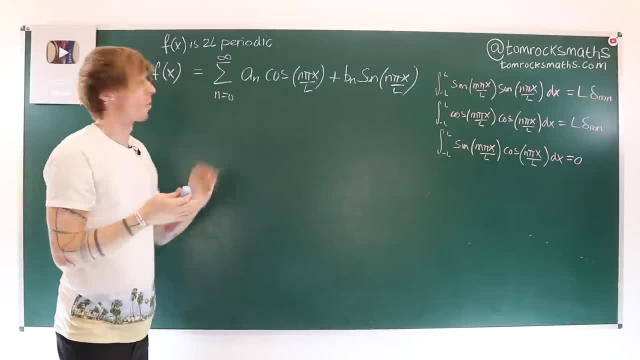 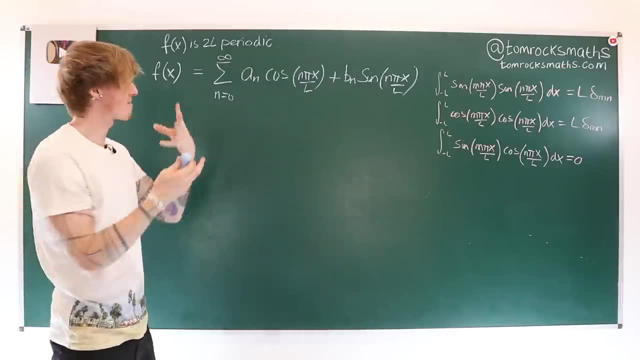 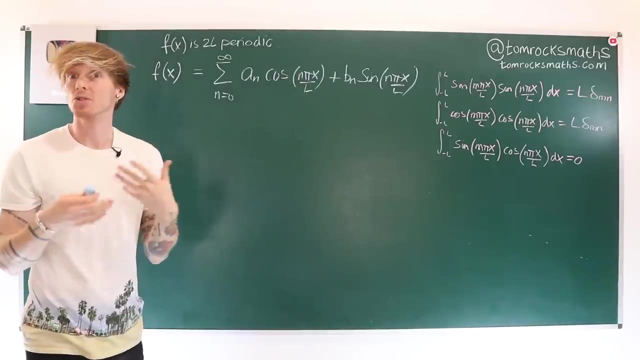 us f, But of course we need to determine what these coefficients are. Just saying this exists doesn't really help us when we're trying to solve a problem. We need a method of determining the coefficients a, n and b. n. Now, if we focus on n, equals naught first. So when n is equal to zero, 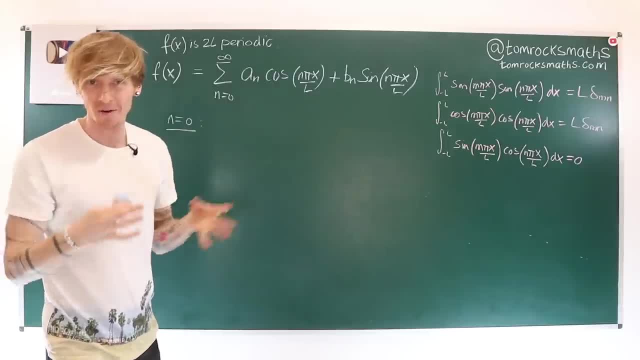 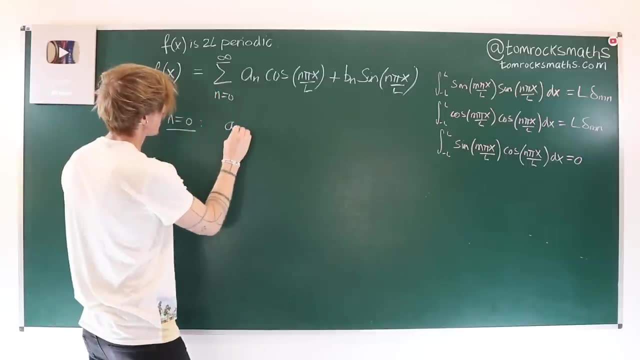 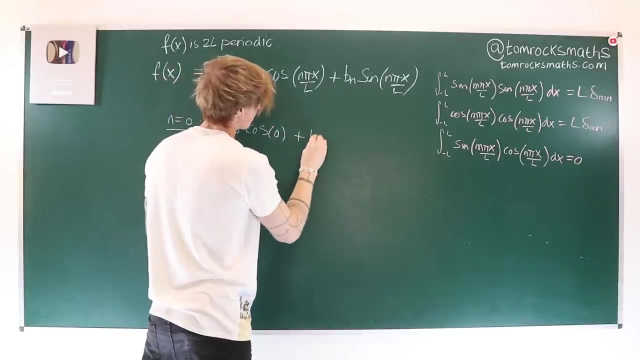 and this is the only one we're going to do. I'm not going to go through all different values, but there's something special about n equals naught. So when n equals naught, we're going to get a zero times cos of zero plus b zero times sine of zero. 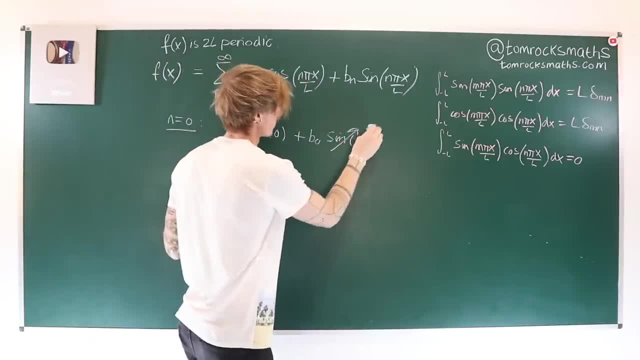 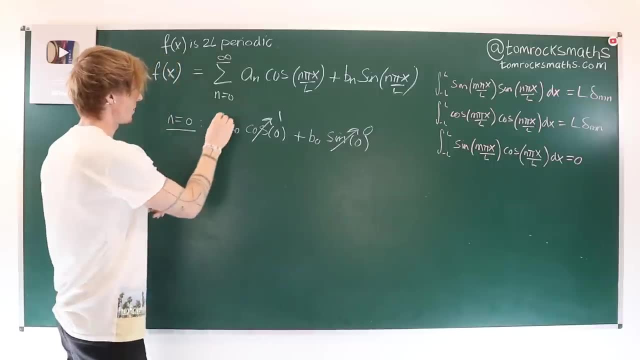 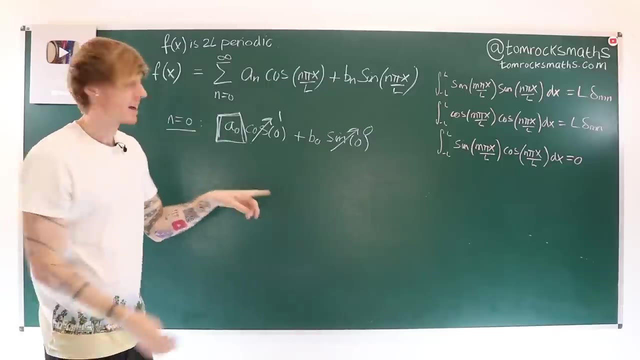 Now, sine of zero- well, that's just naught. and cos of zero- well, that's just one. So all we're left with here is actually going to be this first coefficient, a zero. So this is a much simplified case when n is specifically naught. 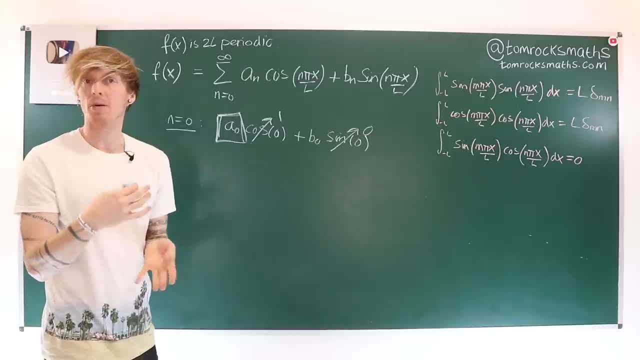 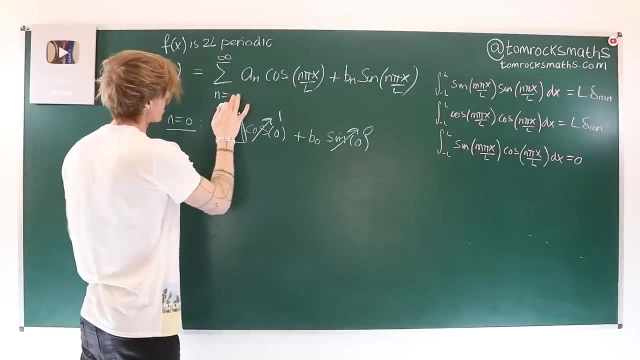 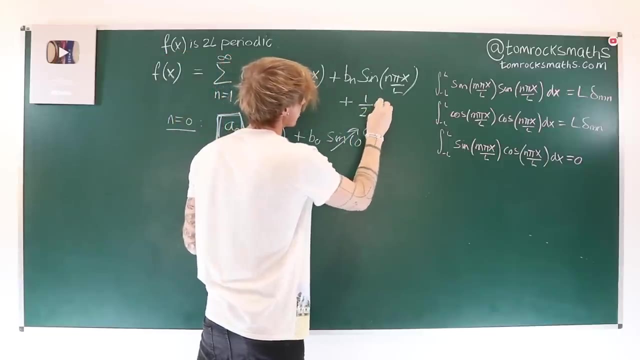 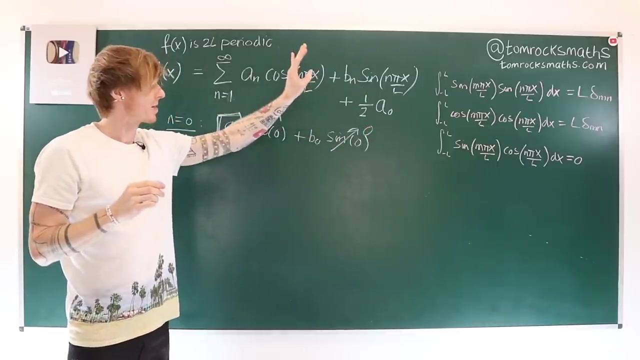 And so what we tend to do in our definition of the general Fourier series is in fact to start the sum from one, and then we add in what we call the zero coefficient, which is often one labeled as a half times a zero. The choice of the half there will become apparent shortly. 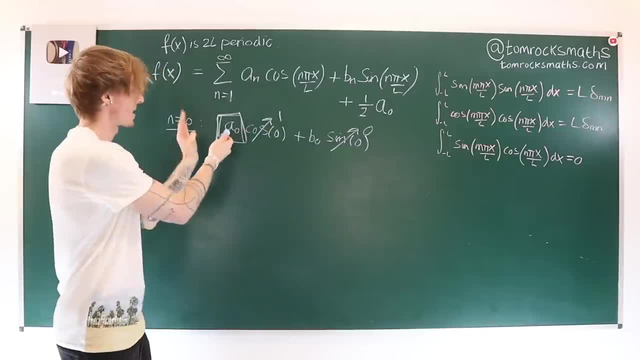 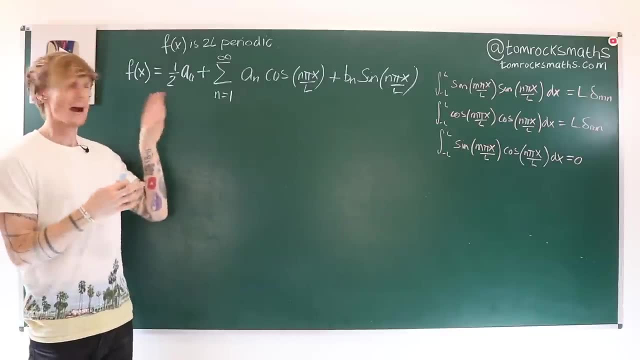 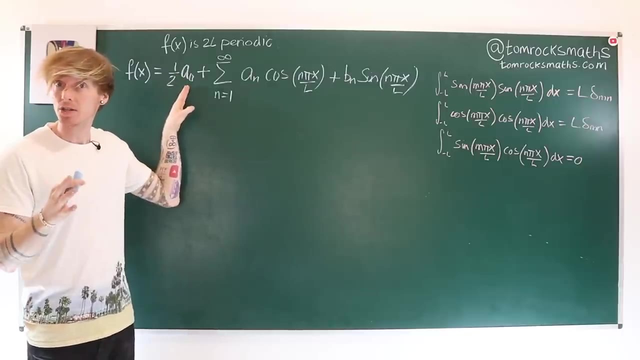 but for now, you can see, this is a constant, because when n is naught, we're going to get a constant term. So the question now becomes: how do we calculate our three different coefficients? We want a formula for a naught, the constant term, a formula for a- n and a formula for b- n. 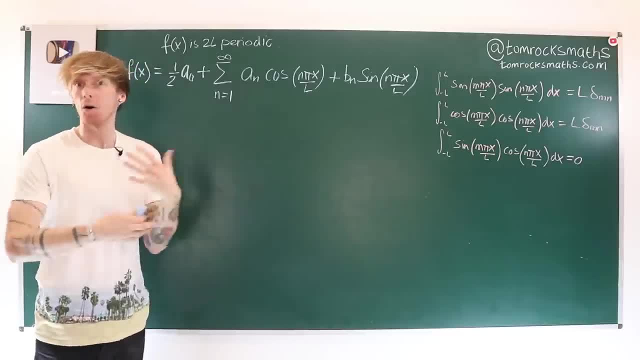 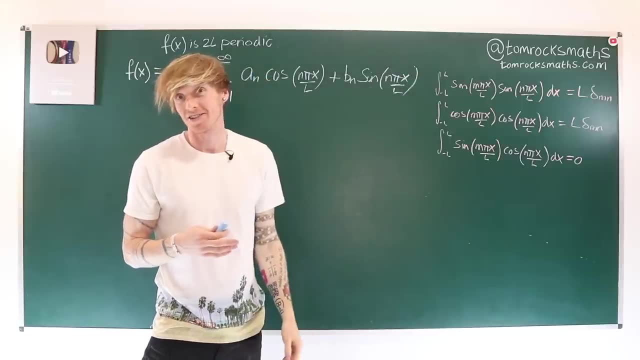 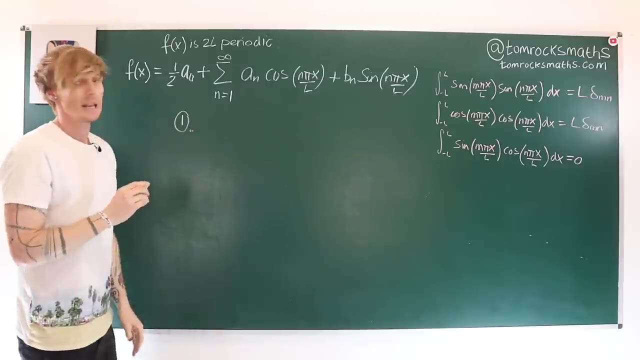 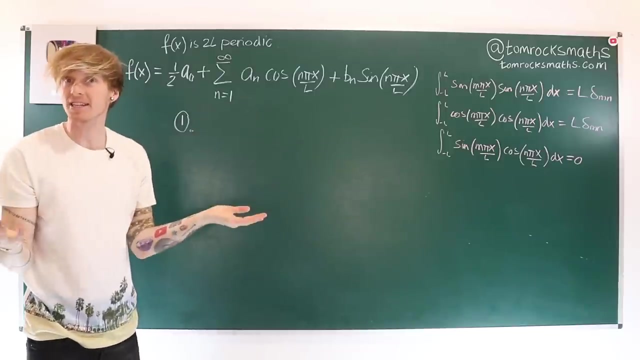 And the trick here, which really all of the theory of Fourier series relies on, is going to be to use our orthogonality relations. So, to begin with coefficient one, let's take this equation which, remember, we've assumed exists, this Fourier series we're saying, suppose it exists, let's see how we might. 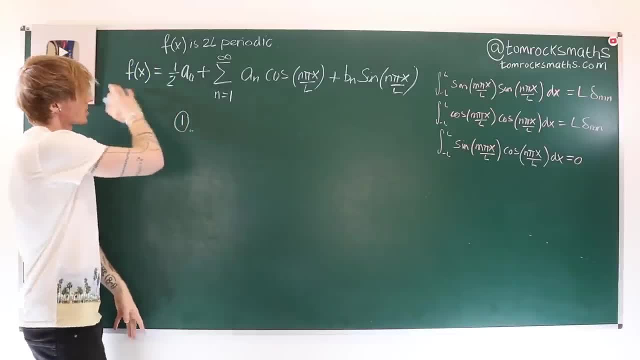 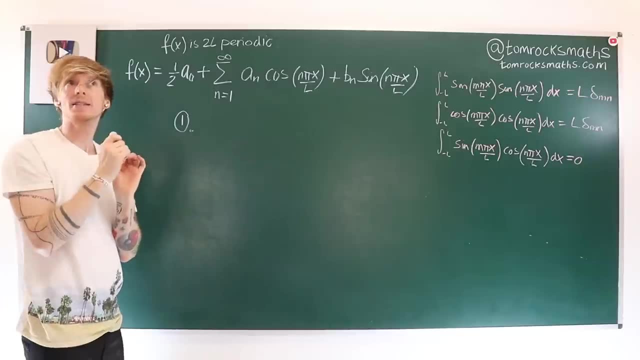 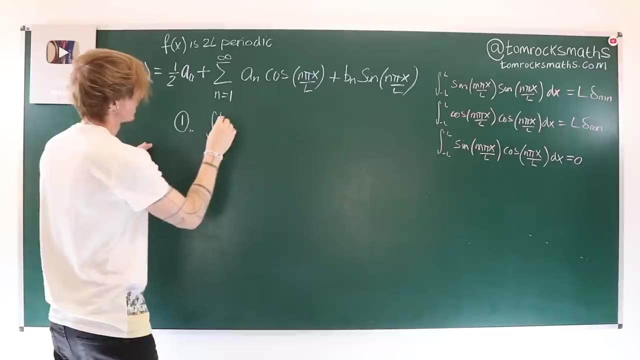 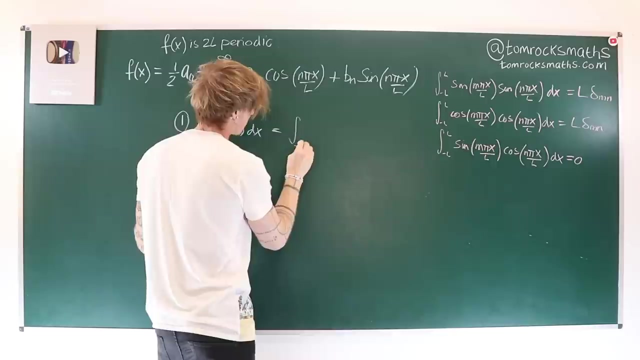 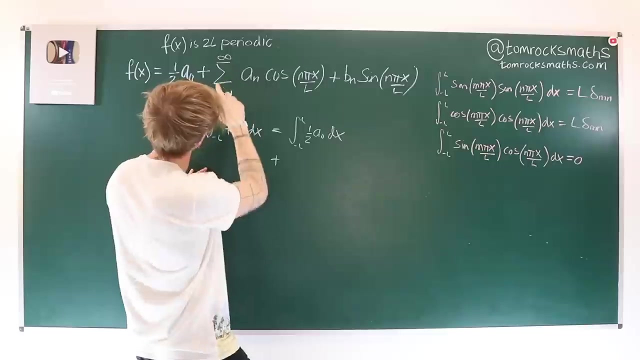 calculate the coefficients. So let's take this whole equation and let's integrate both sides of the equation, from minus l to l, So we can say: minus l to l times f of x dx is equal to the integral from minus l to to L of a half a naught dx plus the sum. and here what I'm going to do is take 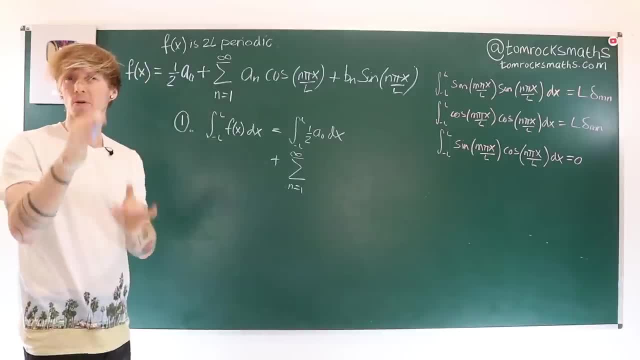 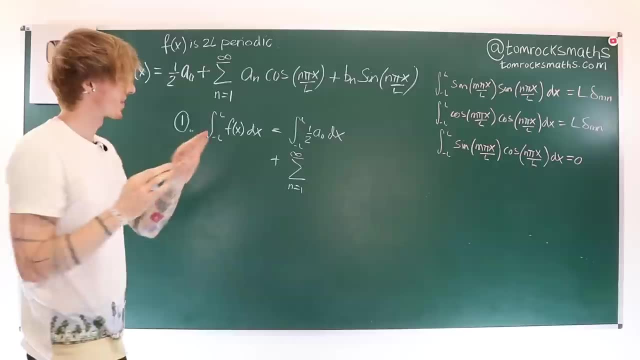 the integral inside the sum. I will talk more about that. well, I will talk more about why that's allowed at the end of the video, but for now let's just go with it. I'm going to take the integration inside the sum and say: this is then the. 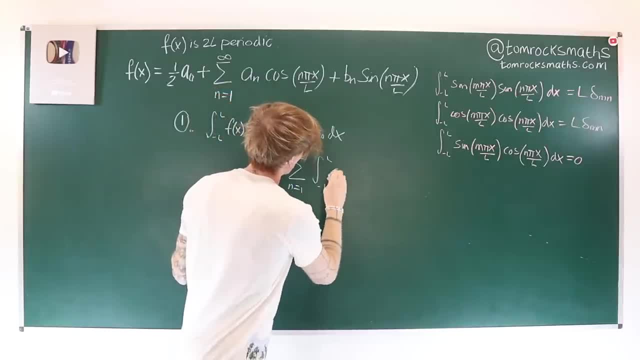 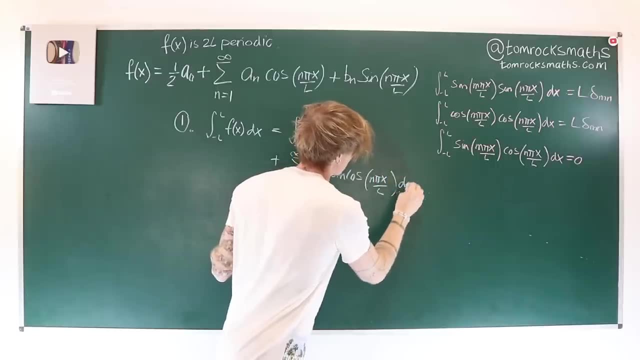 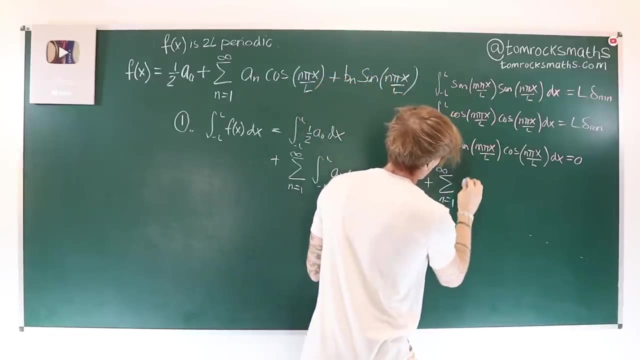 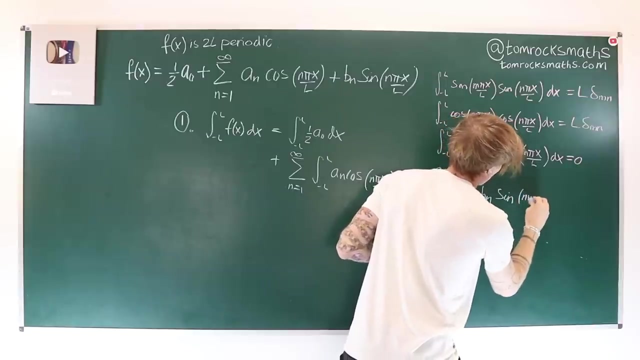 integral from minus L to L of An cos n pi x over L dx. and then we've got another infinite sum integral minus L to L of Bn sine n pi x over L dx. now what do we get when we get a integral from minus L to L of an cos n pi x over L dx? Well, if we get a integral from minus L to L of bn sine n pi x over L dx, Now what do we get when we 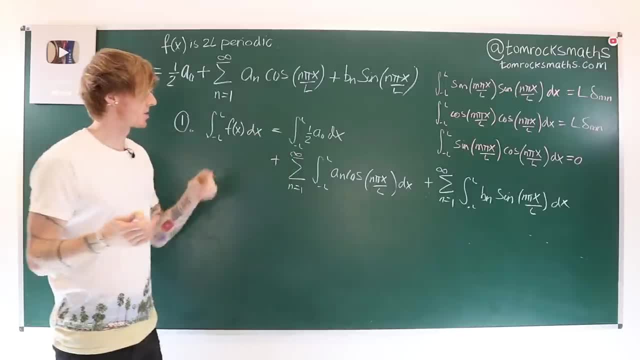 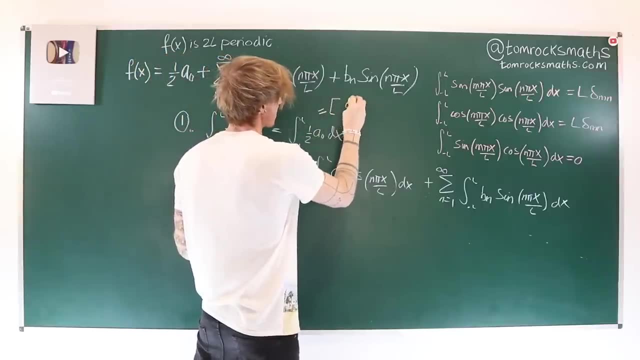 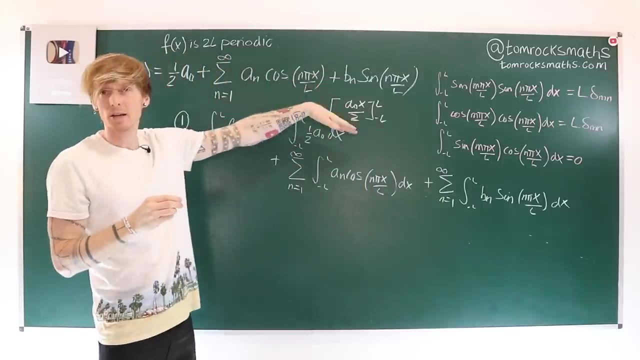 we do these integrals Well. this one's relatively straightforward. This is just a constant. so when you integrate a constant, this just gives me a naught x over 2 between L and minus L. so that will be a naught L over 2 minus minus a. 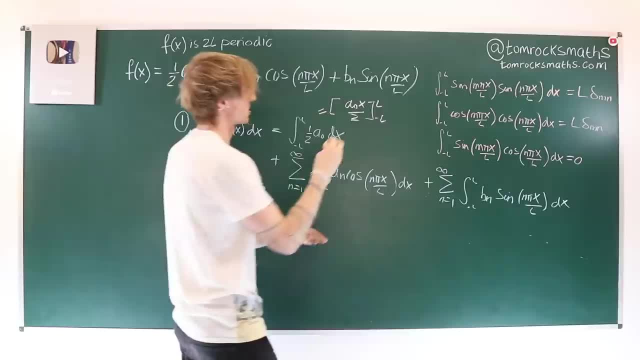 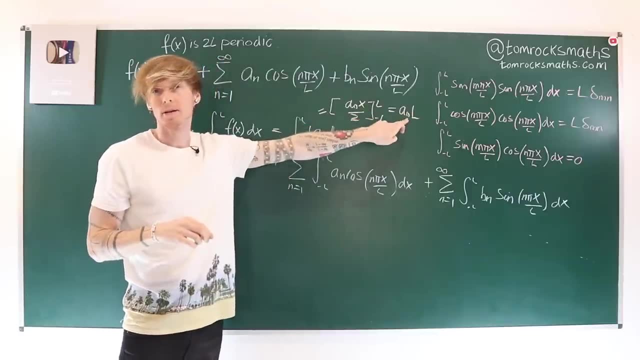 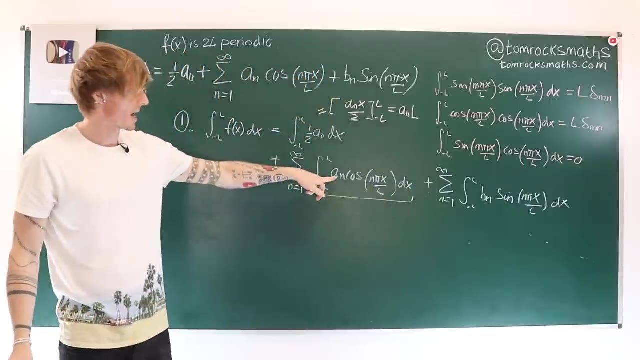 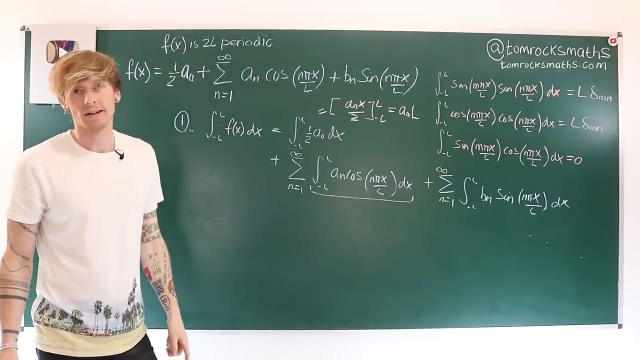 naught L over 2, so I'm just going to get two lots of it. so it's going to be a naught L. So this first integral here gives me a naught multiplied by L. Now this one, we have a constant an multiplied by cos n Pi x over L. Now if I 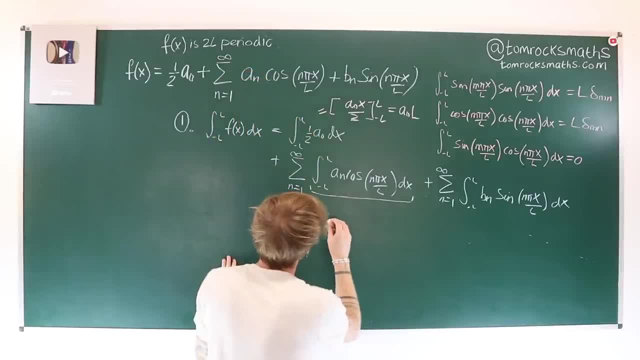 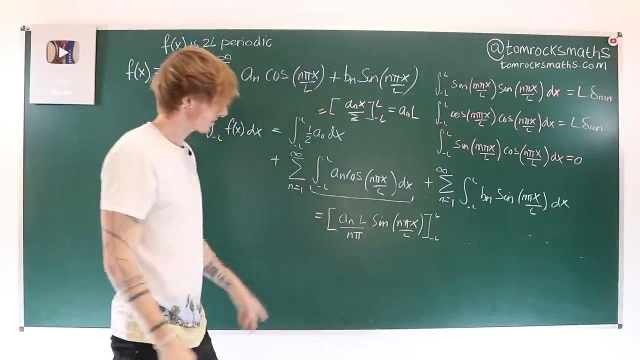 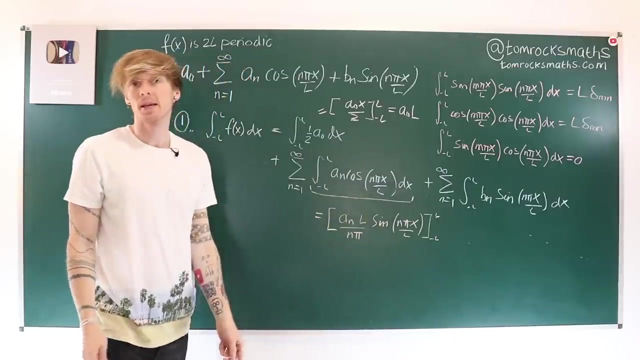 integrate cos, so that will give me a n. and then I've got to remember to do l over n pi, and then I'm going to get sine of n pi, x over l, between minus l and l Now, when I substitute in these values for x, so I get sine of n pi. well, that's zero. 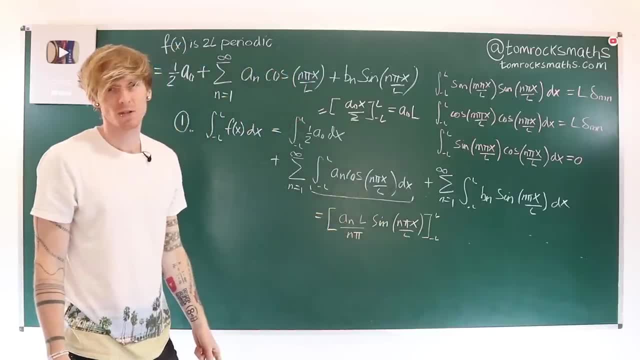 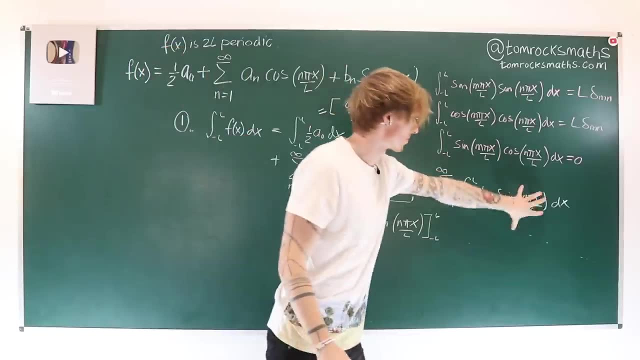 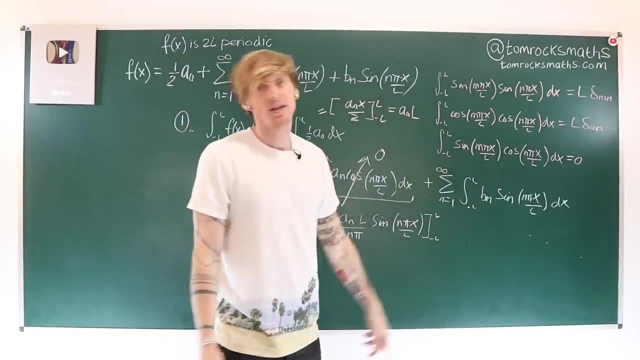 and then I get sine of minus n pi. well, that's also zero. So this whole thing is zero, in fact. and similarly, when you integrate over here, you integrate your sine, it gives you some multiple of cos and cos. at these two points they're going to actually perfectly cancel out. 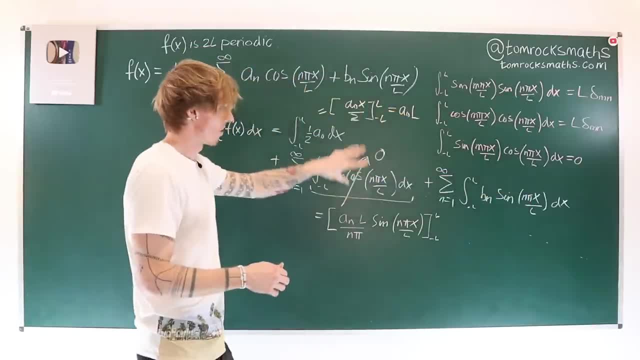 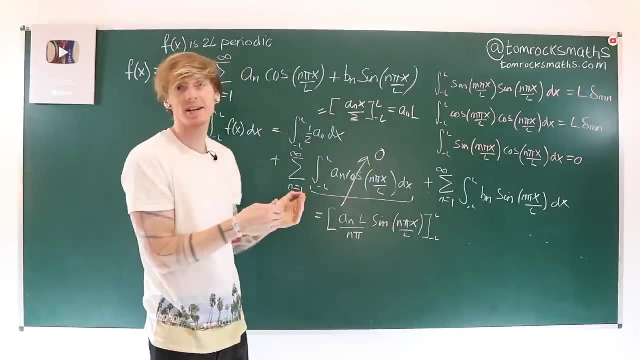 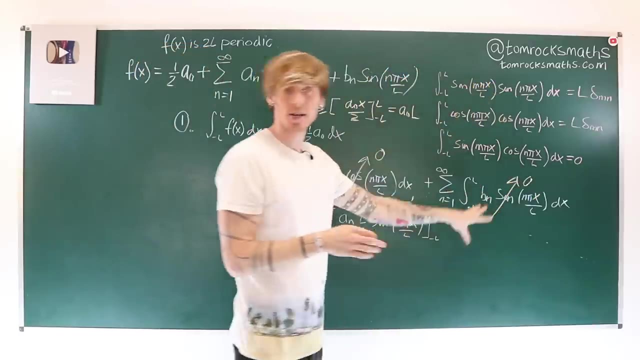 precisely because each of these functions for any value of n, each of them is actually 2l periodic and we're in integrating over period, total length: 2l. So this also gives you zero. and again, if you want to do the integral and substitute in, you can see that explicitly for yourself. So both of these vanish. 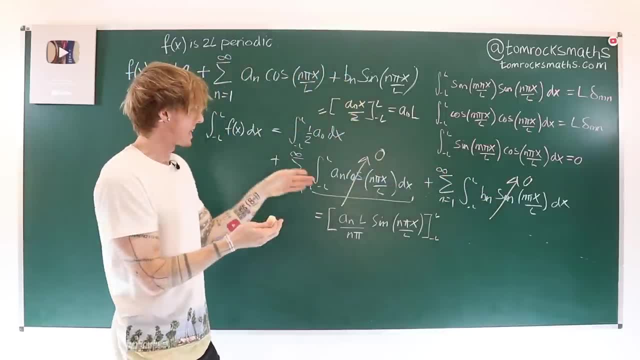 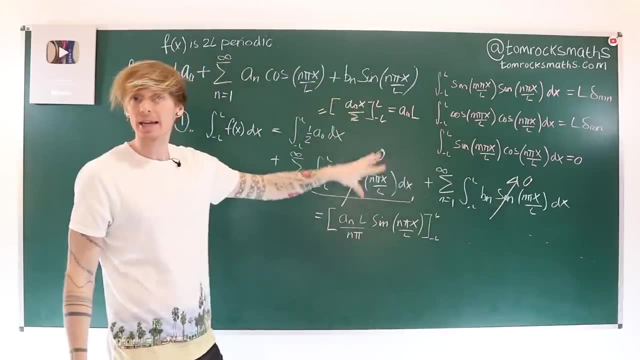 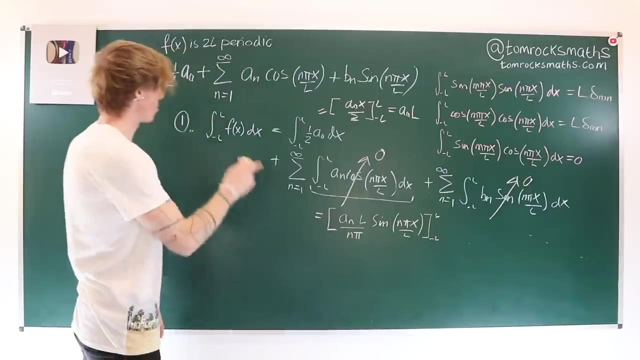 and even though there's an infinite number of them, each individual piece is always zero, because the fact that these integrals were zero is entirely independent of the value of n. So all of these pieces are zero. so all we're left with is the integral of f is exactly a nought times. 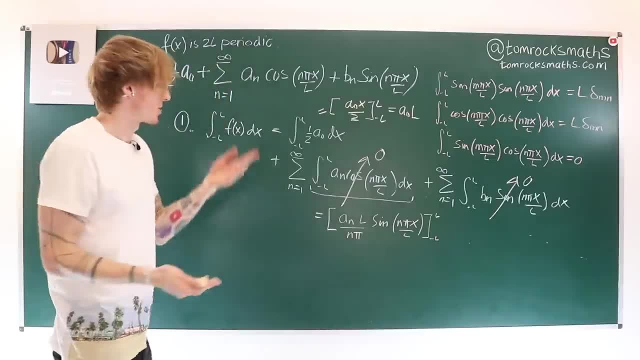 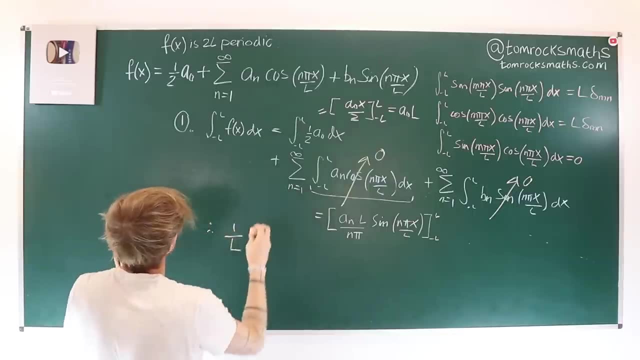 l. So we can just rearrange that equation. So putting this all together, we can just say: well, therefore, 1 over l, dividing both sides, times the integral from minus l to l of f dx, that is exactly a nought. So the first: 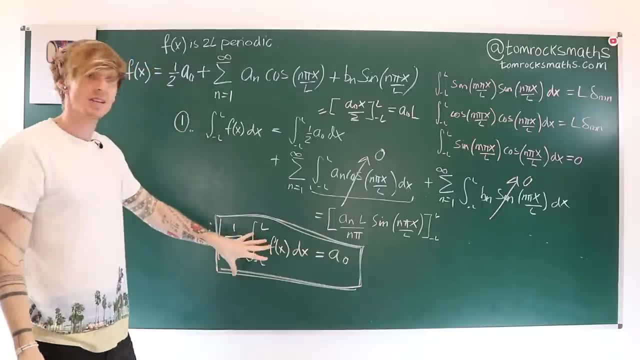 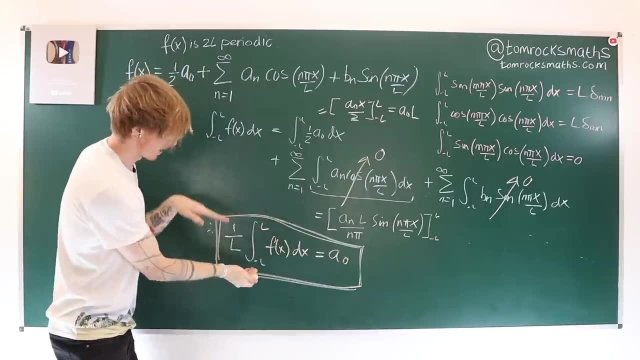 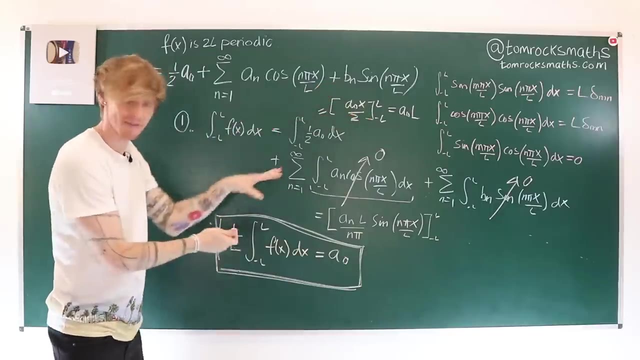 of my coefficients that I want to work out in this Fourier series is just simply given by integrating my function f between minus l and l and then putting a 1 over l outside. That is why we have the half, because it simplifies to this nice neat formula at the end. 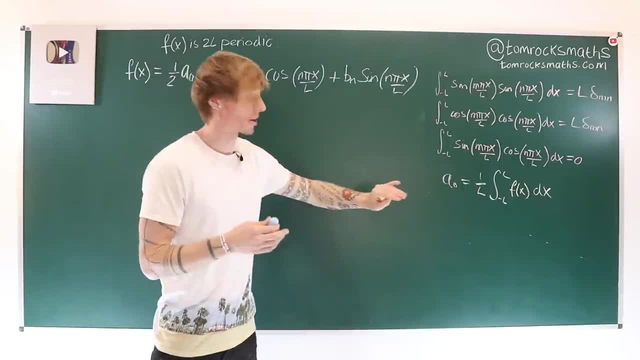 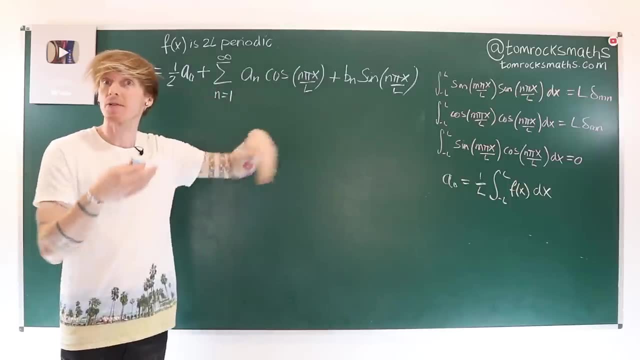 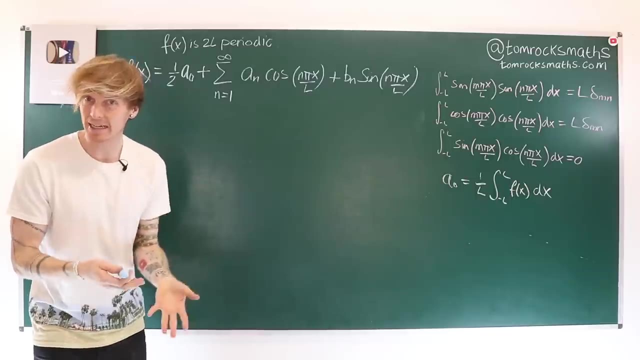 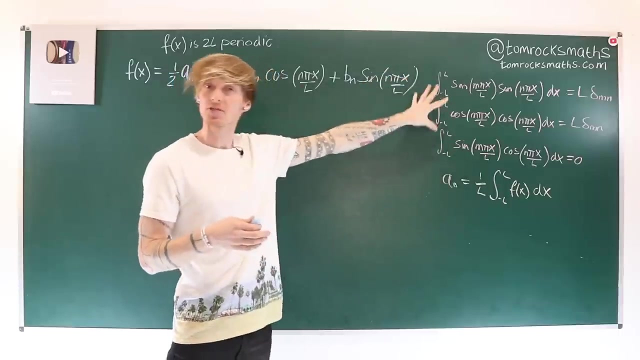 So we have the first of our coefficients, a zero given by integrating f. but how do we work out a, n and b? n for a more general value of n? The trick lies in the integration and the application of the orthogonality relations over here. So you'll note we didn't actually need these relations. 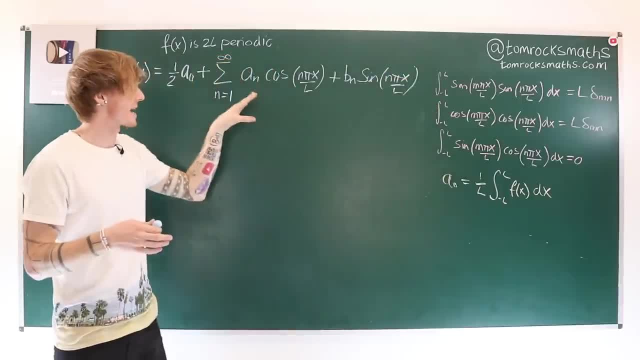 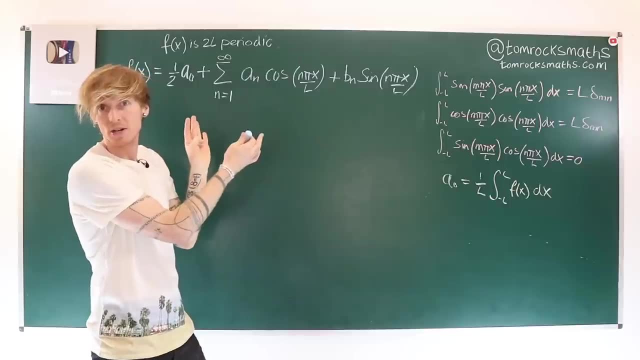 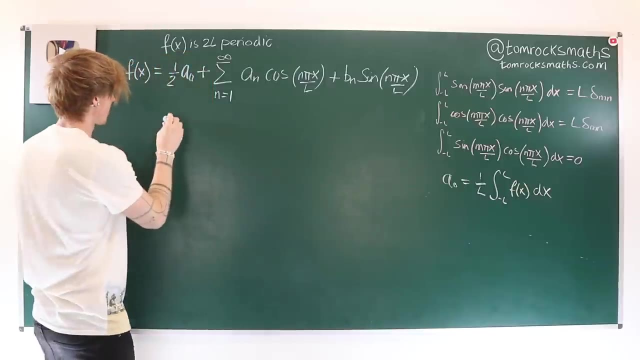 to get this first result. but what we're going to do to get a- n and b? n is actually going to be to combine this idea of integration on both sides of the expression, along with these orthogonality relations. So to get our second coefficient, we're going to take the a- n in general. 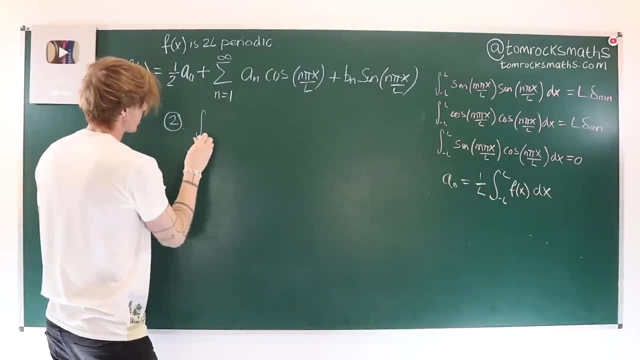 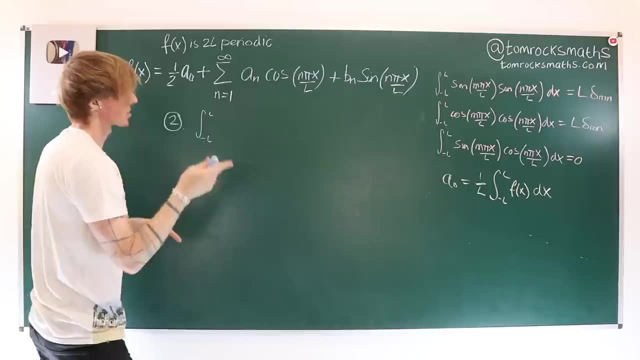 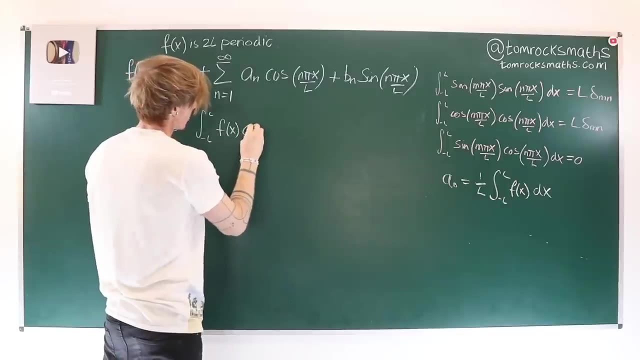 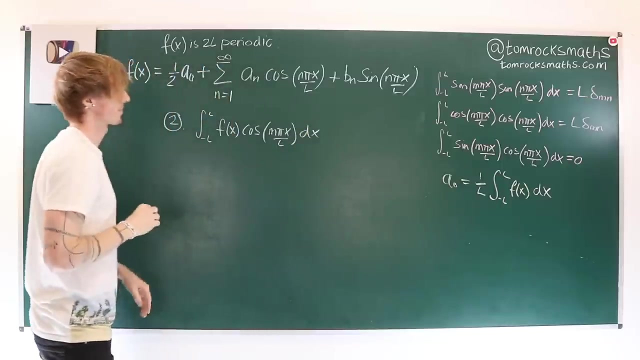 What we want to do now is to integrate both sides of the equation, but we want to first multiply by cos of m pi x over l. So the left hand side is f x cos m pi x over l dx. That's just multiplying the left by cos cos m pi x over l and then integrating. 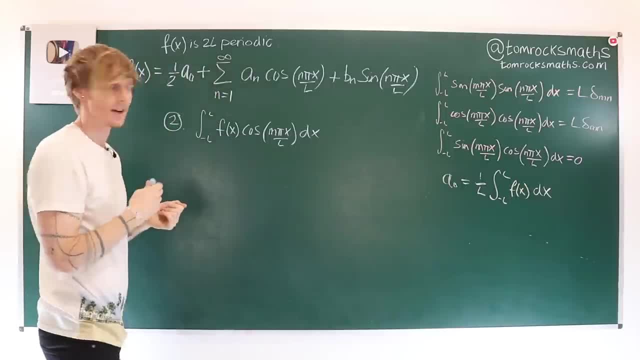 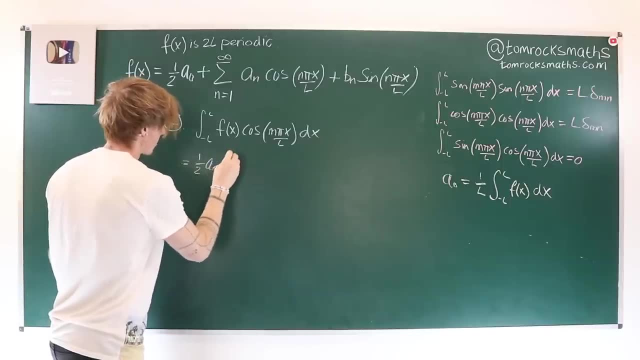 So now we have to do this for everything on the right hand side. So this is now equal to a half a naught, so I can take that out, the bracket a half a naught. the integral from minus l to l of cos. 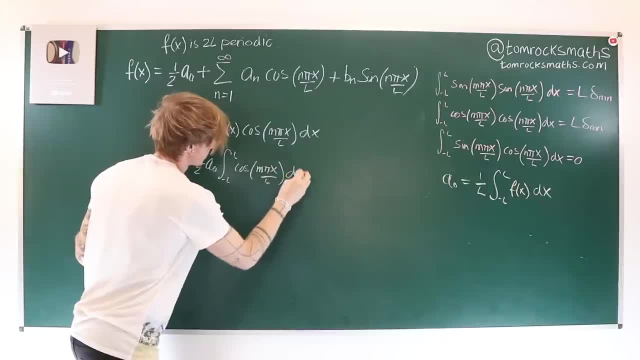 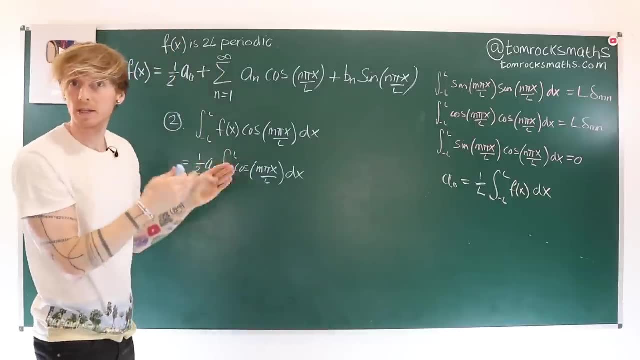 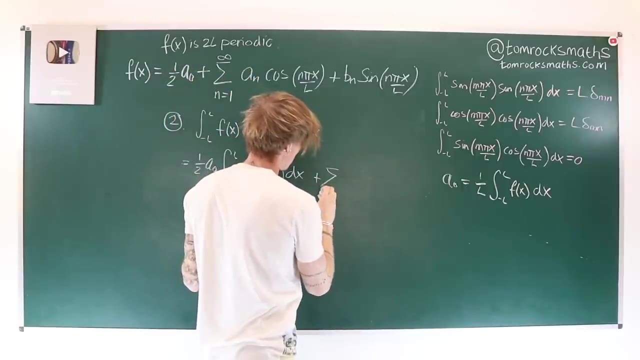 m pi x over l dx. Again, we're going to assume that it's okay to interchange the infinite sum and the integral. I'll talk about that at the end. So that then gives us a second term, which will be the sum from n equals 1 to infinity. Then we've now got the integral from minus l to l of a n. 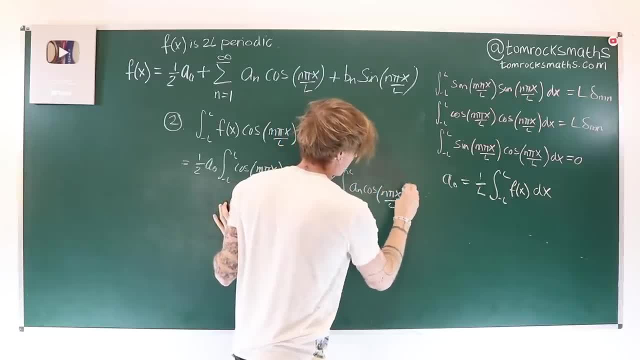 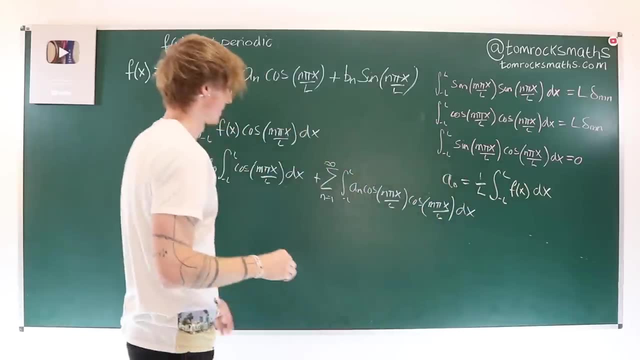 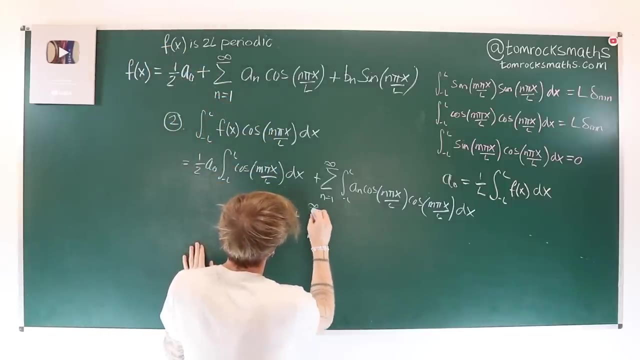 cos n pi x over l times cos m pi x. So that's the integral from n equals 1 to infinity. and then we've got the sine term. So, plus the sum from n equals 1 to infinity, the integral from minus l to l b n sine. 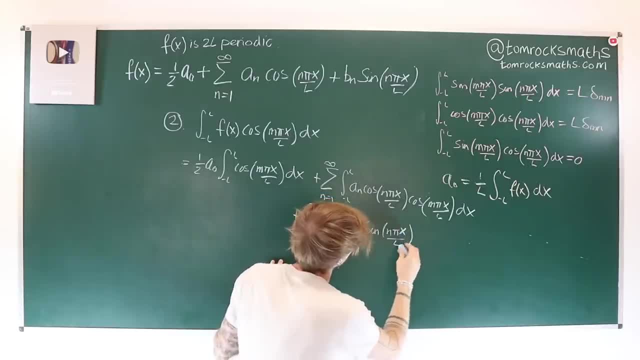 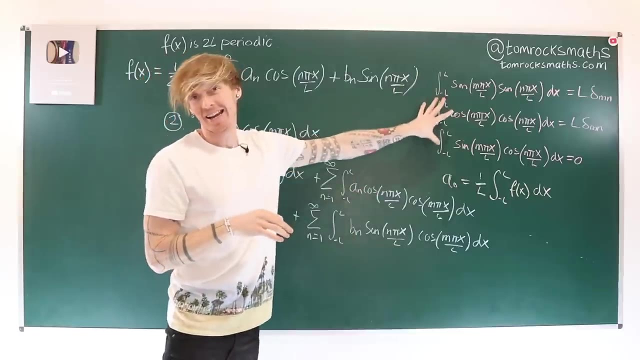 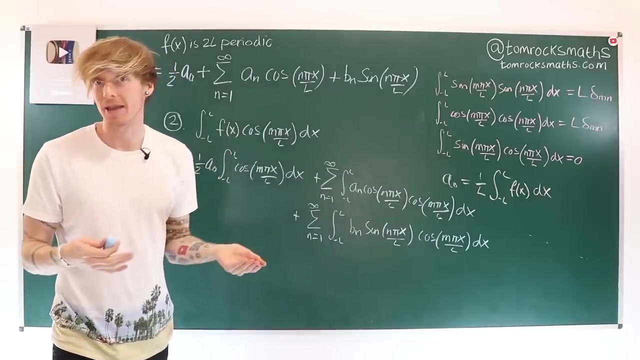 n pi x over l times cos of m pi x over l dx. So hopefully you can immediately see these two look like our orthogonality relations and that is what we're going to use to figure out what these coefficients a? n need to be. So the first integral: 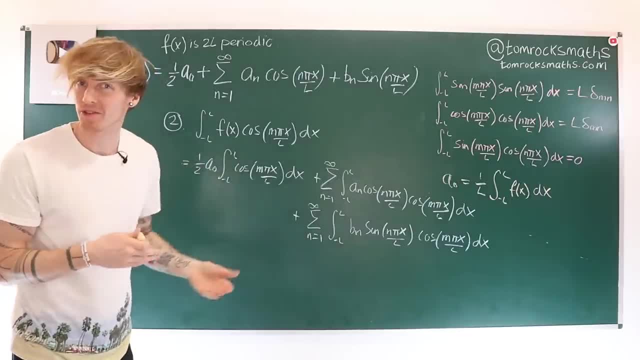 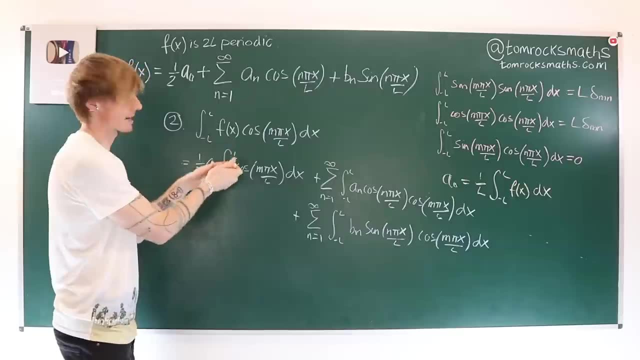 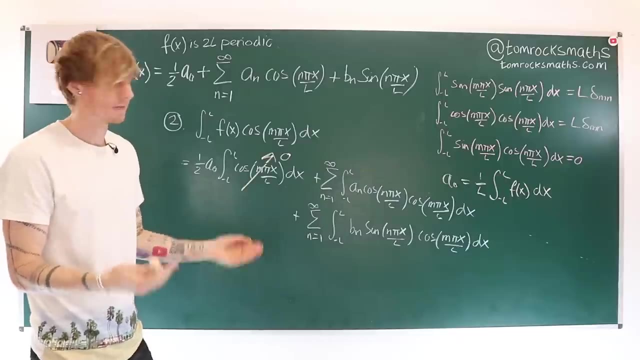 We have something very similar to what we just saw in step one for our a naught coefficient. We're integrating cos, which is 2 l periodic. between minus l and l it's going to be zero. So this is the integral there. So this is zero since 2L periodic function. Now over here let's look at this second term. 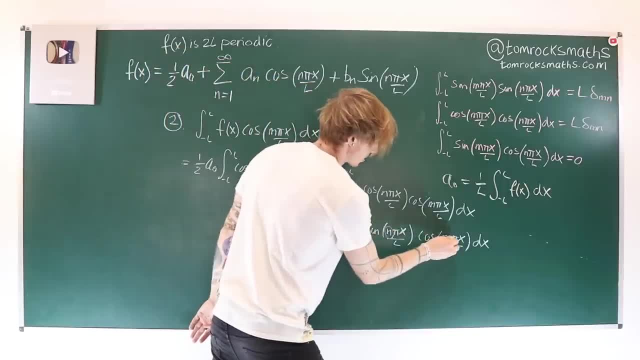 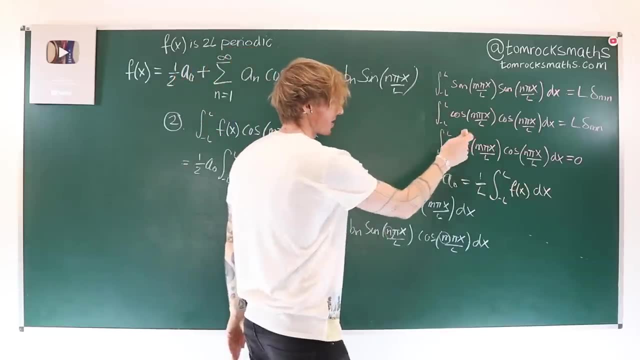 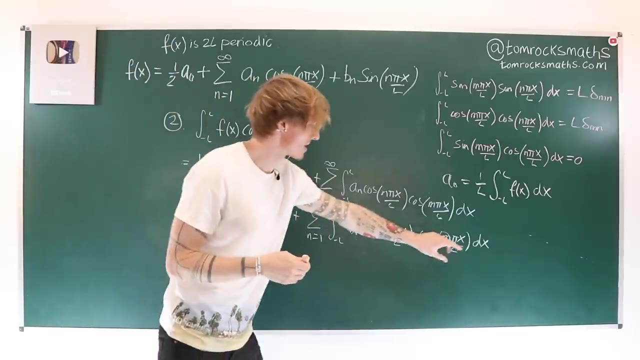 because we've got a sine of n times the cos of m. that's exactly what we've got here in our third orthogonality relation and we saw here that this was zero, no matter what value of m or n. So remember here m is a general number, from 1 potentially through to infinity, and n covers all. 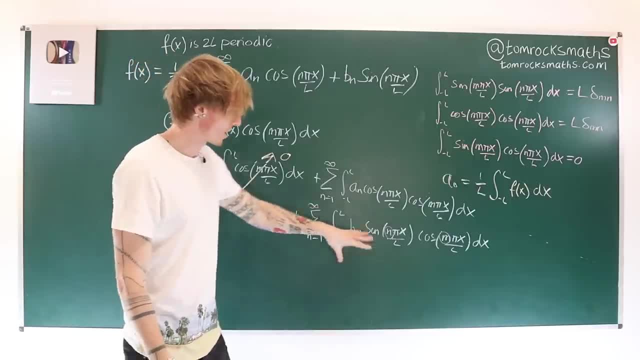 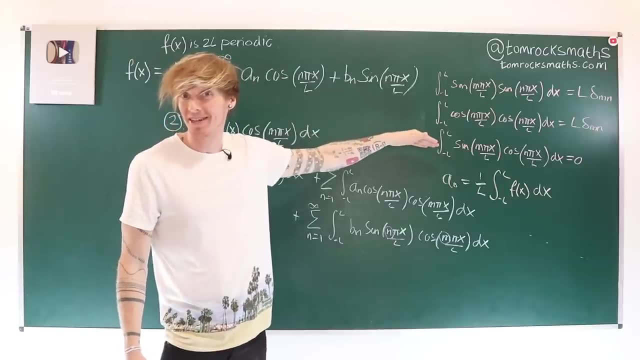 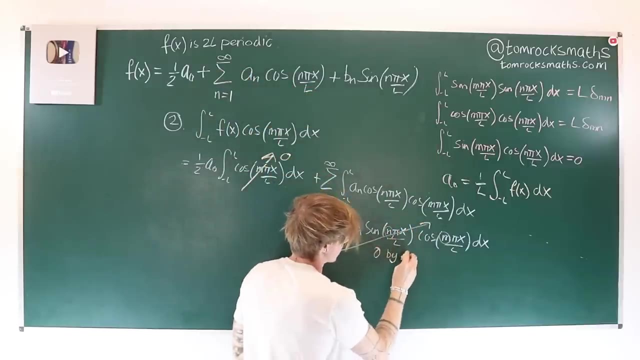 possible values from 1 to infinity. So this covers all possible pairings of sines and causes. but by the orthogonality relation we know this is always zero. So this whole thing, this whole thing here, is zero by orthogonality. 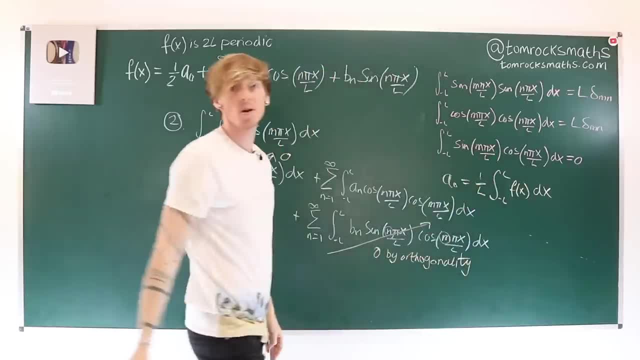 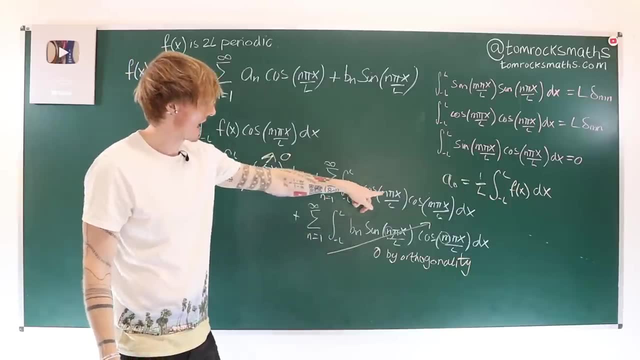 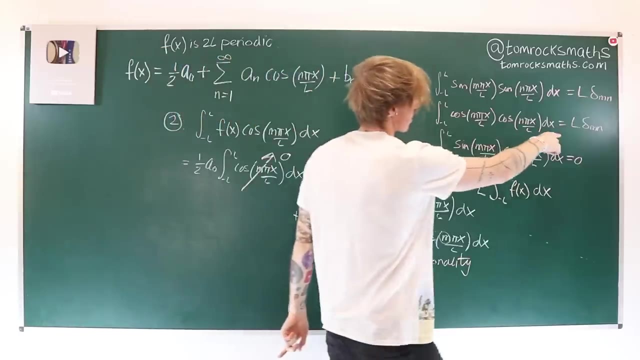 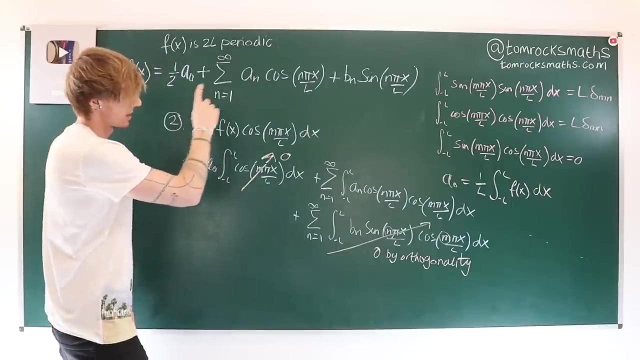 Precisely from this third one up there. So that just leaves this term. Now we've got a cos n pi x over L times, a cos of m pi x over L, and that's exactly what we've got over here. It's L times delta m n. So what we can do is say this: here becomes: we've still got the a n. 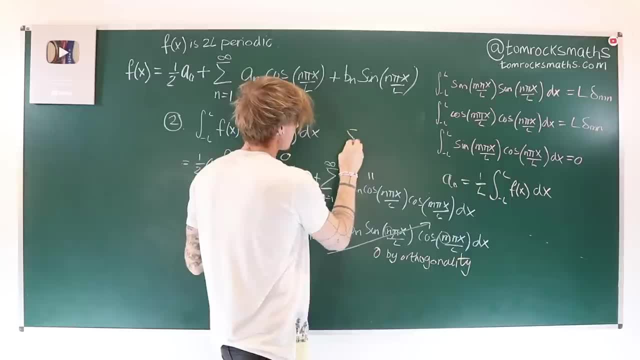 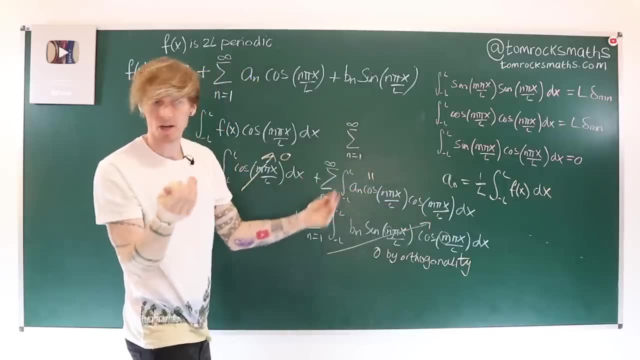 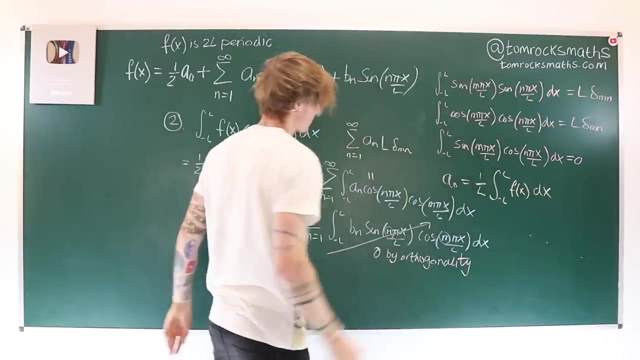 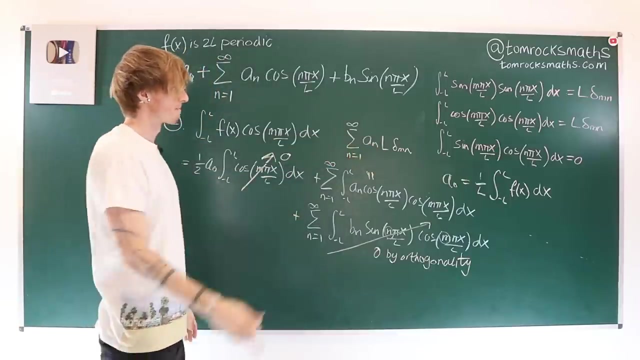 because that can come outside. so we're left with the sum from n equals 1 to infinity and then doing the integral, but taking out the a n because it's constant, we've got a n, L, delta, m, n. Now L is just a constant, so we can just divide by that. that's no big deal. but the n here, a n. 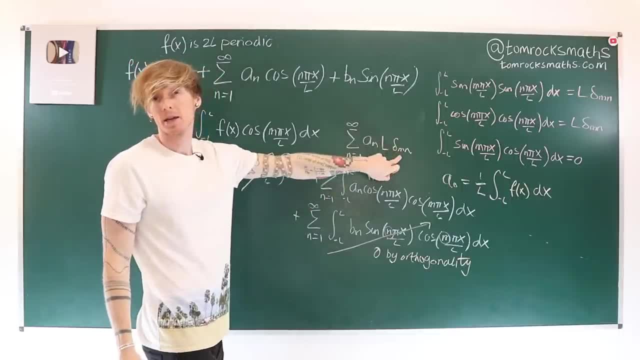 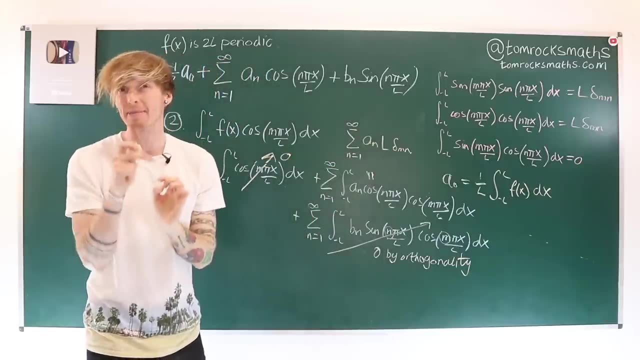 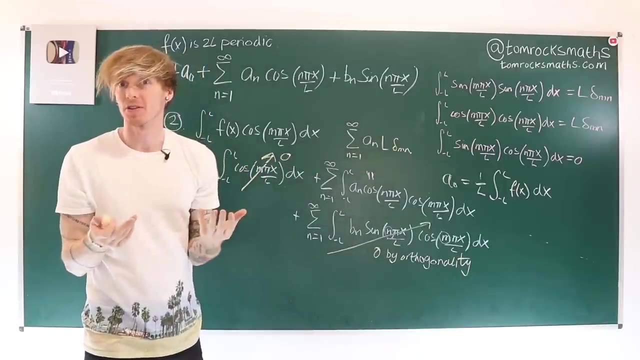 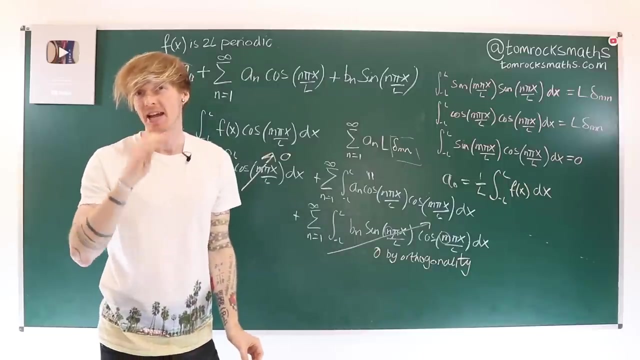 depends on the sum, but it's being multiplied by delta m- n. Now remember, the delta function was one: when m equals n, When they are the same value, it gives you one and it gives you zero when they are different. So what this does is it actually picks out exactly when m and n are the same thing. 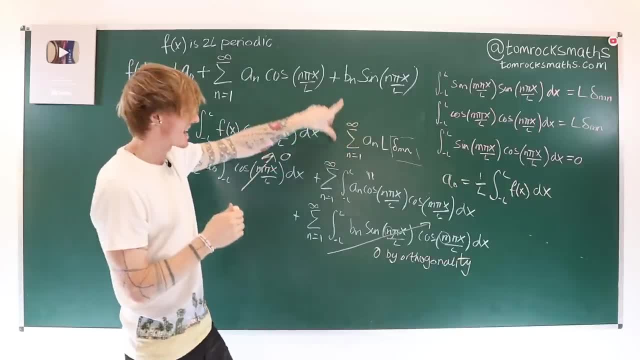 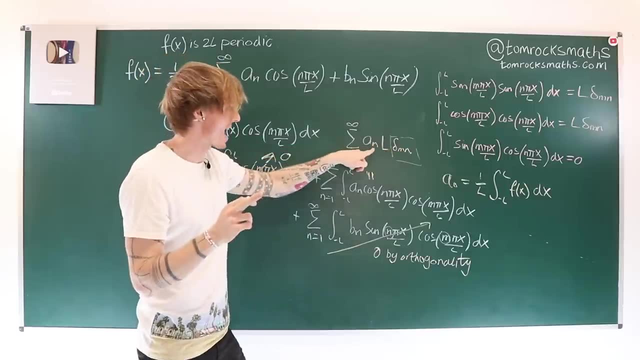 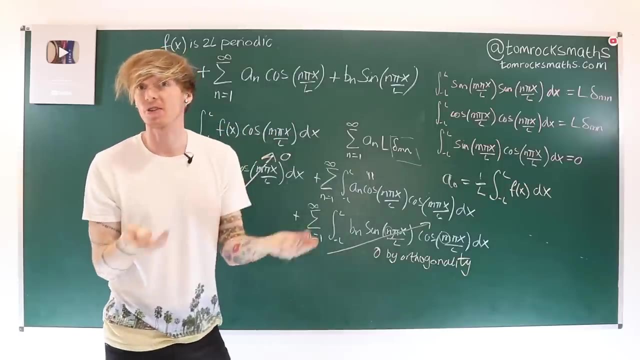 So, even though there are an infinite number of terms in this sum, this ensures that we get a single term, and that single term is when n and m are the same thing. So, whatever value of m I pick, if I pick m is 1,, m is 2,, m is 3,, every time I pick a value of m, 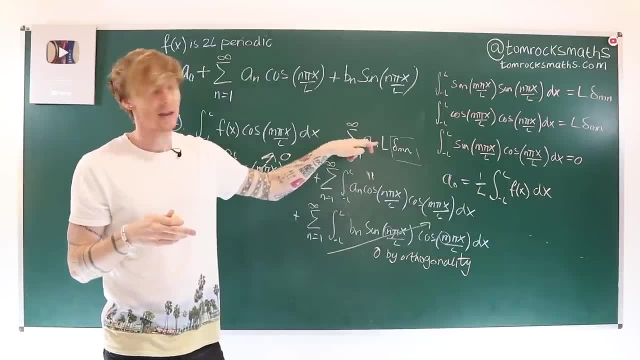 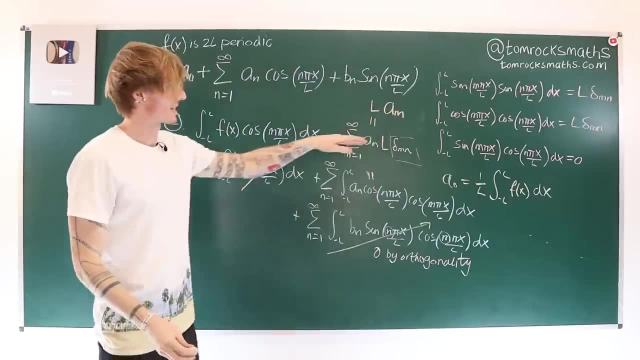 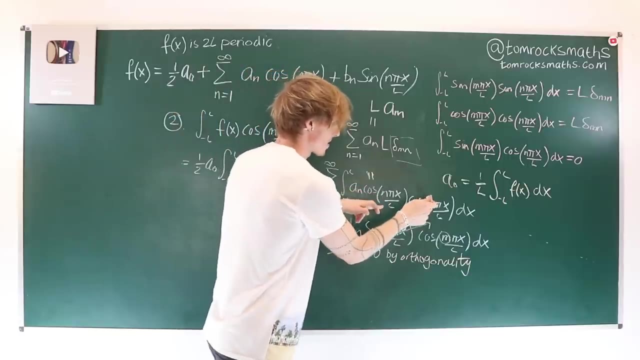 this will pick out exactly that coefficient. So we can actually say this whole thing is just L times a- m, because again, we only get a non-zero answer to this integral when n and m are the same thing. So what this means for our coefficient in our Fourier series. 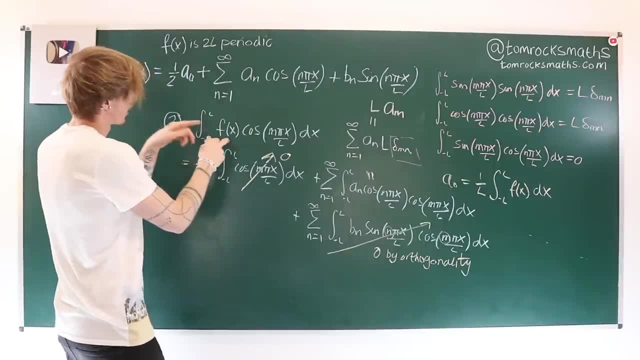 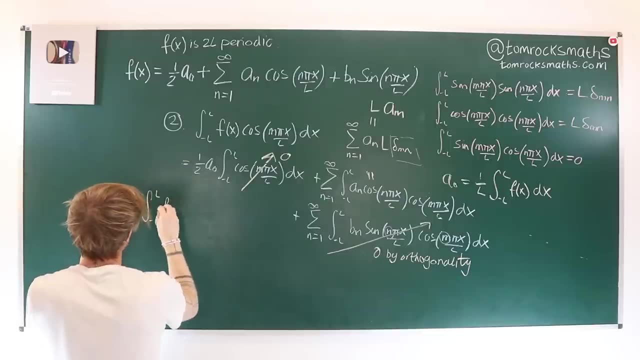 neatening this all up is we're actually left with this expression here. So we've got the integral from minus L to L of f times cos. remember we fixed this cos of m pi x over L dx, That's the left hand side. 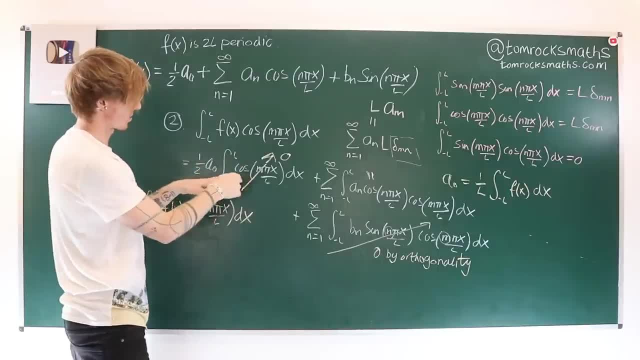 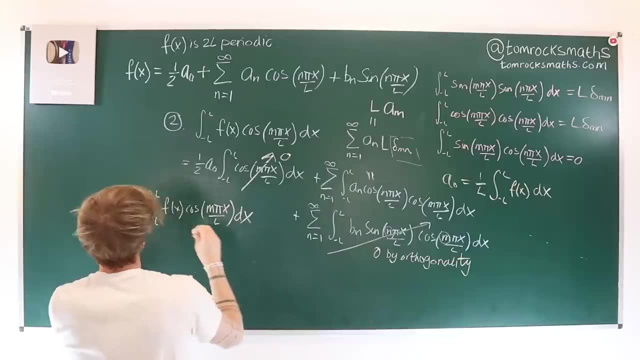 side of our expression, And all we've got on the right was: we've got zero from this, zero from this. l a m, That's it. So this whole thing, we can actually just say: well, if I just put a m here, then this is 1 over l times all of this. So 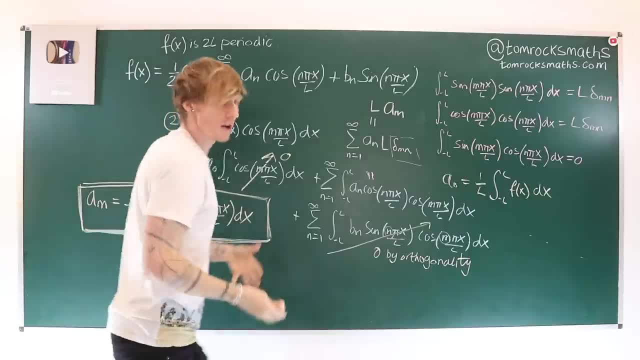 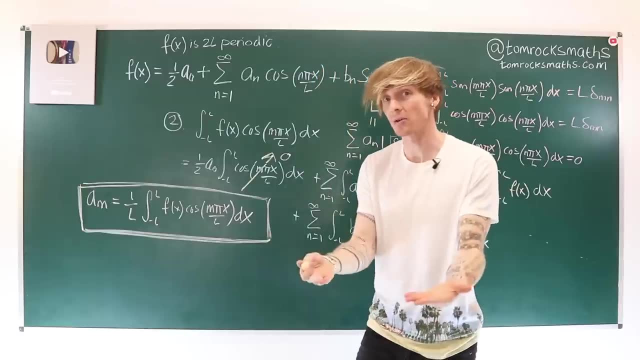 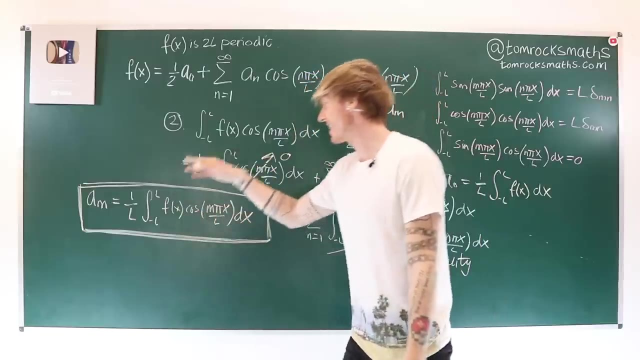 again. you think about it by saying: if I want to know the coefficient a, m, so say I want to know a2,. the way to get a2 is to take my function f, multiply by cos 2, pi x over l, integrate from minus l to l, all of these terms disappear and I get a2.. 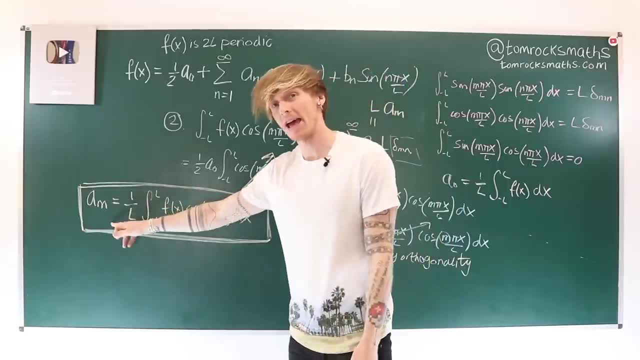 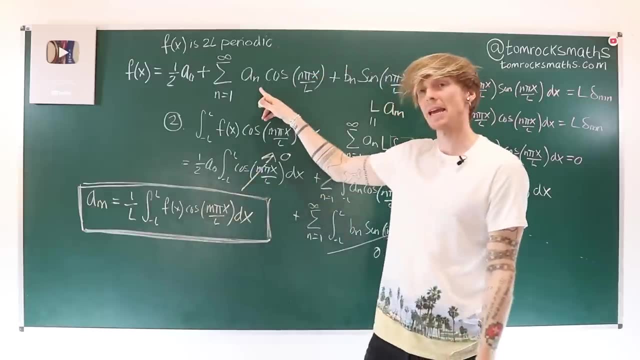 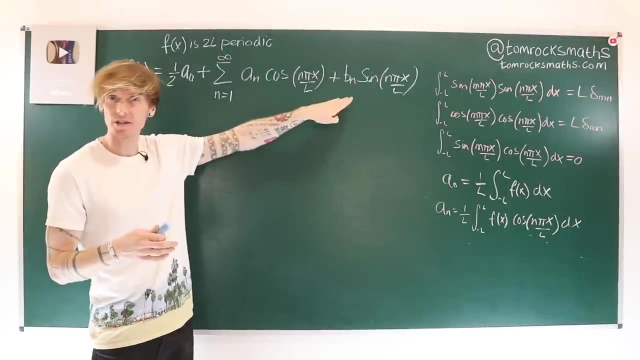 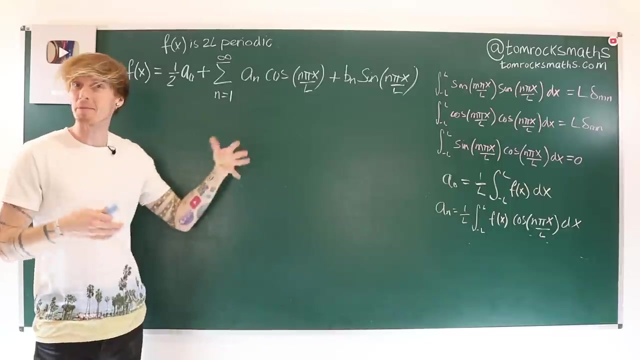 So we can do this for any value of m. so this gives us a way to calculate now every single coefficient that goes up here in our Fourier series. Finally, to get the term b, n, which is the coefficient, the constant coefficient of our sine term, in the infinite Fourier series, we follow the same approach and 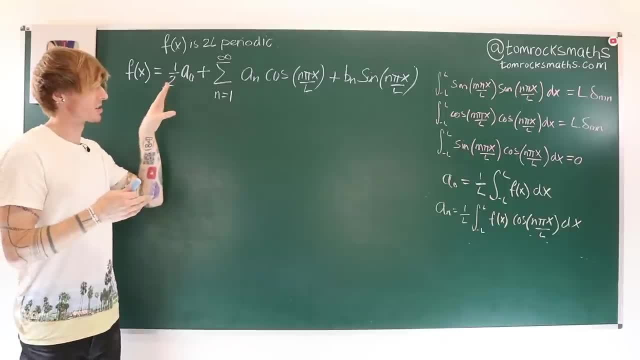 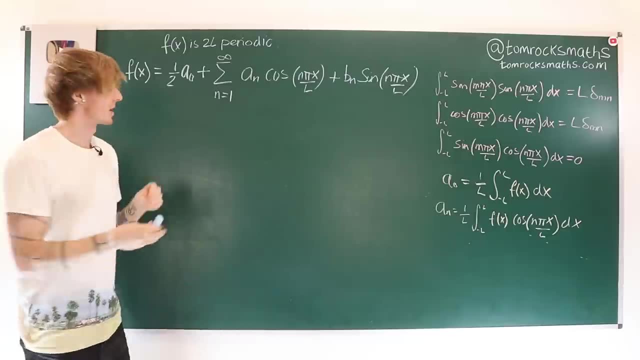 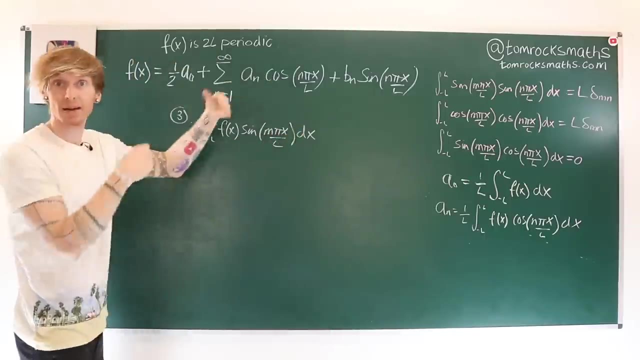 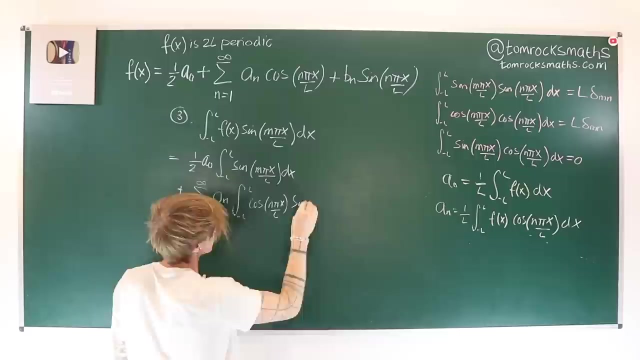 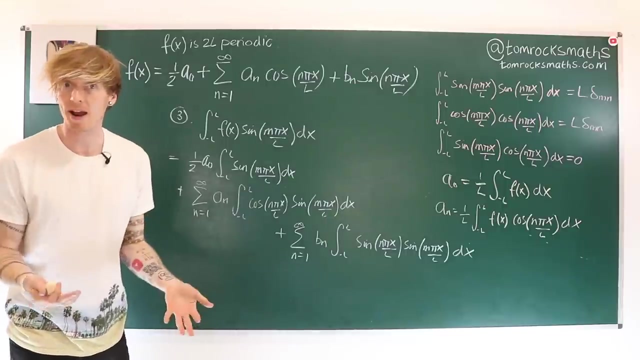 as I'm sure most of you may have realized, we're going to now multiply by sine of m, pi x over l and then integrate. So for our third coefficient we do exactly that, As we've seen a few times before now. this integrates to give me zero, since. 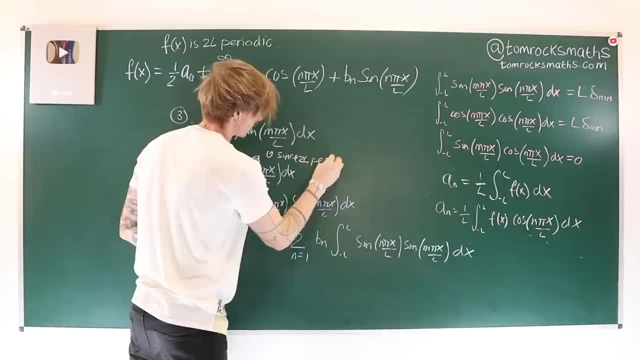 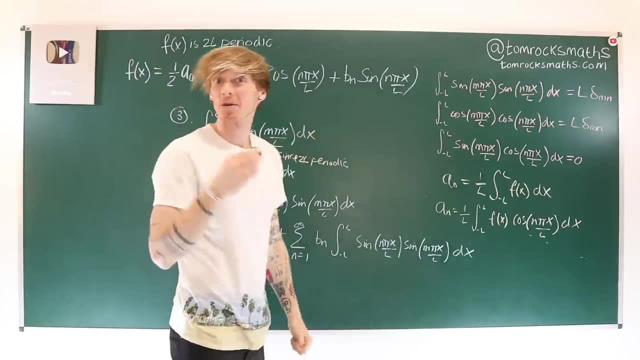 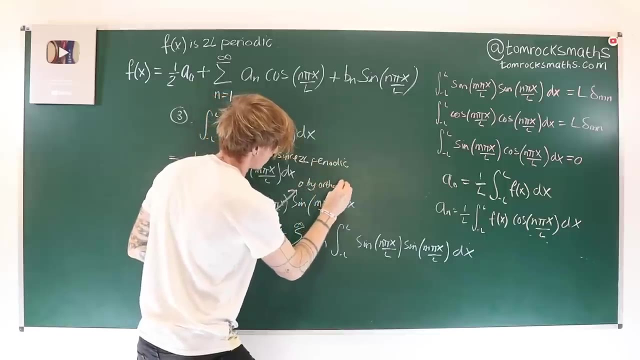 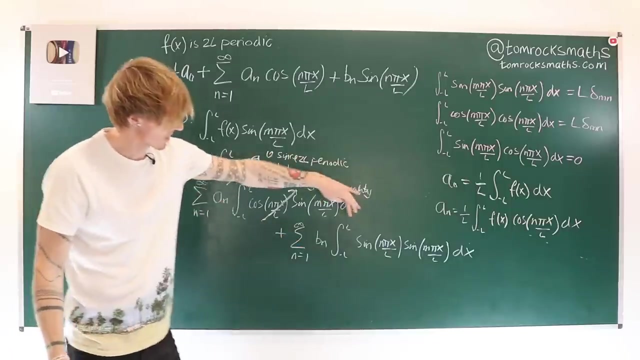 it's 2l periodic and we're integrating over an interval of length, 2l. This term is a cos times a sine. that's zero, always by orthogonality. so this is zero by orthogonality. And then, finally, we have this expression: 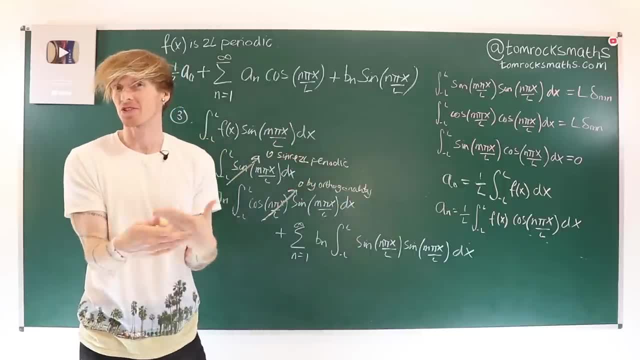 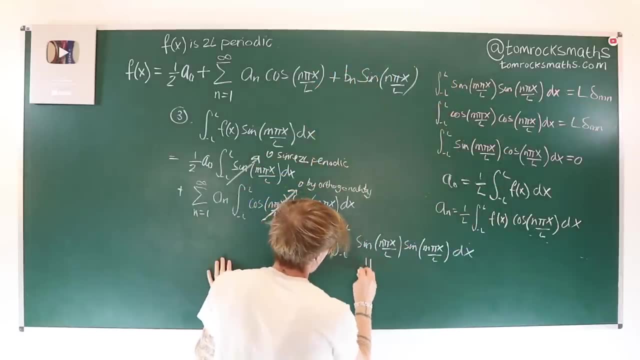 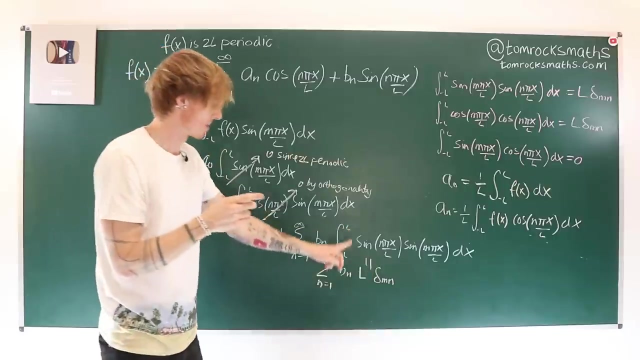 involving the two sine terms, exactly as we just saw with the cos terms. We're going to get this result here. this is equal to l, delta, m, n, and then we've of course got the sum from n equals 1 to l, 1 to infinity of b? n. The delta function picks out exactly the b m. 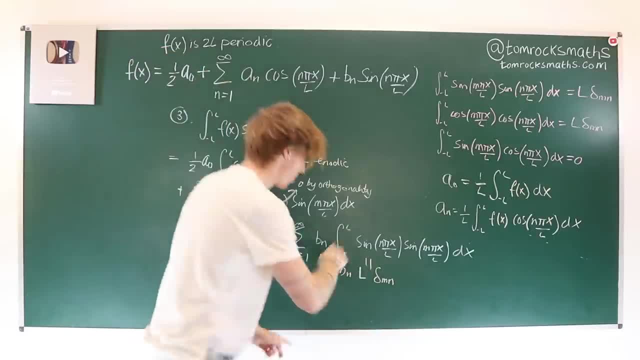 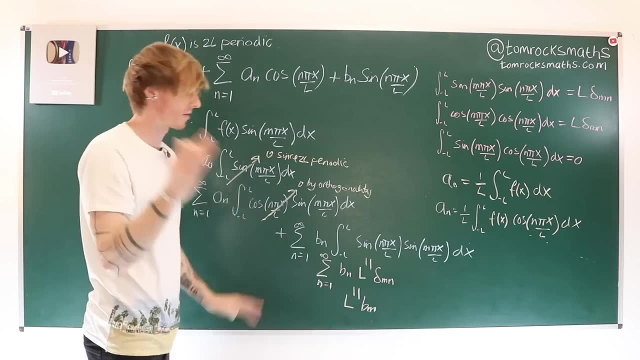 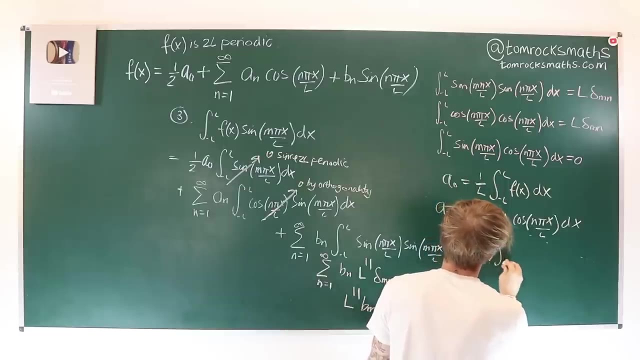 coefficient and absolutely nothing else. so this whole thing together is l times b m. So again we can rearrange and get our final formula. b: n is equal to 1 over l. the integral from minus l to l of fx times sine. 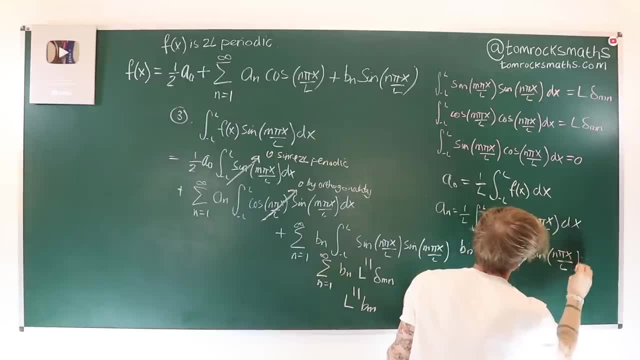 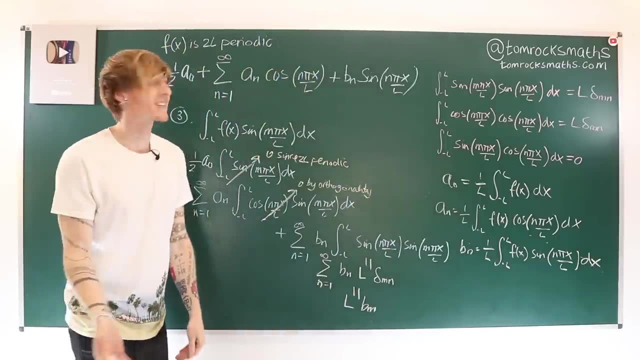 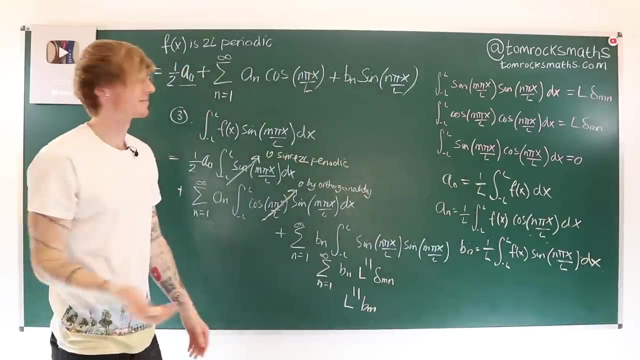 n pi x over l dx. So we have our formula here for all three coefficients, which allows us to determine the constant 1 a 0.. We integrate f between minus l and l For our constant in front of the cos term. we multiply by cos n pi x over l. 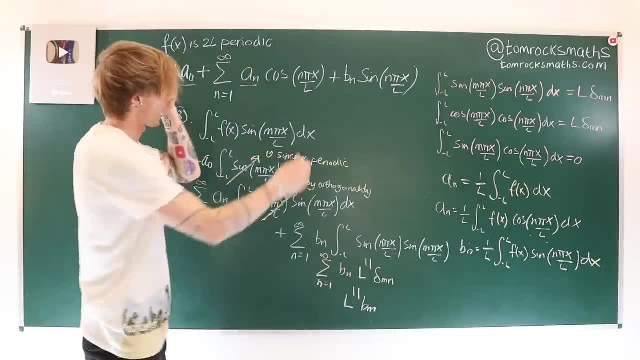 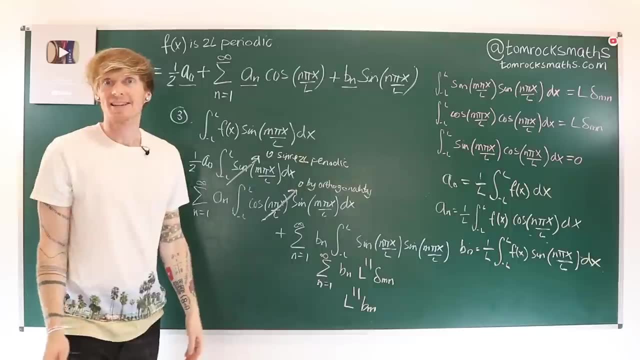 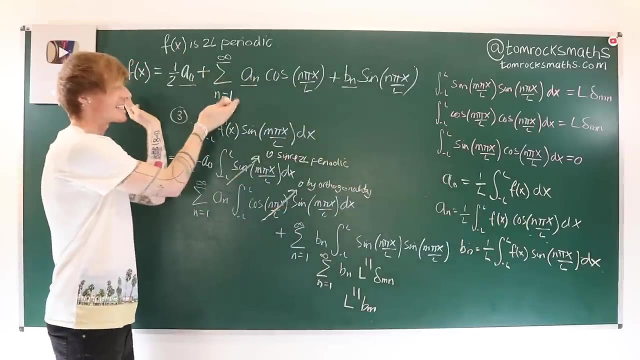 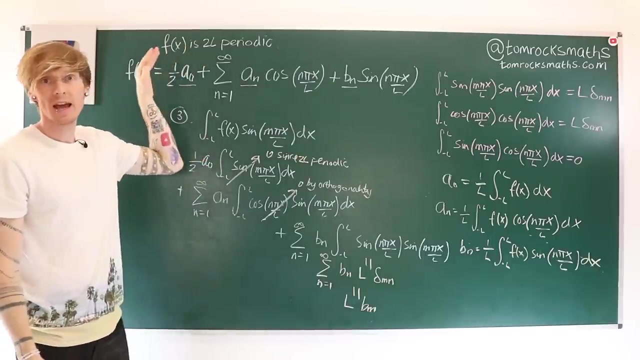 Multiply f by that and then integrate. and for our coefficient, here we got our on the sine term- multiply f by sine and integrate. So this gives us explicit formulae for all of the coefficients, which means we can indeed write down our Fourier series for any 2L periodic function f, The best way to get to grips. 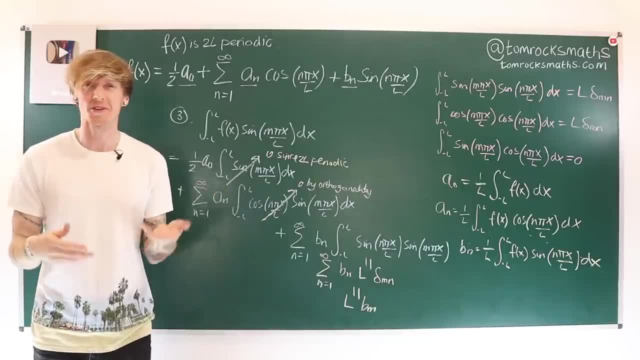 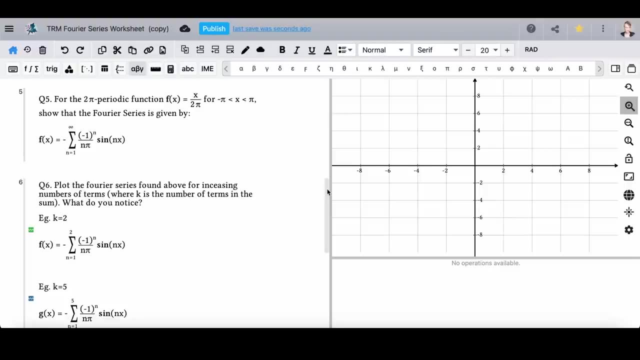 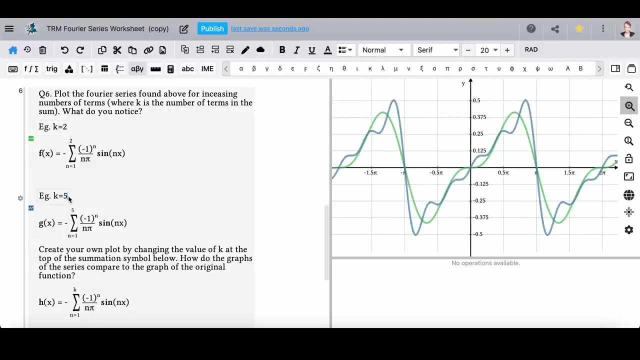 with Fourier series is, of course, to play around with them for yourself, which is exactly what you can do. in the accompanying MapleLearn worksheet, There is a question which takes you through a full derivation of the Fourier coefficients for the sawtooth function and allows you to see how the series 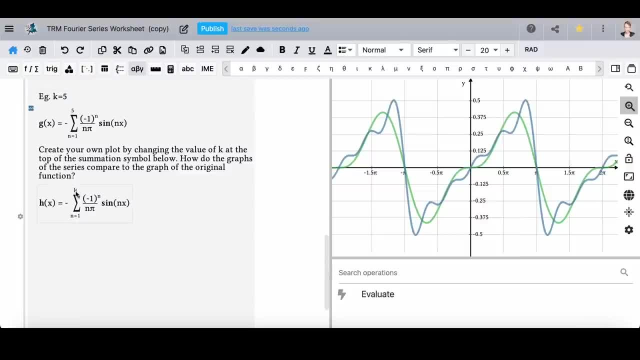 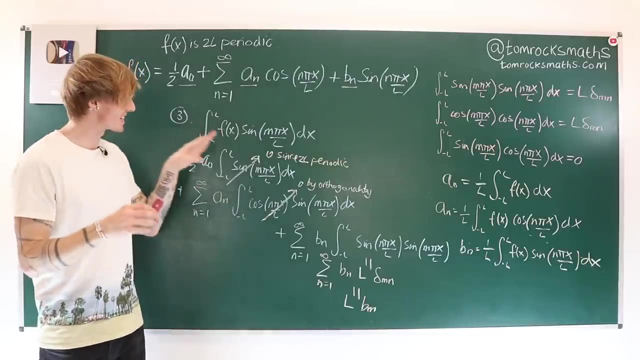 provides a better and better approximation to the graph as you include more terms. As always, the worksheet is linked below and is available for free courtesy of MapleLearn. Now, I did mention that I would briefly address the series in the next video, The issue of interchanging the sum and integration sine, as, of course, our 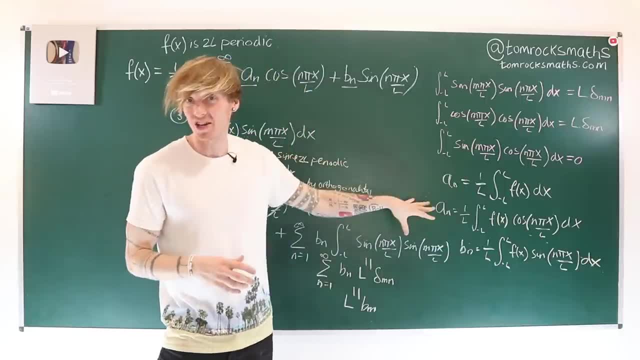 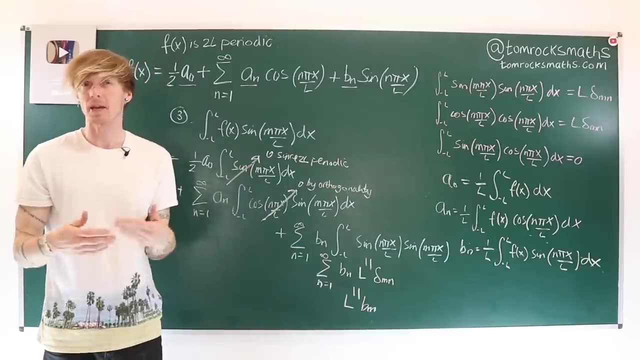 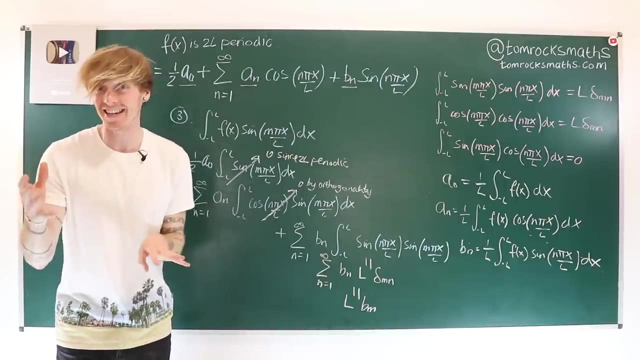 derivation of the formulae for the Fourier coefficients in all three cases did rely on this, interchangeability being okay. I'm not going to go into the full details because that would require a course in analysis and I don't want to go off on that much of a tangent, but the key. 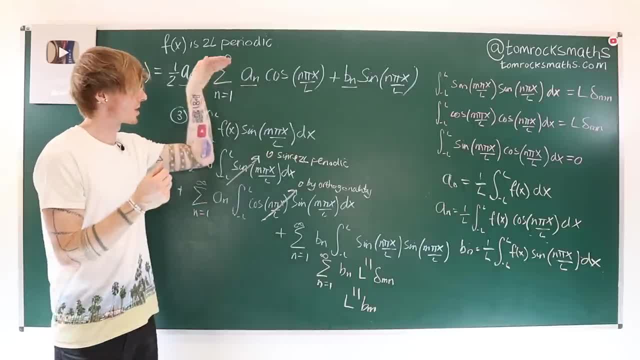 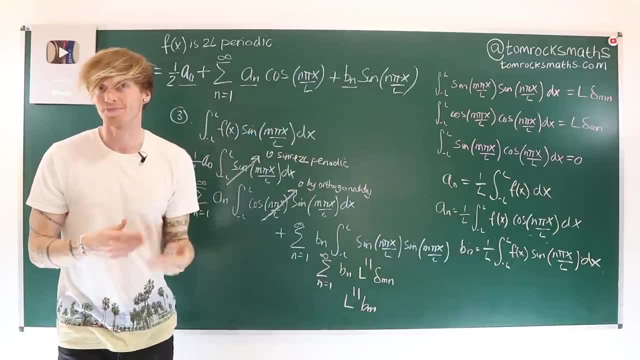 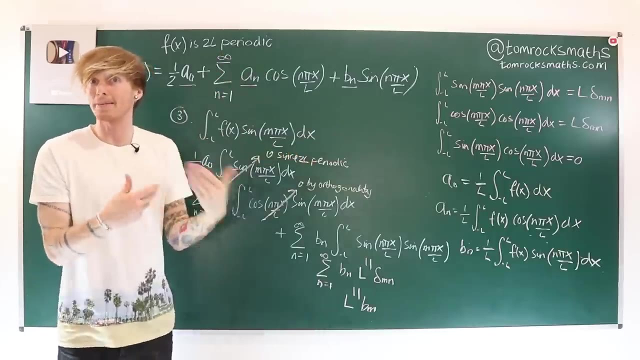 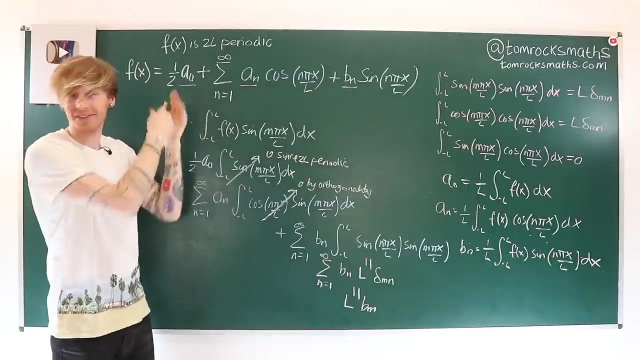 aspect or the key property that we need of our sum for this to be justified, is that the sum is uniformly convergent. Now, what this means in a nutshell is that not only does our sum converge to a limit, which of course has to be finite, it has to converge to something. Here it's clearly converging to f. So not only 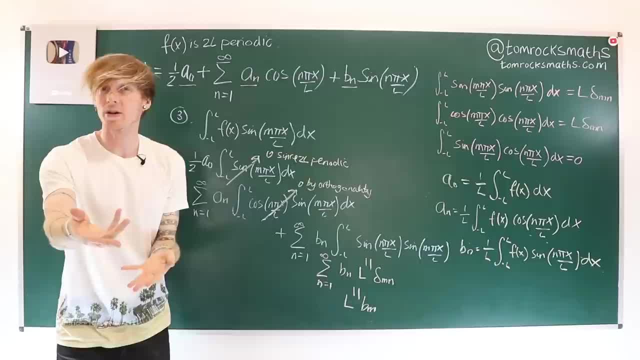 does it have to converge, but if you were to get a sum with a definite of a finite, it would have to have a finite of f. So not only does it have to converge, but if you were to get a finite of f, it would have to have a finite of f. 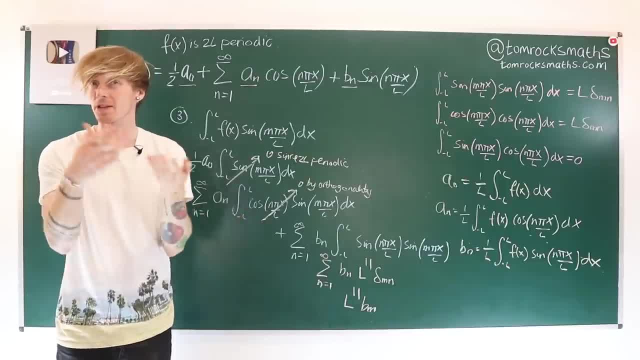 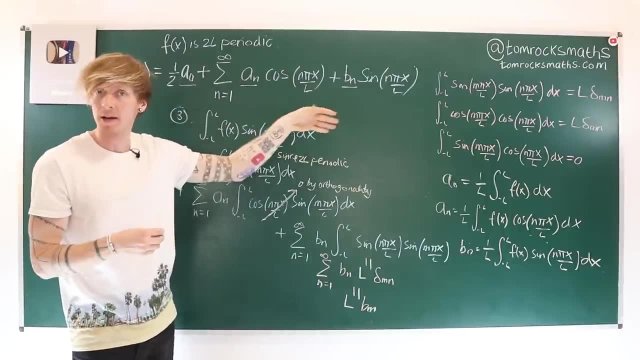 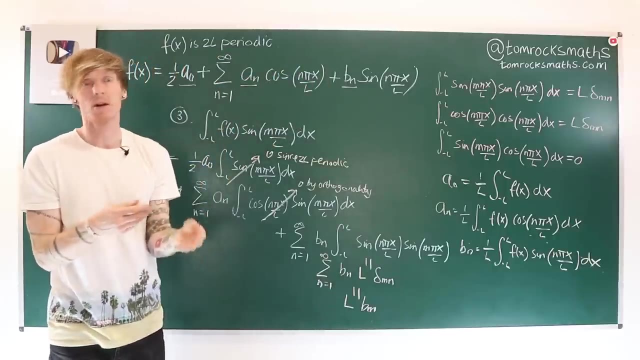 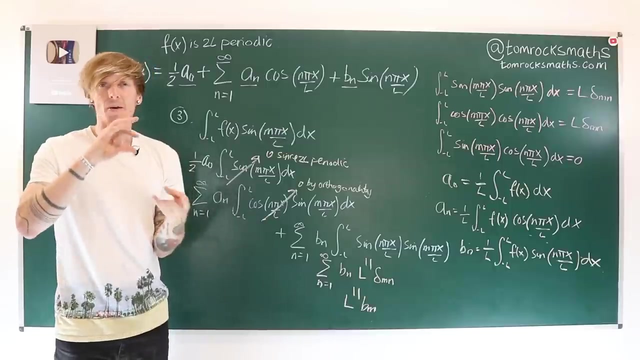 me an epsilon, any epsilon small number that you can think of. my task is to find an n sufficiently far down the sum that I can always add up terms to that value of n and be within epsilon of the final limit. So that just means that the sum converges. Now, if it's going to be,